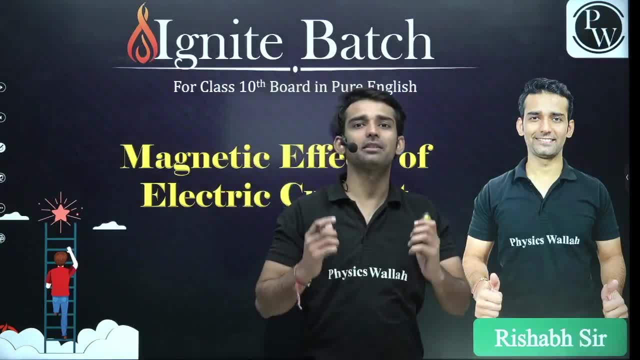 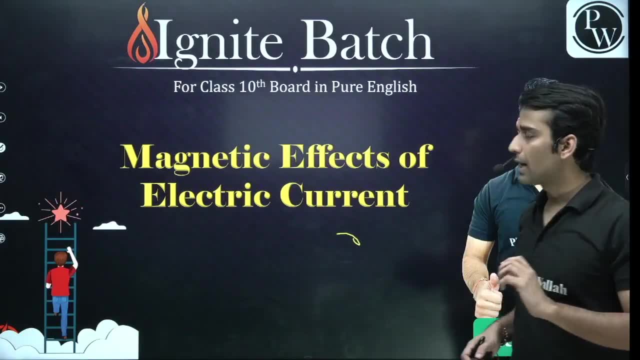 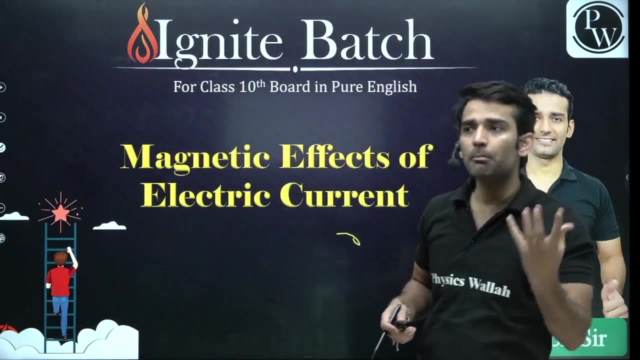 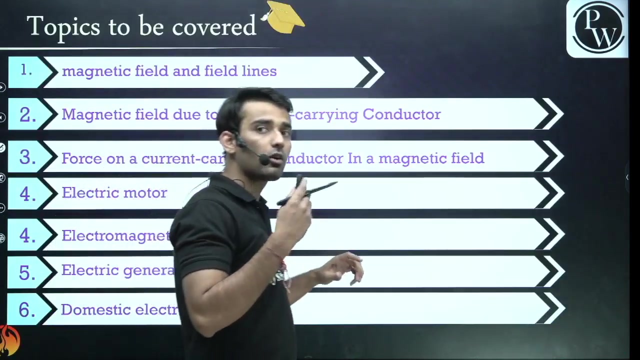 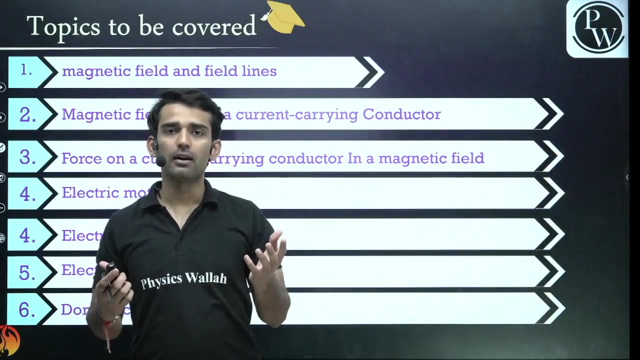 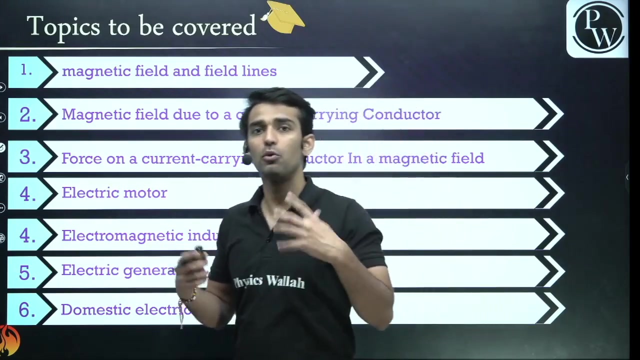 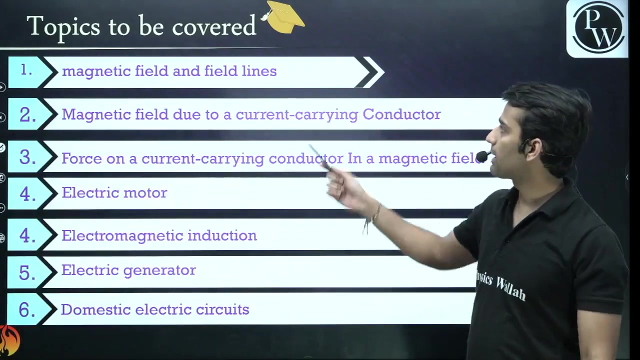 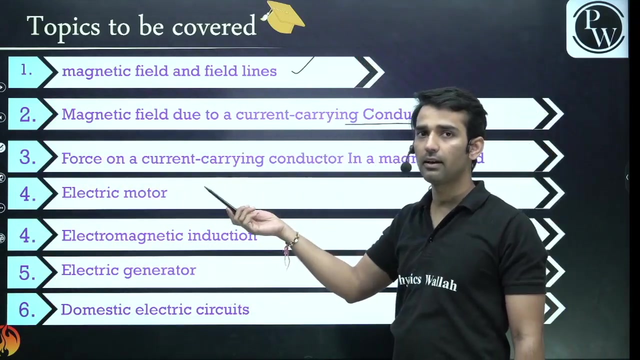 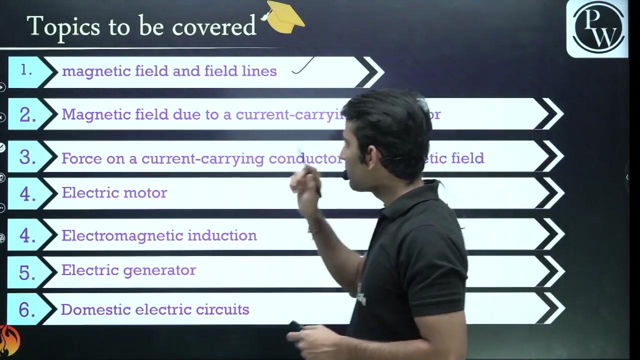 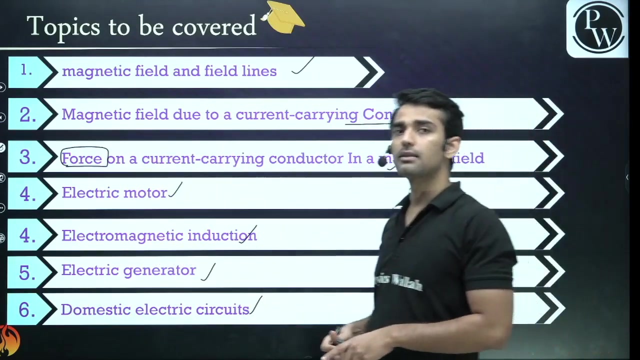 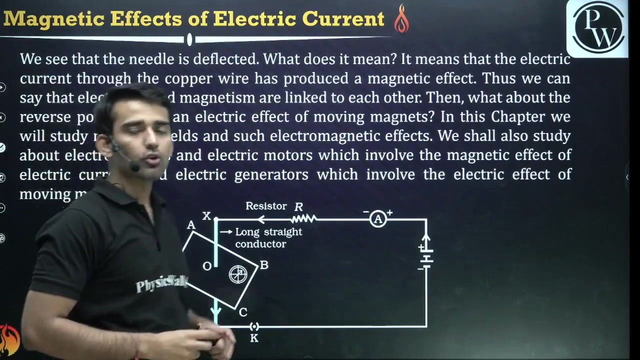 Hey guys, welcome to this amazing platform of PW. My name is Sishyap, your physics teacher and in today's session we are going to start with a new chapter that is magnetic effects of electric current. So guys in this chapter we are going to study about the magnets, about how do current generate the magnetic field around it, how does a compass needle moves when it is put in external magnetic field. Then we will also be studying about the electric motor, electric generator, all these things. So guys this chapter is very very interesting. After human eye, right after electricity, after light, this is one of the most important chapter for your 10th class for your board examination because it covers most of the weightage in your exam. So guys what are the topics that we are going to study in this chapter? First will be magnetic field and field lines. We will study about the magnetic field lines, their properties. Then how does the magnetic field, you know what is the shape of the magnetic field, how the magnetic field due to a current carrying conductor. Current carrying conductor can be straight wire, right can be circular wire. Then we will study how a current carrying conductor experience some force when it is put in magnetic field. At last we will study about electric motor, electromagnetic induction generator and domestic electrical circuit. So guys we are going to discuss these all these topics in brief one by one. So I hope you guys are very very excited about this chapter, right. So without any wasted of time let's start the session now. So guys first of all what are the magnetic effects of electric current, right. So guys Austrid was the physicist what he had observed 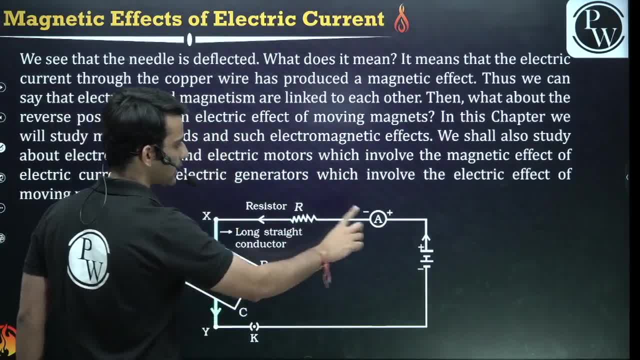 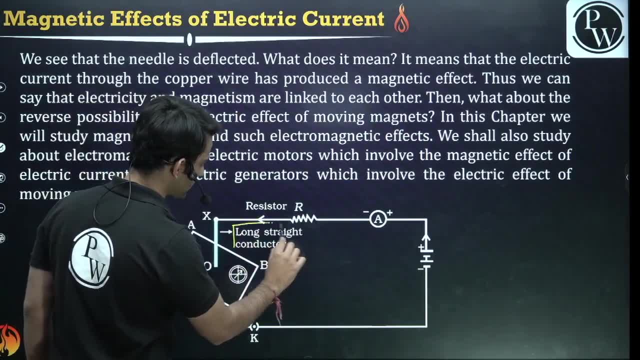 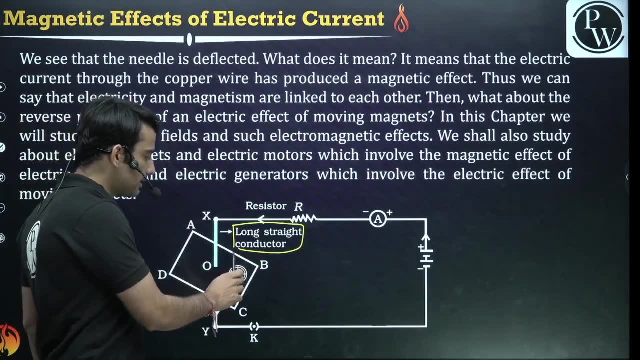 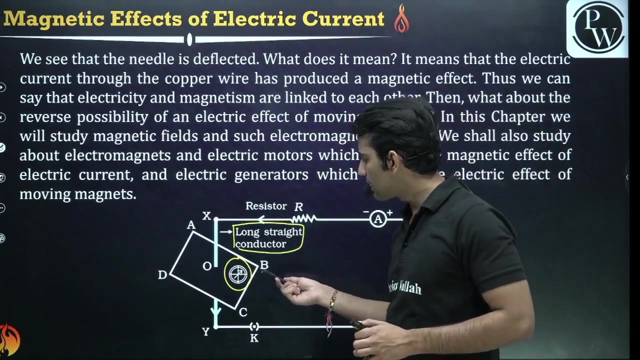 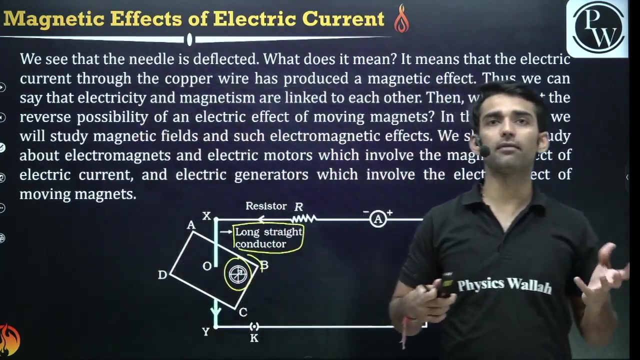 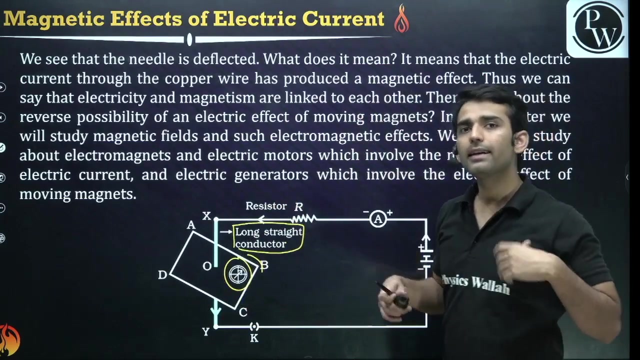 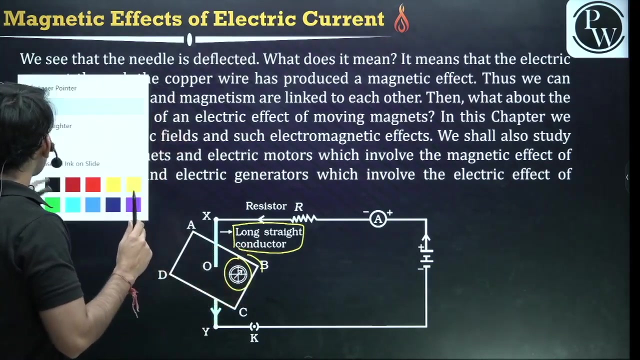 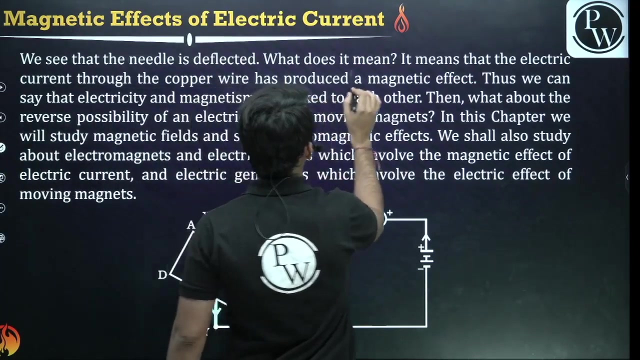 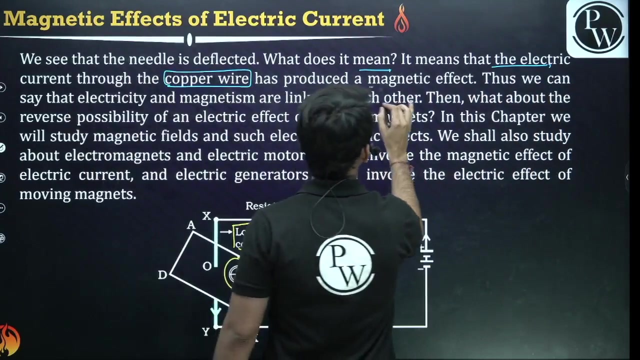 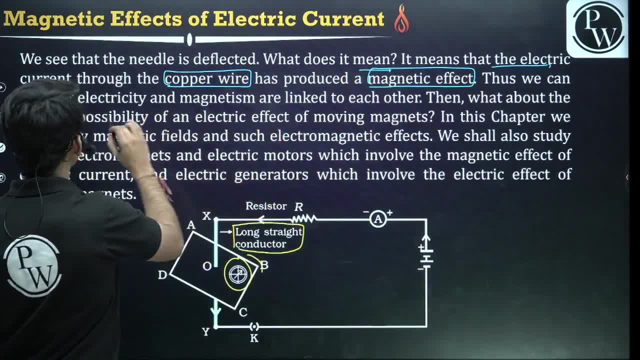 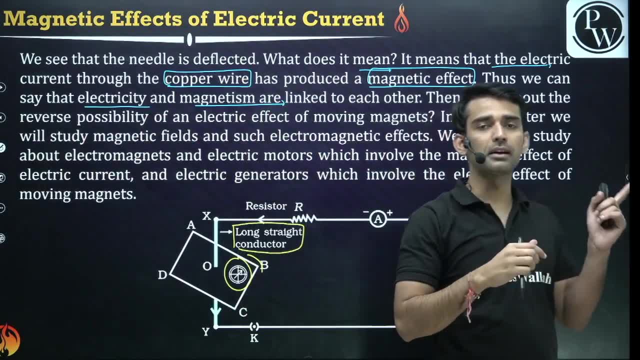 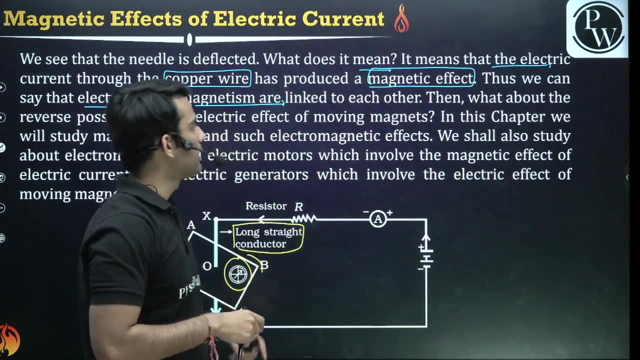 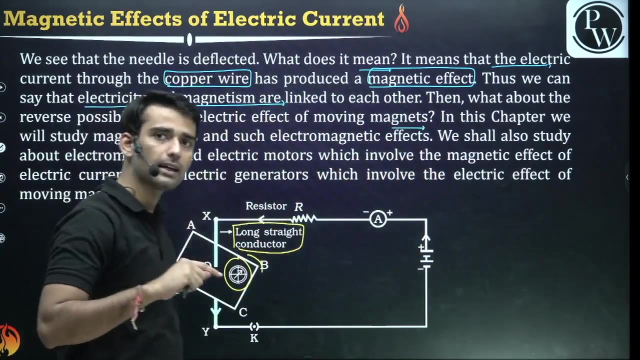 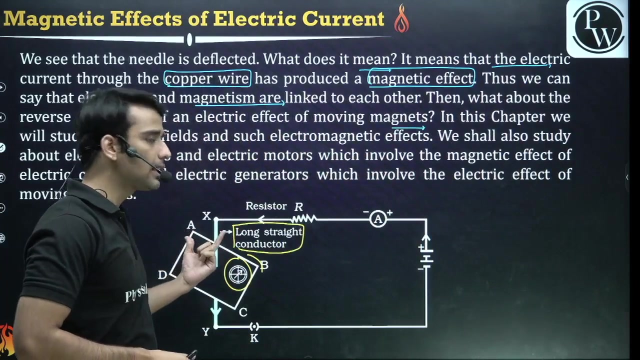 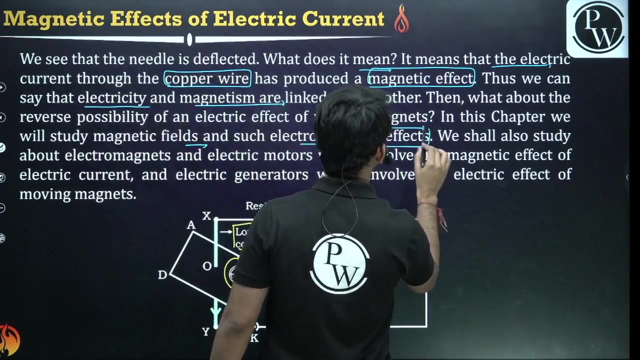 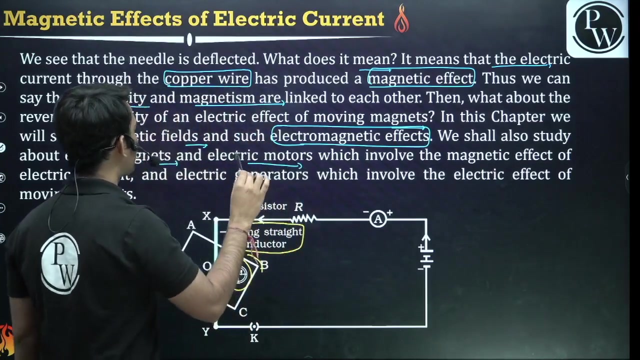 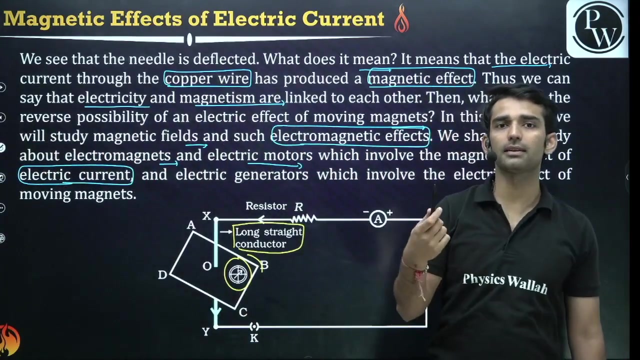 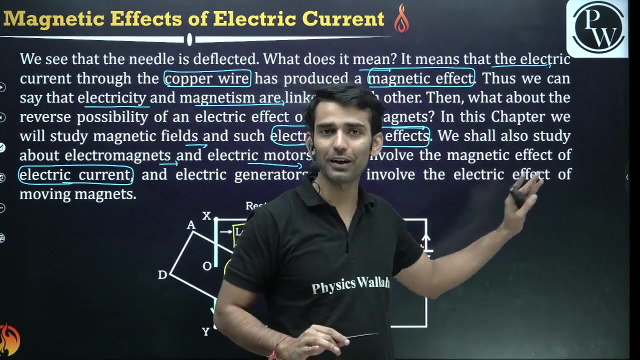 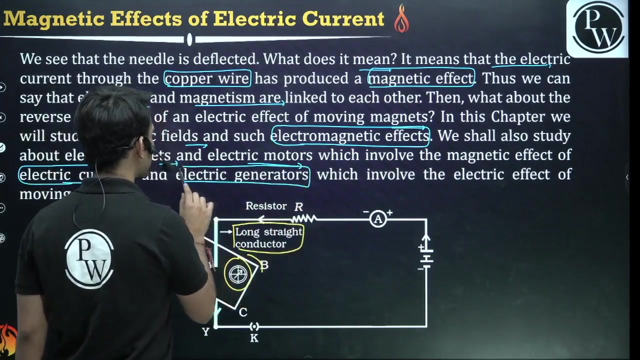 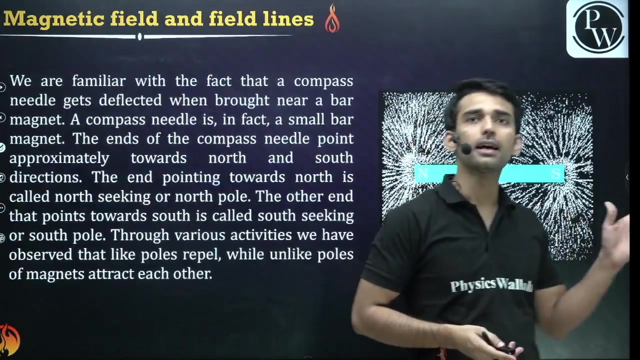 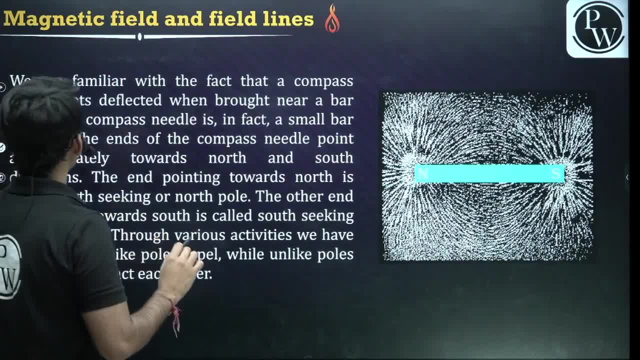 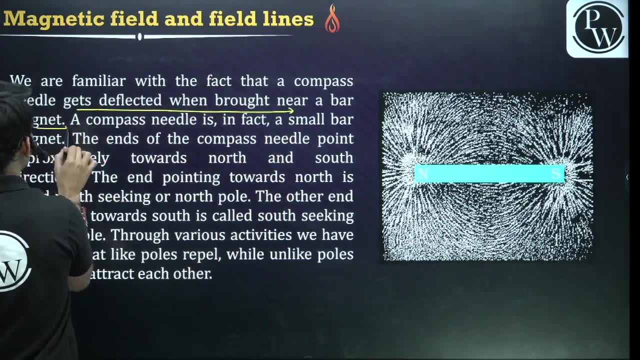 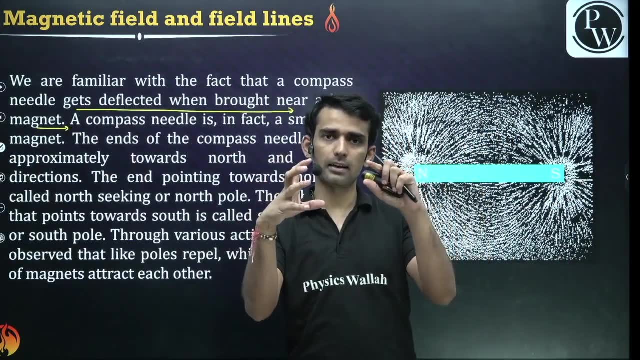 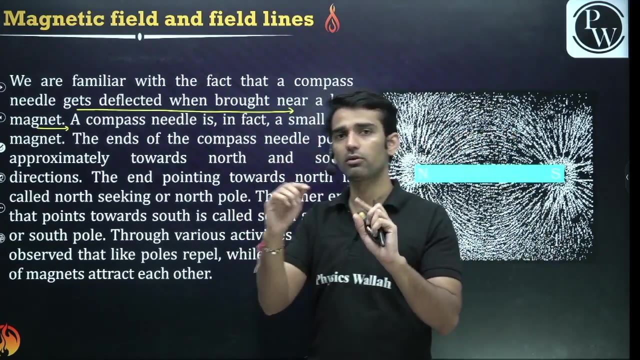 is the shape of the magnetic field as per the austrade so we are familiar with the fact that compass needle gets deflected when brought near a bar magnet we had seen because a bar magnet has its magnetic field so when compass needle is brought compass needle is nothing but iron needle right so when you bring the iron needle a compass needle or near a bar magnet the needle will show some deflection north north will repel north south will attract so that deflection right so basically 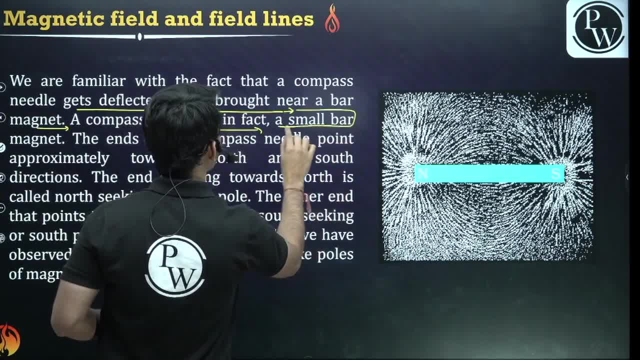 the compass needle is in fact a small bar magnet what is compass needle guys it is a small bar 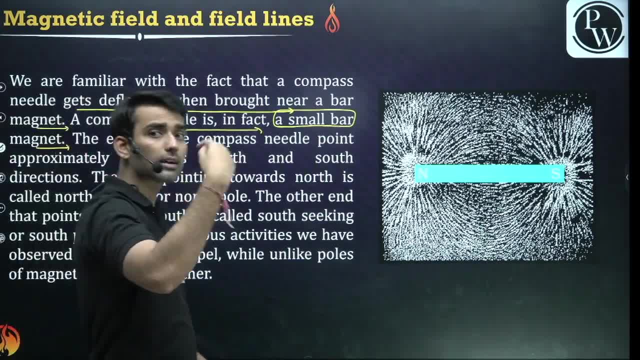 magnet so when you place this bar magnet in any external magnetic field obviously it will experience some force right 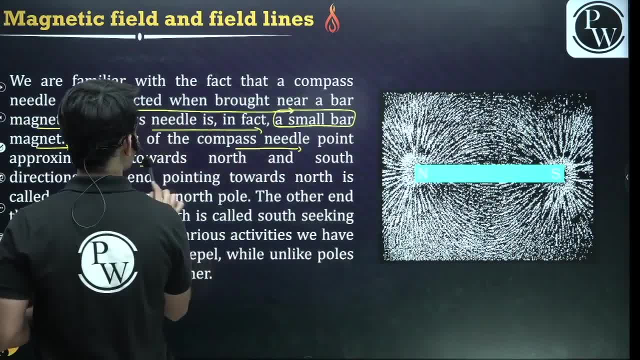 so ends of the compass needle point approximately towards south and the south north and the south 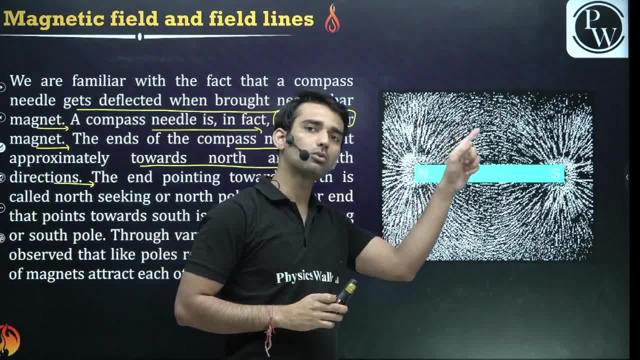 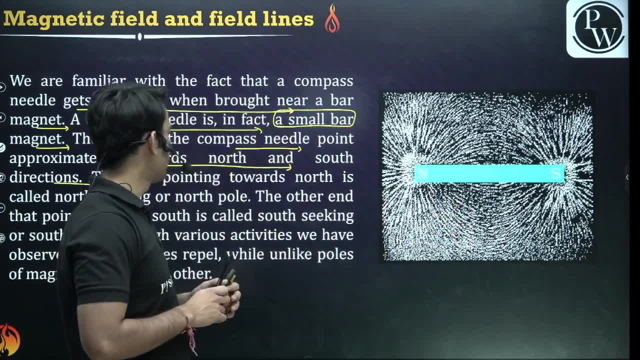 direction right the north of the south will be towards the south of the magnet and the south of the compass needle will be towards the north of the magnet because opposite poles attract right 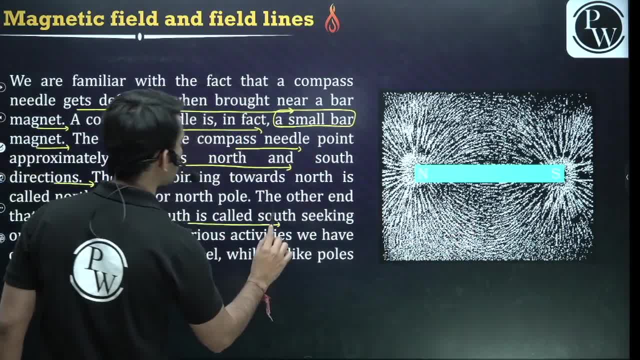 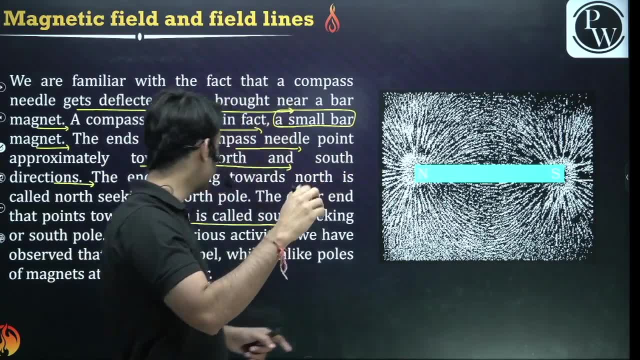 guys the other end that points towards south is called south seeking the point that is point the the pole of the magnet that is pointing towards south it's south seeking right and vice versa 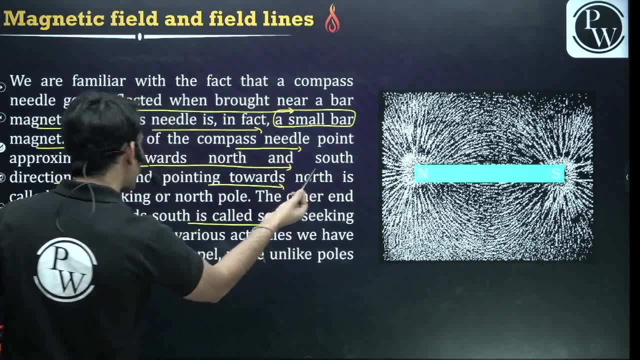 and the point that pointed and the and which is pointing towards north it's not seeking or north pole 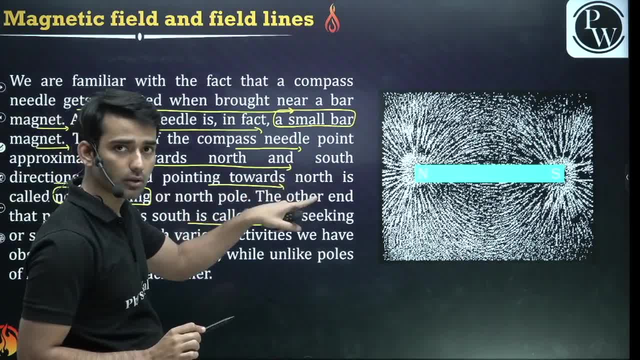 right the and which is pointing towards north which is pointing towards north it's not seeking or north 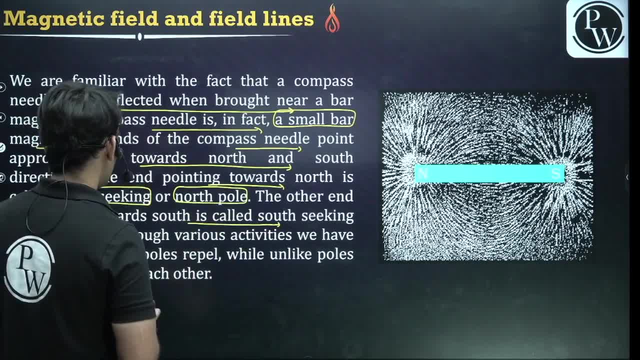 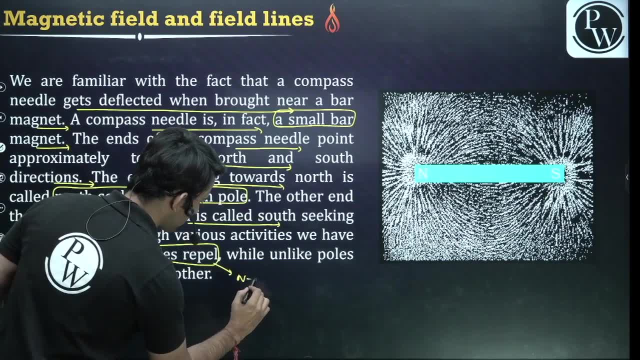 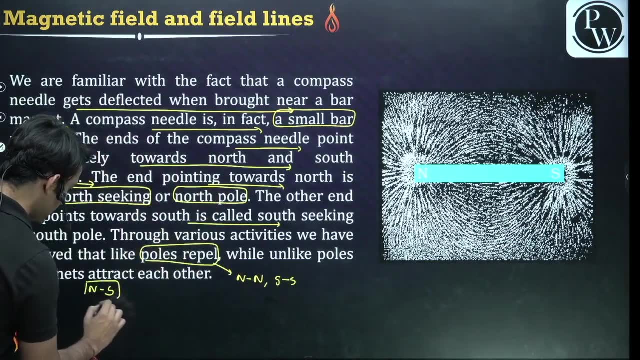 pole we call it north pole right guys so we have seen a various activities that like poles repel if you take a for example north and north pole will repel south and south will repel but if you take unlike poles like north and south so they will obviously attract each other right attract 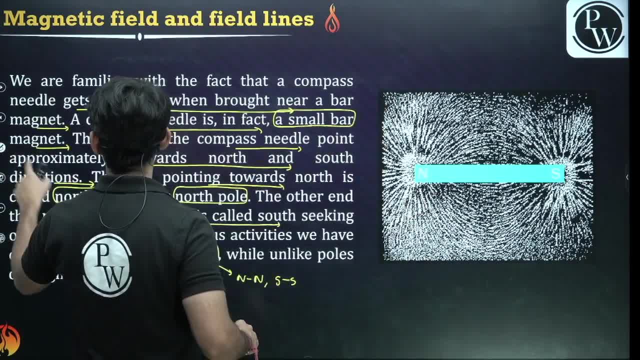 each other so this is the pattern of the magnetic field line what you have done you have taken a bar magnet right you have taken a bar magnet and you have sprinkled iron fillings this is nothing but 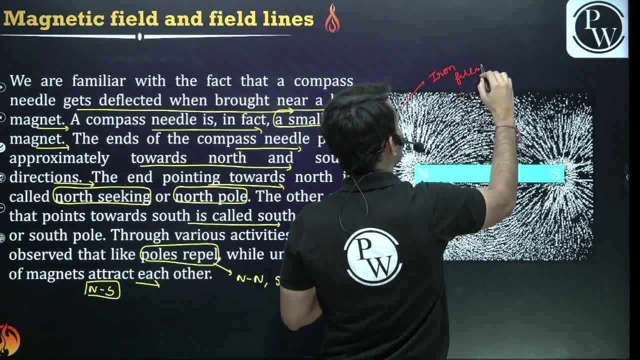 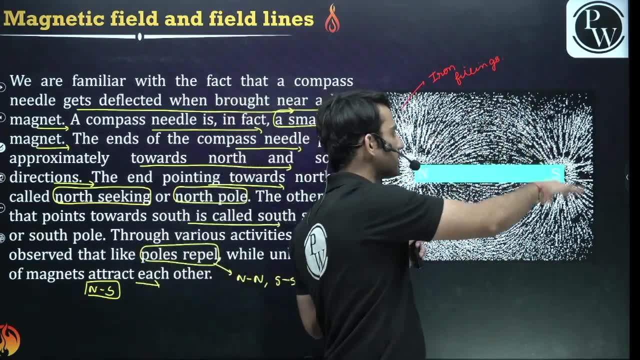 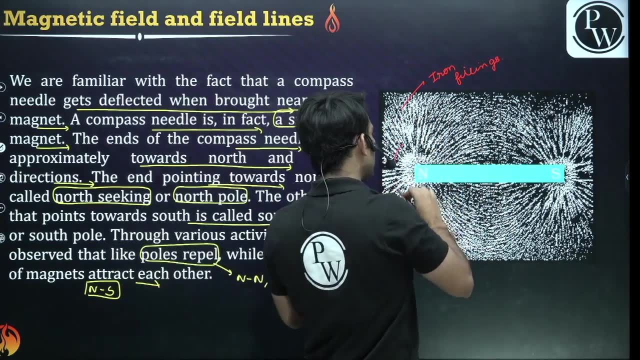 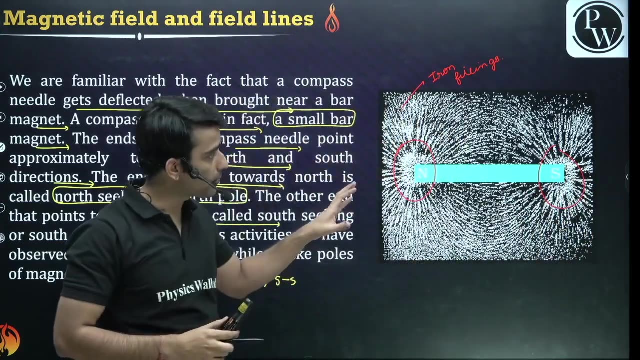 iron fillings iron fillings so after some time you have or you had observed that the pattern kind of looks like this because these iron fillings arrange themselves in the pattern of the magnetic field so you can see they are crowded near the poles right and kind of shape is like this the shape is like this so this is nothing but the shape of the magnetic field around this bar 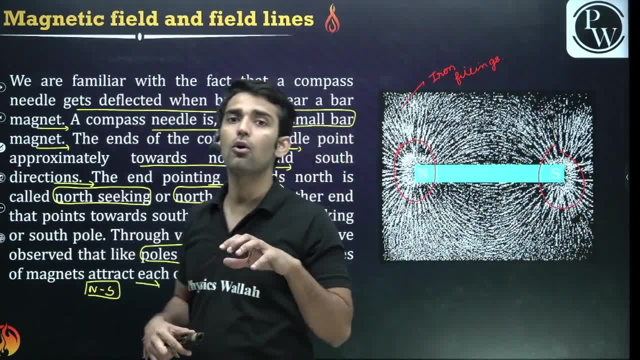 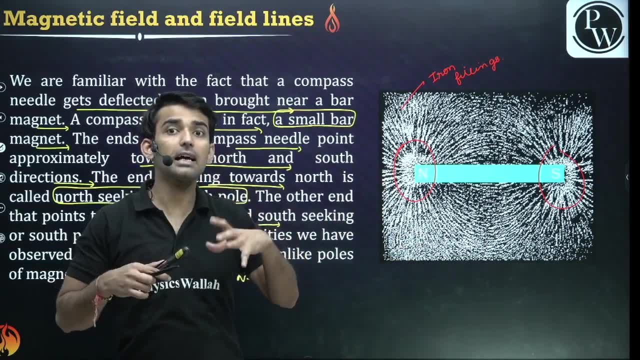 magnet so that's how we came to the conclusion that how how does a magnetic field around any bar magnet look like by this experiment the way the iron fillings arrange themselves clear okay 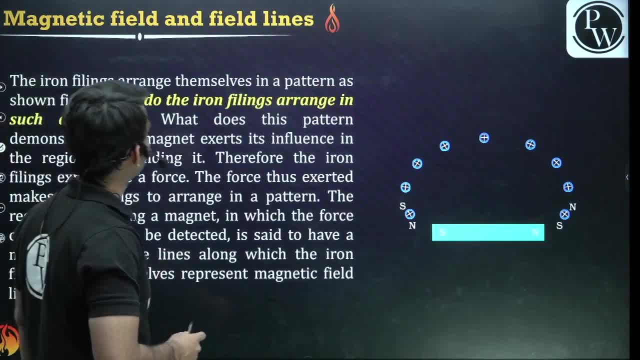 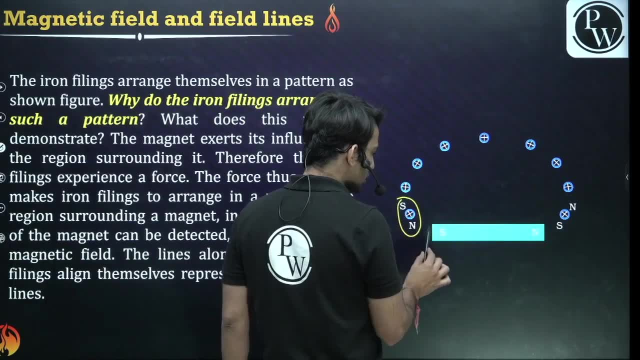 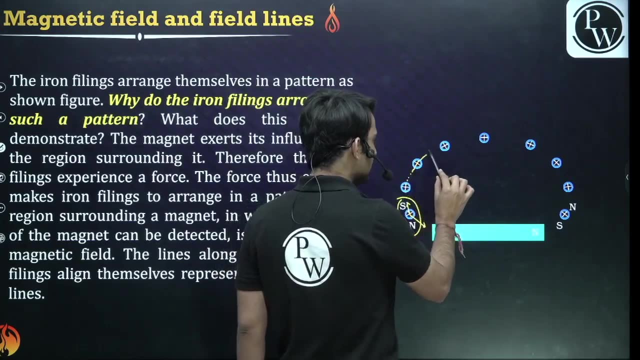 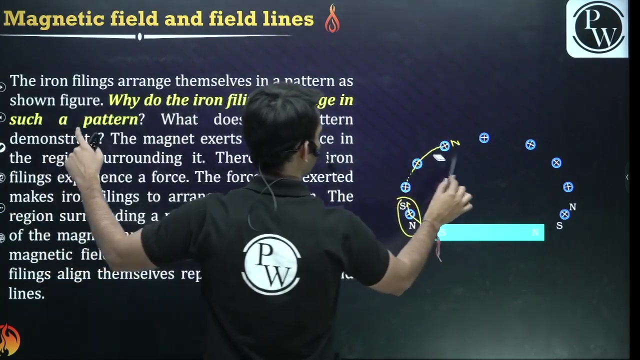 guys so how can we conclude that basically magnetic field and field lines see you have taken a bar magnet north is this south is this you have brought a compass needle here so guys here north will be pointing here and south of the compass will be pointing away so you you keep on moving it like this so you can see this is north this is south right okay sorry this will be basically as soon as you keep on moving this will be what guys 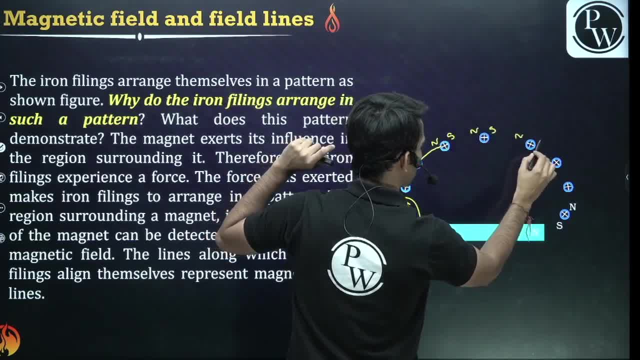 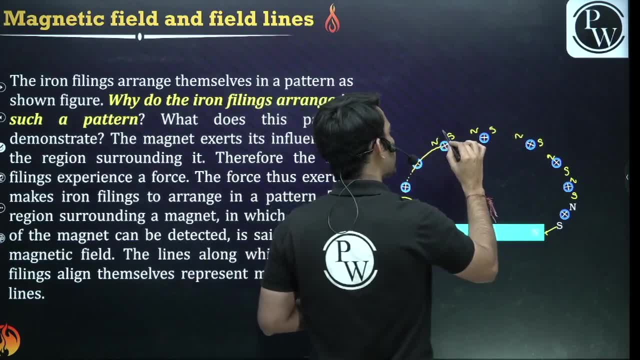 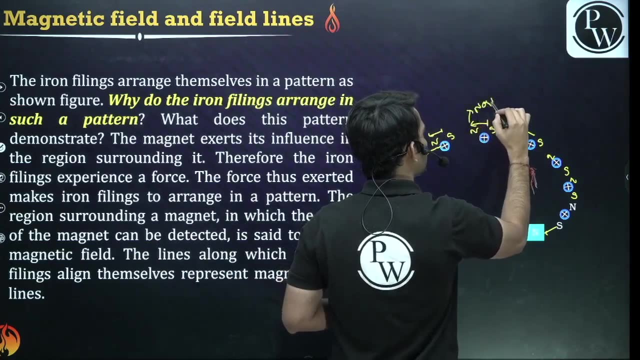 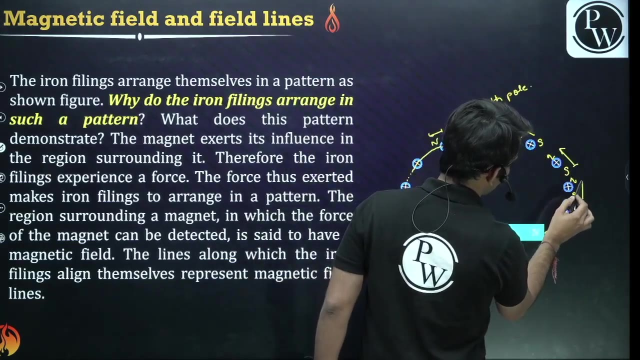 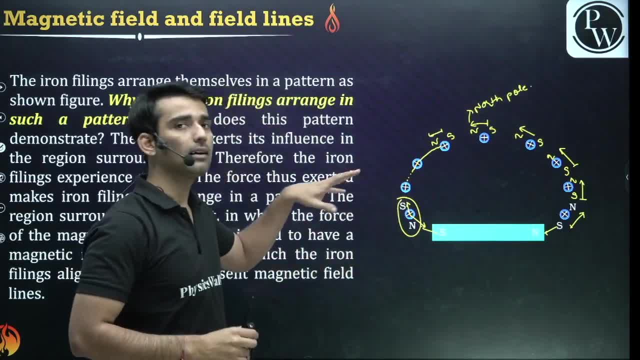 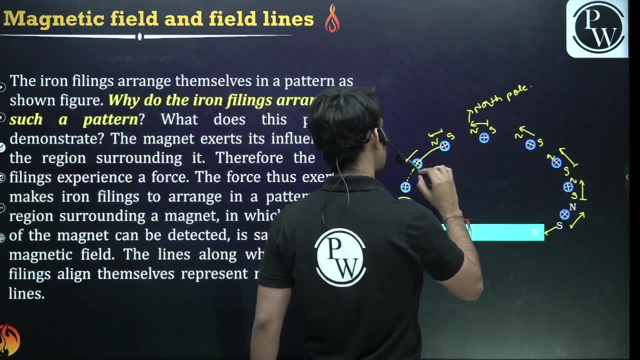 the pattern of the see basically the compass needle align itself in the direction of the magnetic field basically the compass needle aligns itself in the direction of the magnetic field 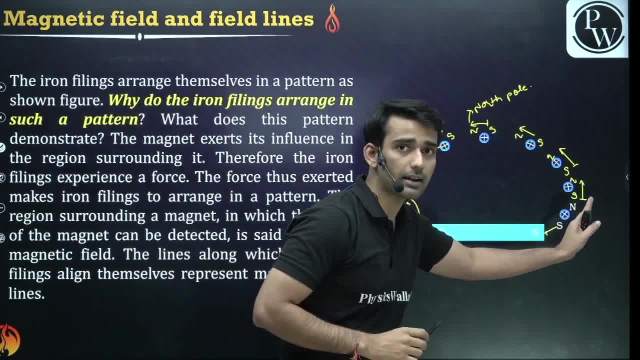 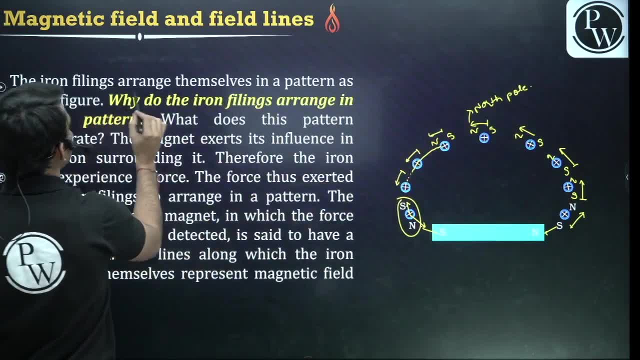 right so that's why you can see it is the direction in which it is aligning if we if we join that we will get the pattern of the magnetic field right guys so iron fillings unease themselves in a pattern as shown in the figure so question is how why do they unease themselves like this 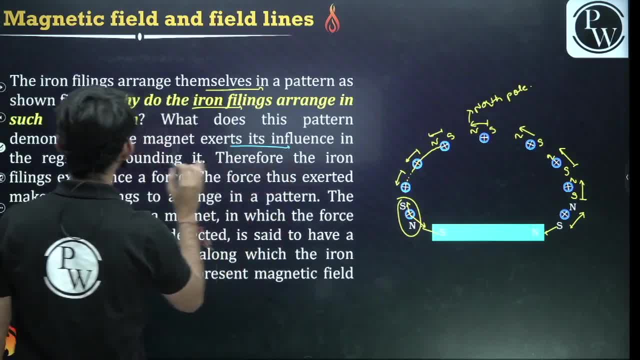 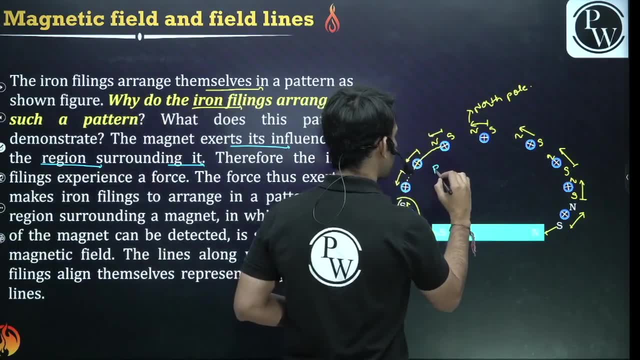 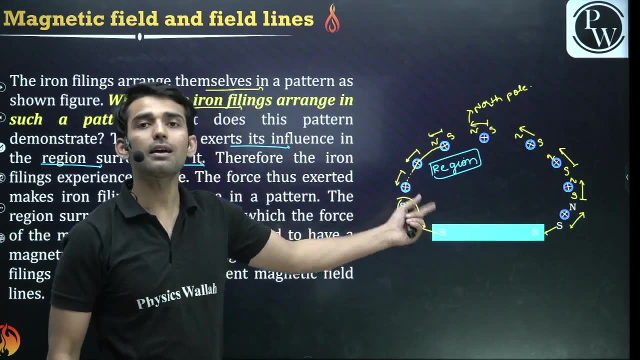 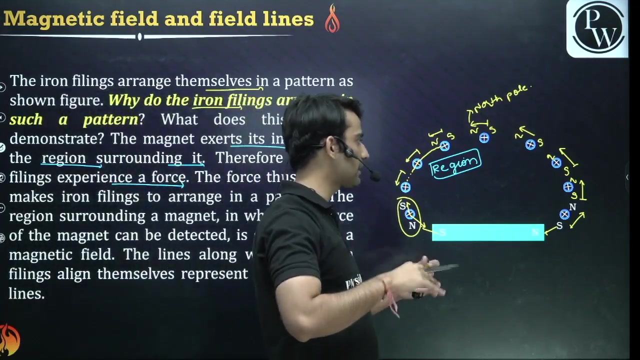 the answer would be basically the magnetic field exerts its influence in the region surrounding it it's a basically every around every bar magnet we have a region this is nothing but the region in which this compass needle can experience some force this is the region so this region is called magnetic field okay so therefore the iron fillings experience some force and if you place any iron fill iron material in this magnetic field or any other magnet it will experience some force 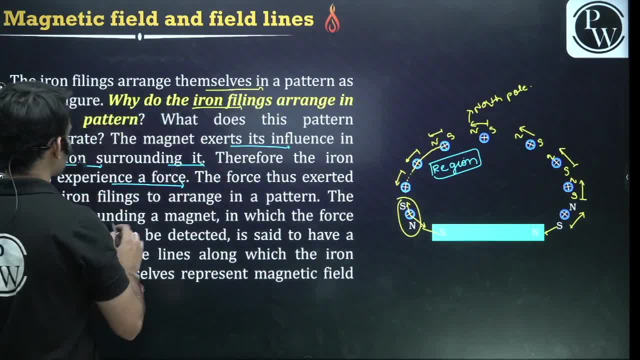 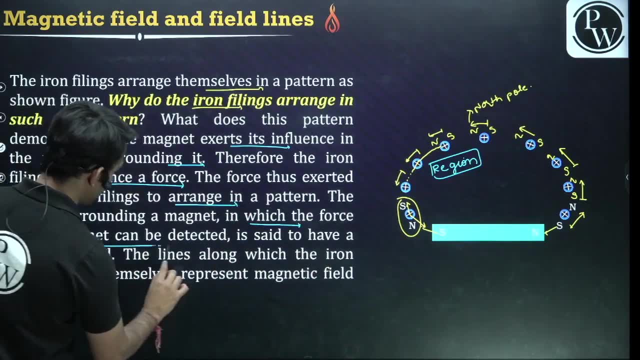 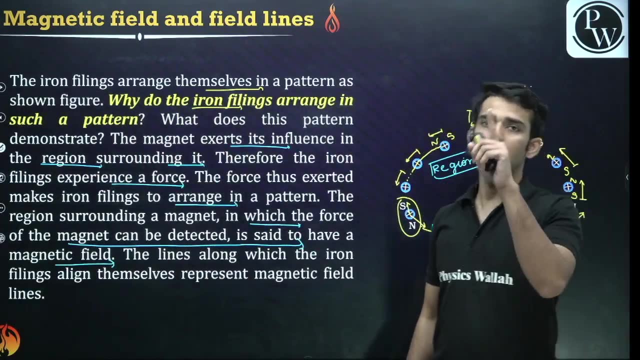 clear so the force that is exerted makes the iron fillings to arrange themselves in that pattern the region surrounding a magnet in which the force of the magnet can be deducted is called is said to have a magnetic field the region around any magnet in which you can observe the force that region around that magnet is the magnetic field of that magnet right guys so the lines along which the 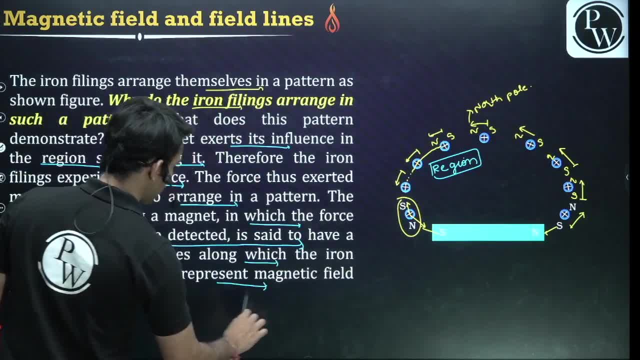 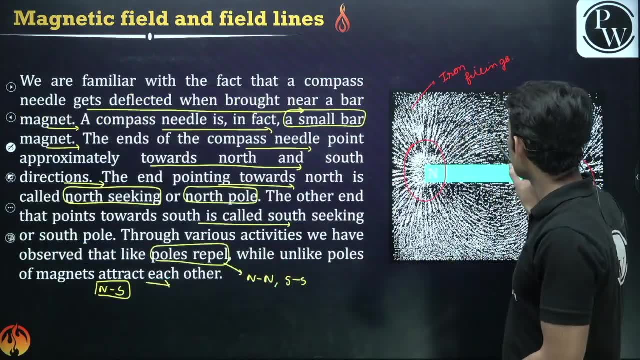 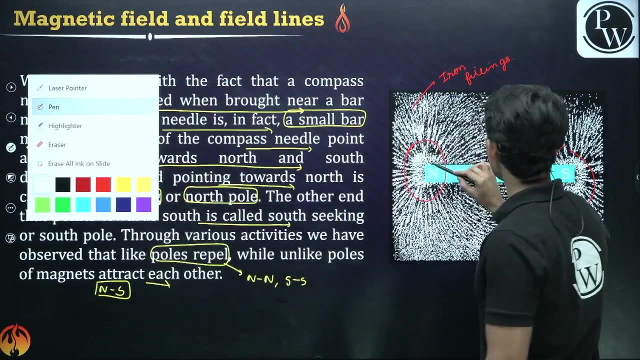 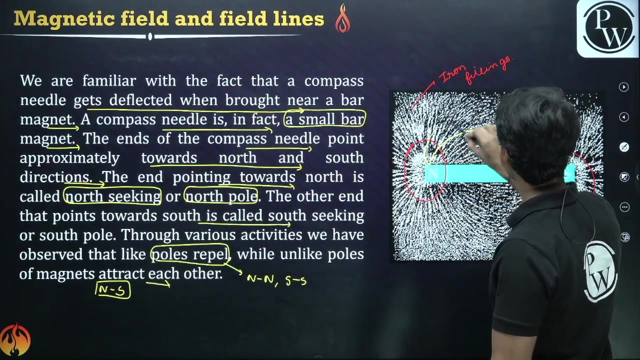 iron fillings align themselves represent magnetic field lines the field line the lines along which the magnetic field or the iron fillings arrange themselves like you can see the field kind of would kind of look like this can you see it basically the field kind of looks would look like this can you see it guys it kind of looks like this because the they have arranged themselves 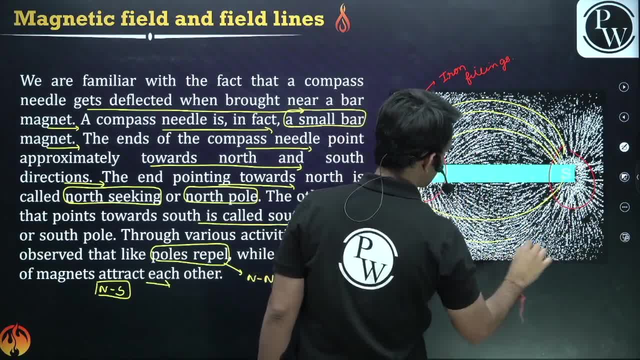 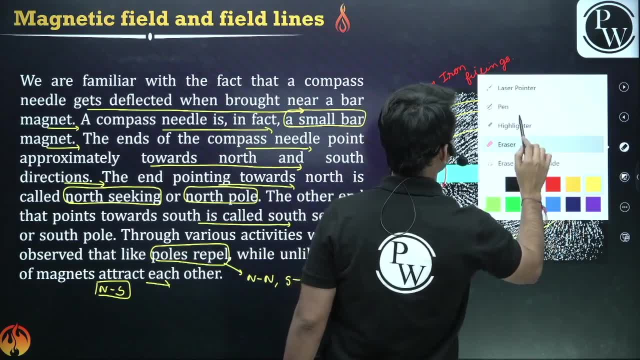 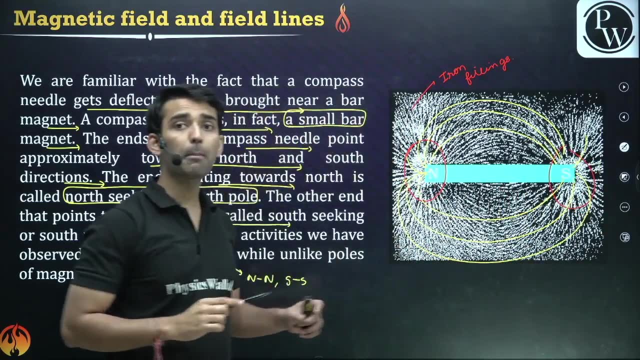 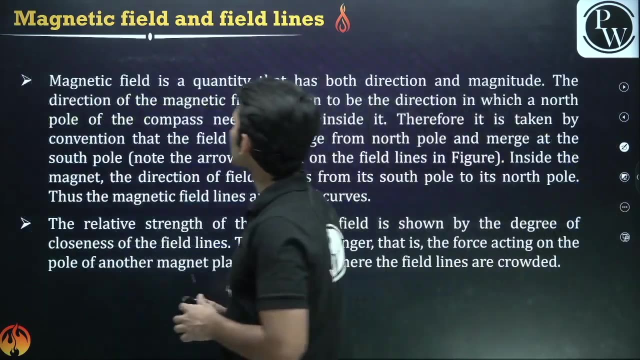 like this they have arranged themselves like this okay guys so this is the they won't don't intersect yeah so they kind of arrange themselves like this okay guys is it clear right so this is the pattern of the magnetic field lines clear so around any bar magnet fine guys now thing is how does the 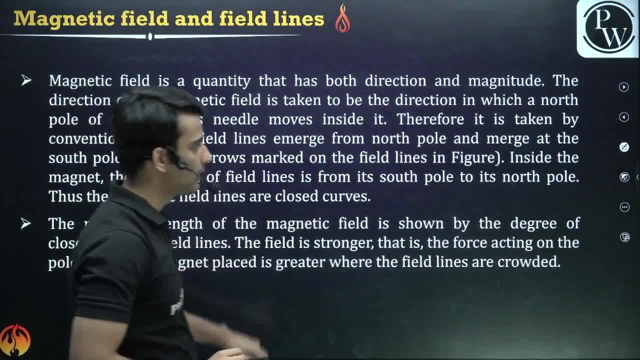 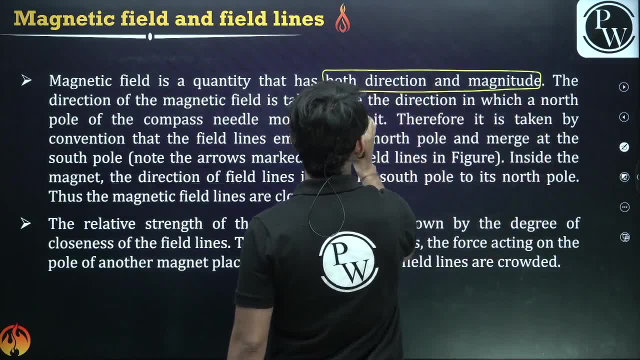 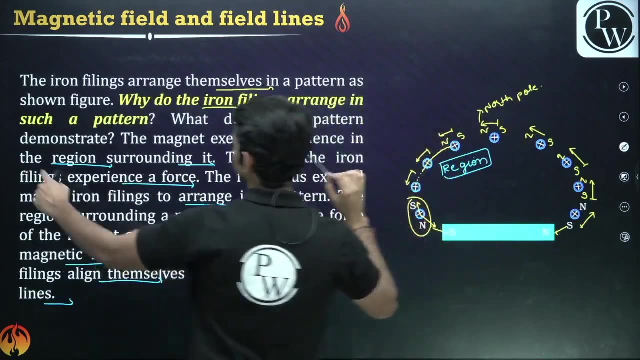 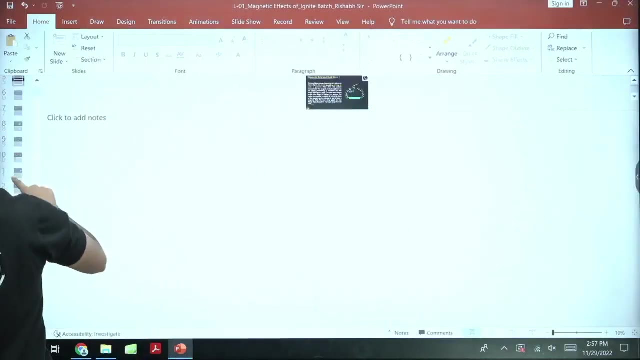 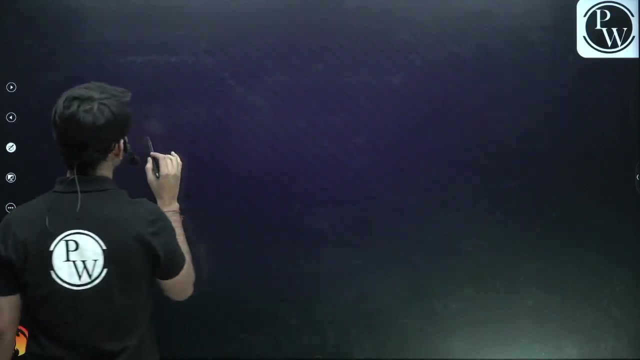 magnetic field I mean let's have a discussion of the magnetic field thing so that point is magnetic field is a quantity that has both direction and magnitude guys right how does a direction is specified see if you take if you take magnetic field at this point let me tell you how let's say if you ask hold on a second so guys basically it has both magnitude and direction let me tell you what is the meaning 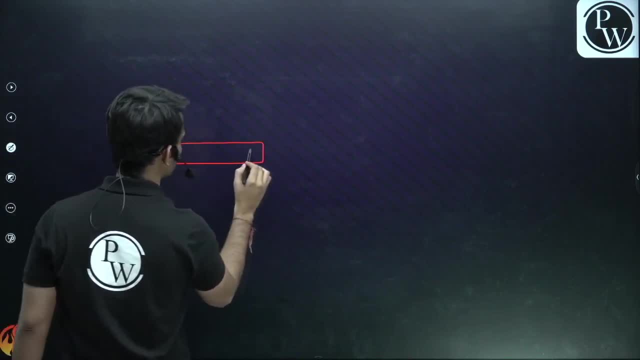 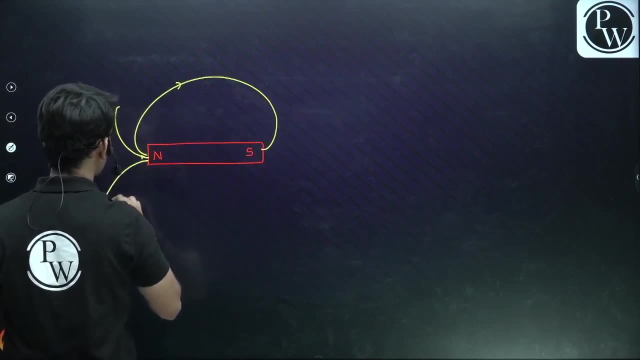 of this suppose if I draw any bar magnet this is North Pole this is South Pole right guys so basically the field lines kinds of arrange themselves like this right the kinds of arrange themselves like this right okay now the question is guys if I ask you the direction of 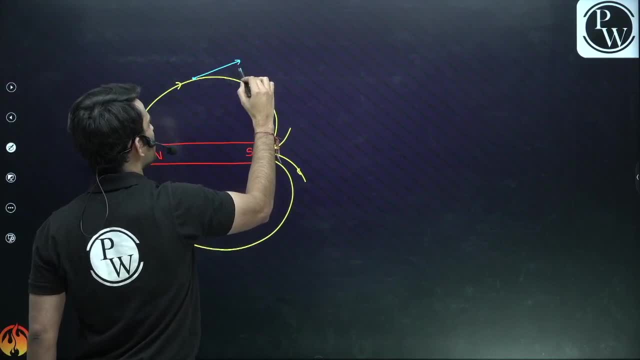 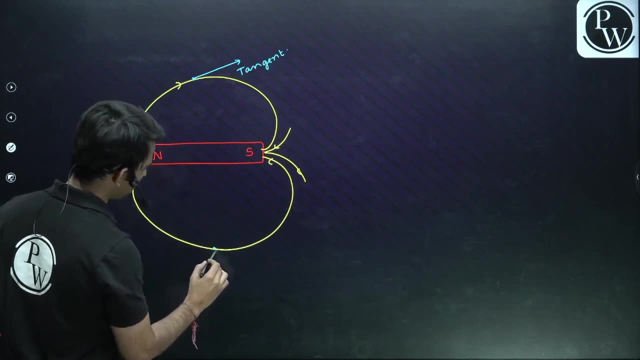 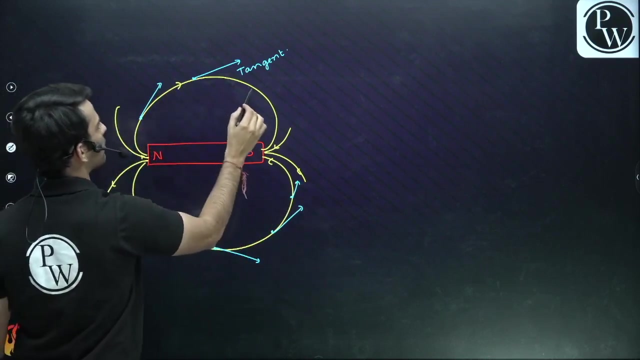 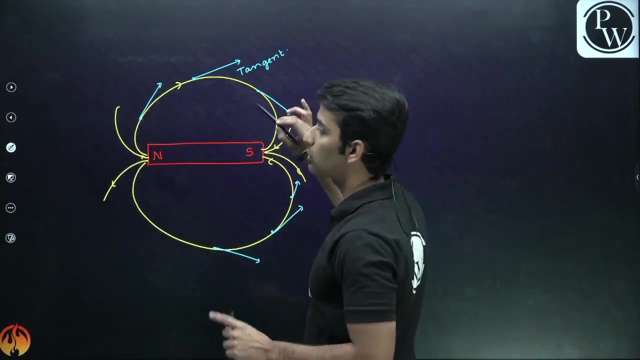 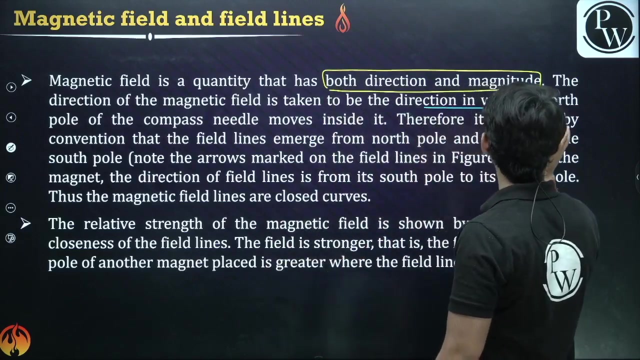 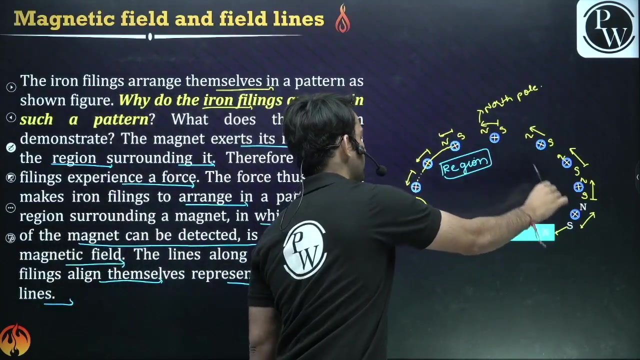 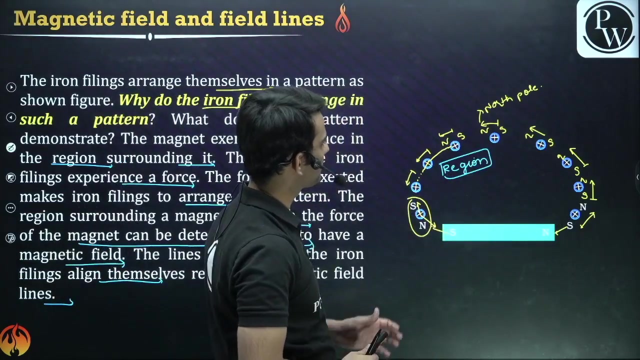 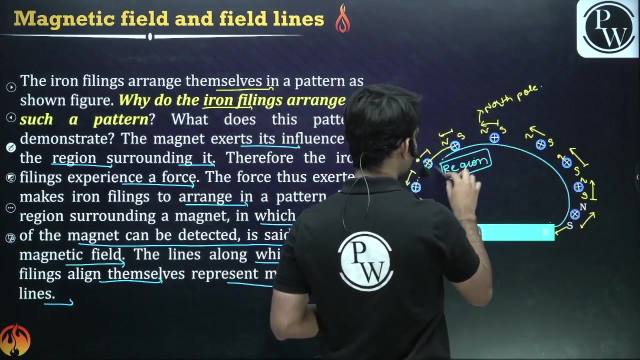 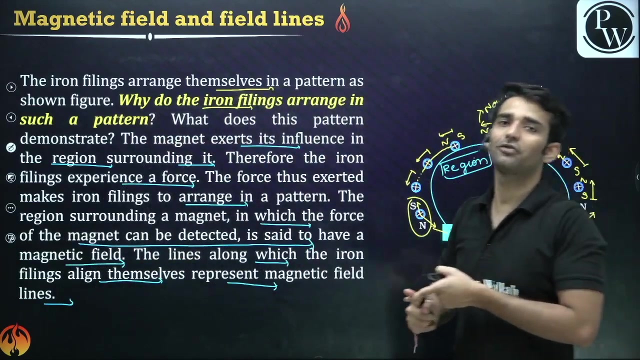 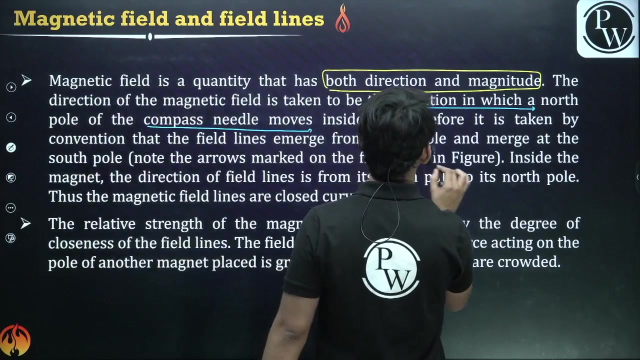 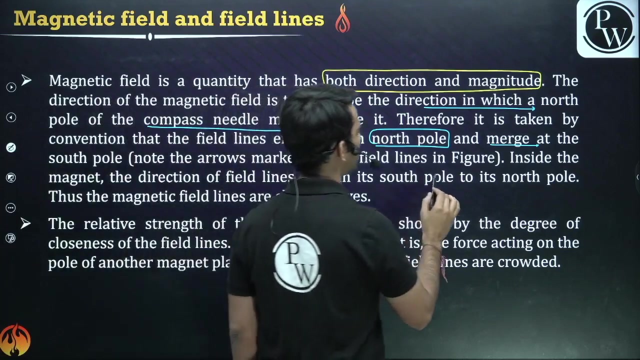 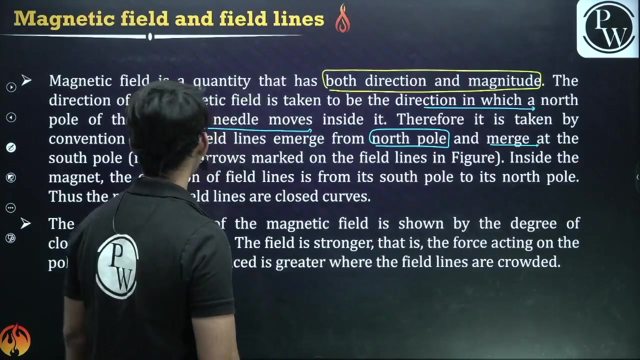 the magnetic field at this point so it will be along the tangent the magnetic field along this line would be along the tangent if I ask you direction of the magnetic field at this line it would be like this at this point it would be like this at this point it will be like this at this point magnetic field would be along this here it will be along this so basically a magnetic field at every point is along the tangent so it has both magnitude as well as direction the magnetic field that is what is written here so direction of the magnetic field is taken to be direction in which a North Pole of the compass needle moves so can you see it guys here the North Pole was moving in which direction basically the North Pole basically moving in this direction in which the compass the North Pole of the compass needle moves right so North Pole is moving in this direction so therefore magnetic field would be like this isn't it the direction in which compass the North of the compass needle moves that is the direction of the magnetic field clear so therefore it is taken by convention that field lines emerge from North Pole right emerge from North Pole and they merge or they terminate at the South Pole note that arrow marked on the field lines in the figure can you see the arrows basically they emerge from North and terminate at the South Pole right guys inside the magnetic direction of field lines is from South to North can you see it guys what is the direction of 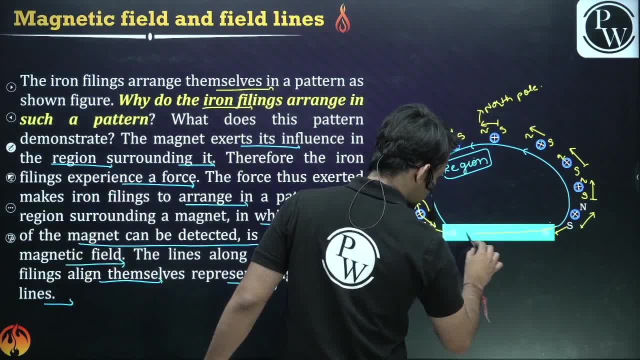 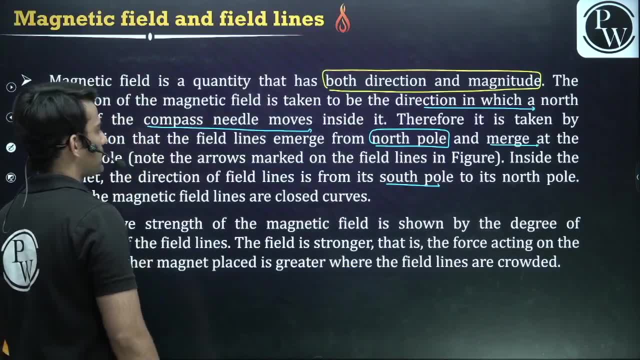 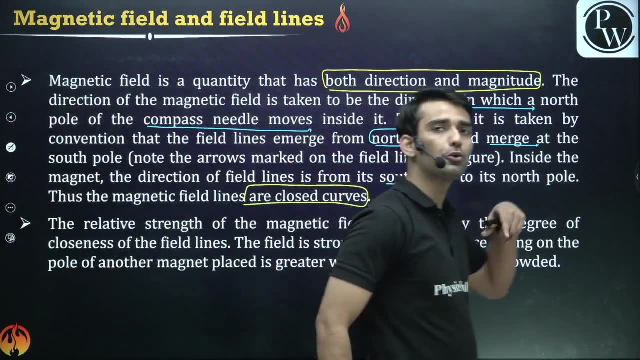 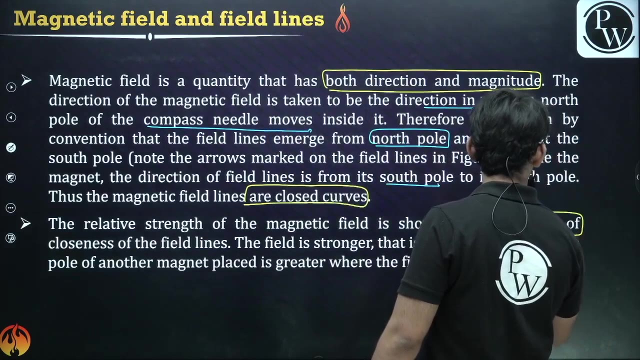 the field lines inside it inside it the field lines would be like this it is from South to North outside it is from North to South okay so basically you can see the field lines are closed curve the field lines form closed curve now how do you how do you check the strength of the magnetic field guys the thing is relative strength of the magnetic field is shown by degree of degree of closeness 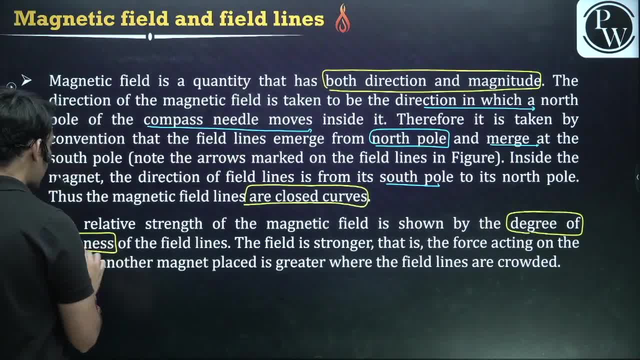 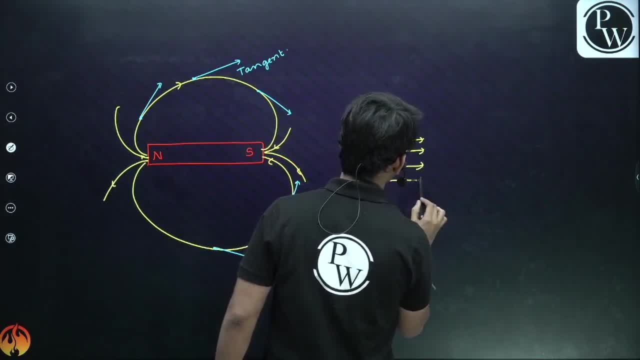 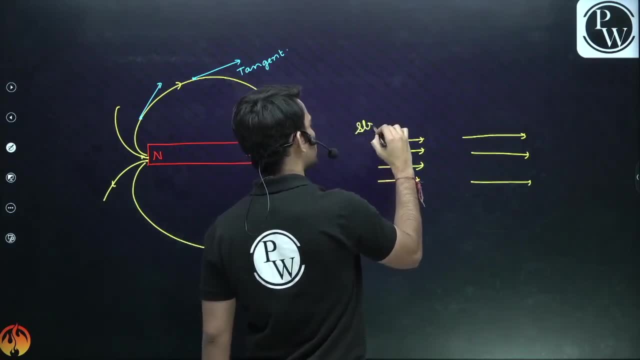 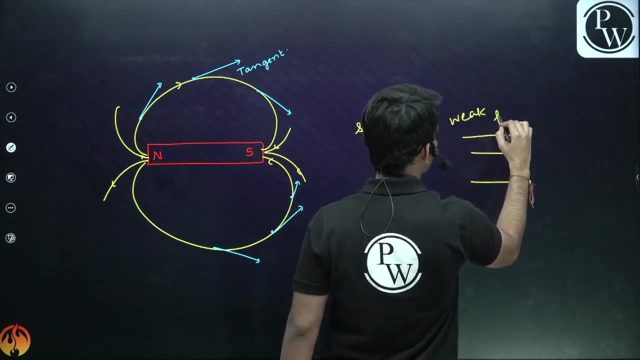 closeness of the field lines that means the more close the field lines are the strong would be the magnetic field at that point that means if I draw two magnetic fields this one and second is this one so guys which is a strong magnetic field this one is strong because here field lines are comparatively closer field lines are compressive comparatively closer this represents weak field this represents weak field okay 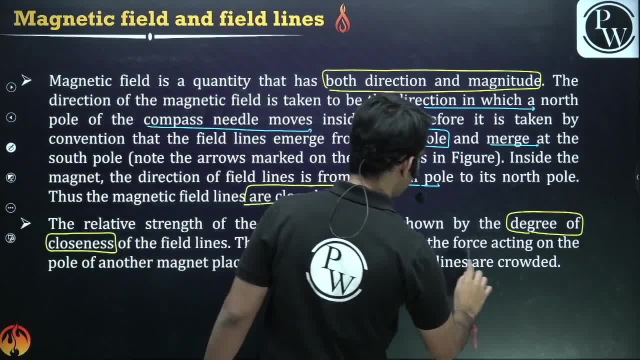 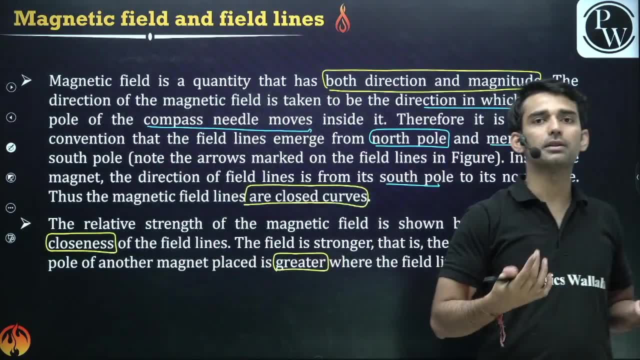 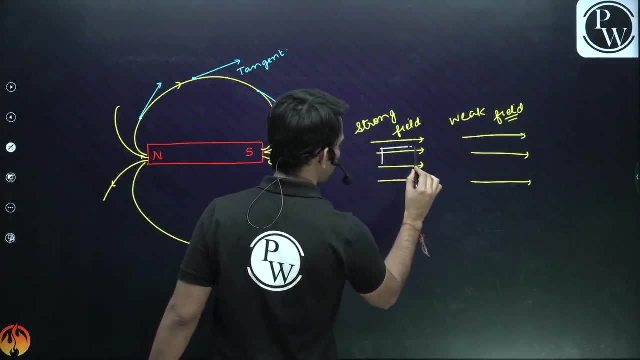 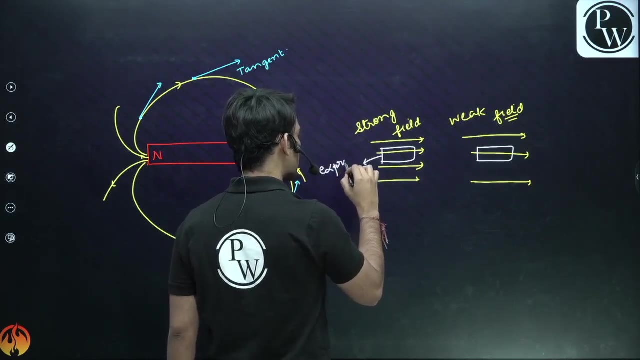 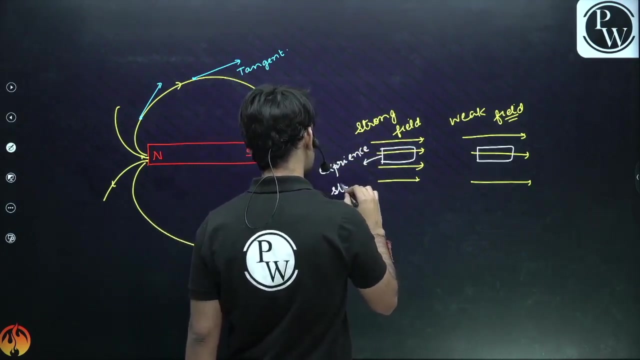 here the force acting on the closeness or the field is stronger that is the force acting on the pole of another magnet is greater you can see where the field will be strong the force will be strong that means if you place any bar magnet here let's say if you place any bar magnet here and any the same bar magnet here so here this bar magnet will experience stronger force why because here we have a stronger field stronger field means stronger force it will experience stronger force this is the point that you should be knowing it will it will 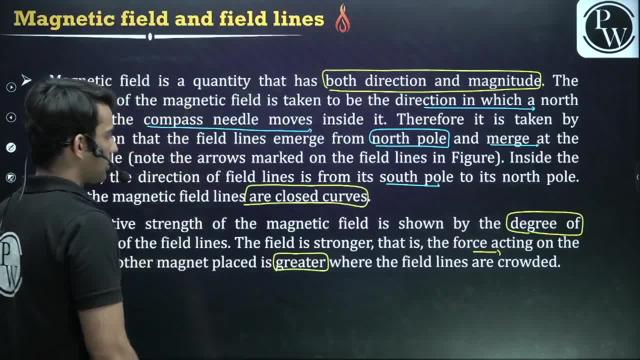 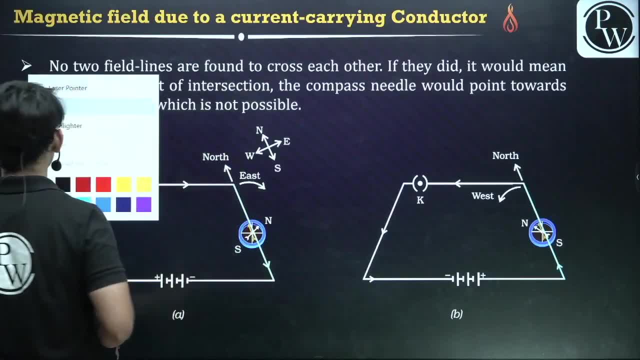 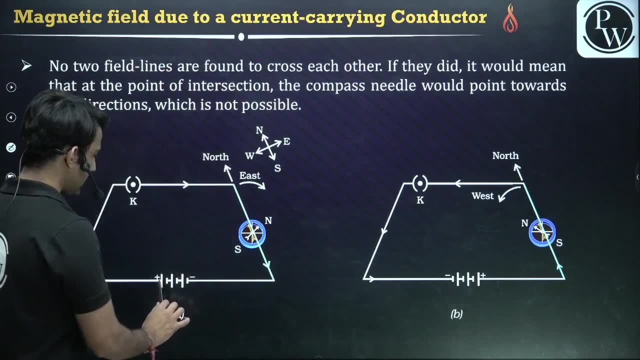 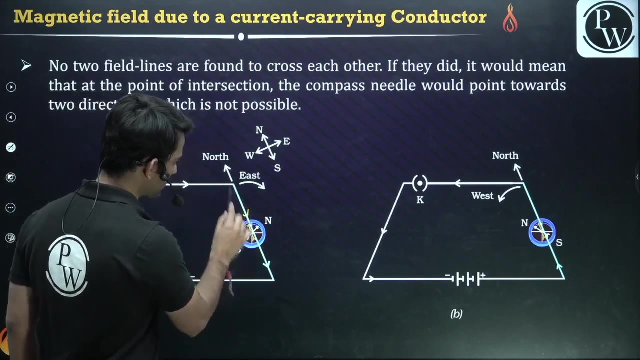 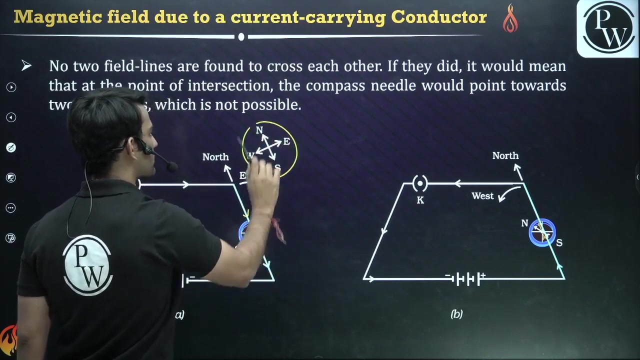 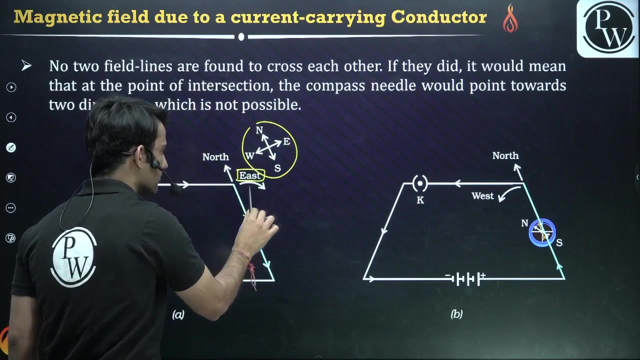 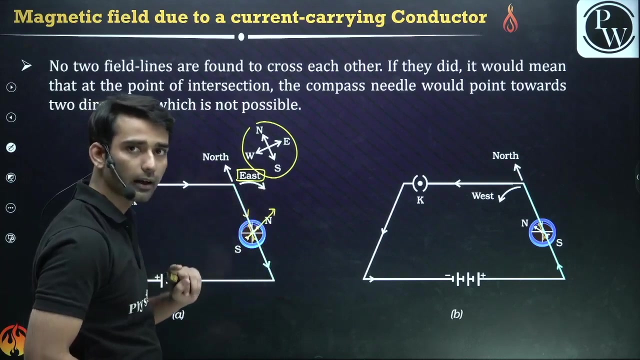 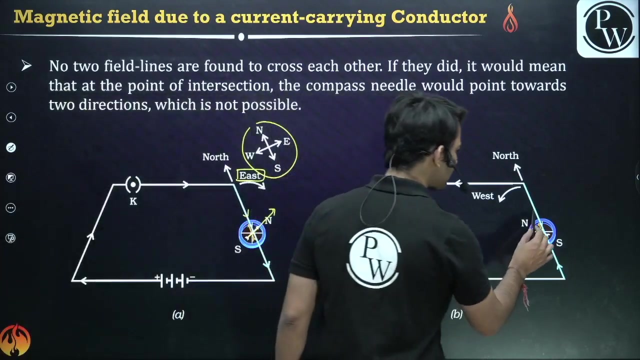 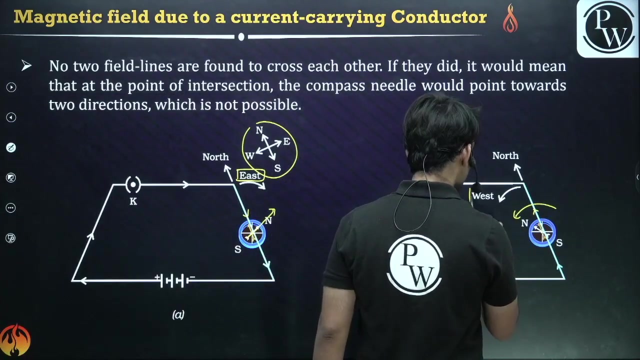 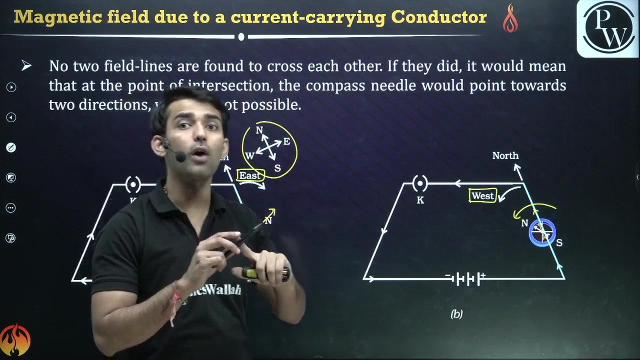 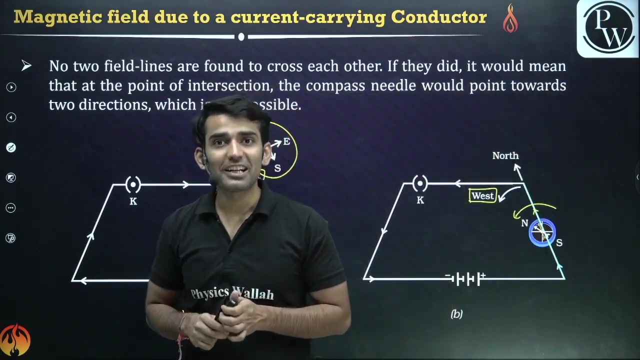 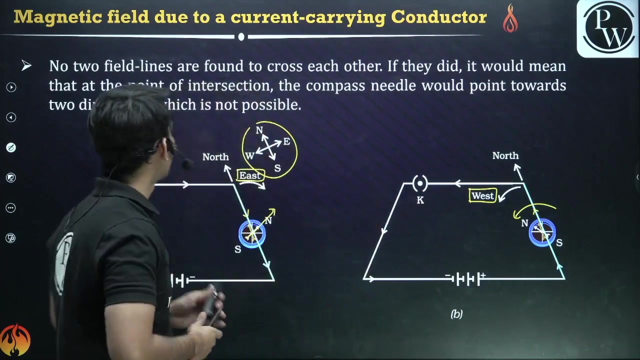 experience stronger force right guys right so where the field lines are crowded the field will be stronger right so this is the concept now thing is what are magnetic field due to current carrying conductor so guys we have taken apparatus let's say I have connected a battery a key right and we are flowing a current through this and this is the blue one is the copper wire current is going from this to this from upside down I have brought a compass needle here right this is North right can you see the direction guys this is North this is East this is West and below we have South so the compass needle has deflected towards East can you see it this is the North Pole so North Pole the compass needle is deflected towards it by this current carrying conductor now if you reverse the polarity of the battery can you see the battery polarity of the battery is reversed guys the direction of the current is reversed now it is upwards now you can see the magnet the North Pole is deflected towards West here it was East here it is West that means the deflection is reversed why because you have reversed the direction of the current and that reverse that has caused the magnetic field to reverse its direction and that is that is why the deflection is reversed okay guys fine now 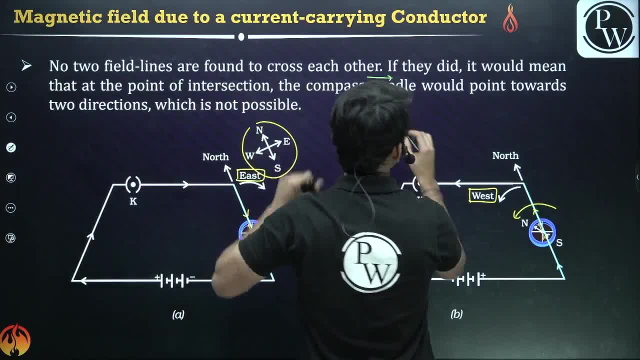 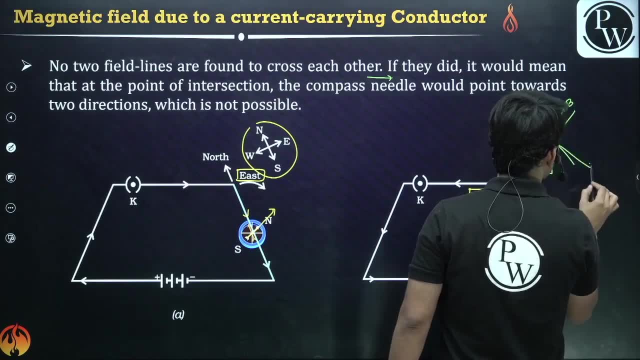 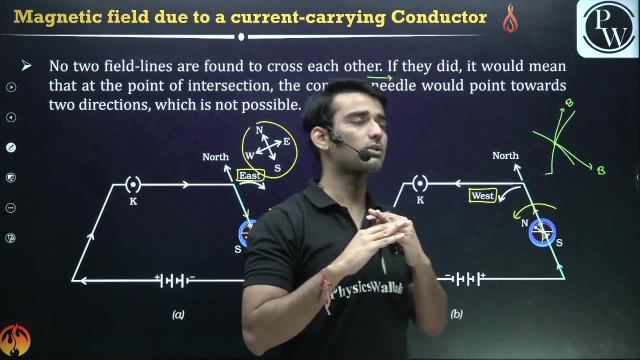 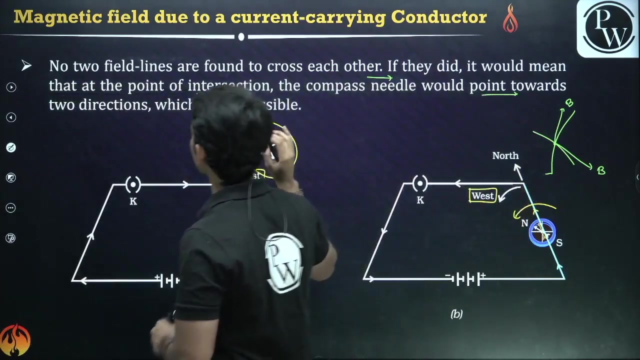 two no two magnetic field line found to cross each other why guys see if two magnetic field lines cross each other that means at this point one magnetic field would be this one would be this is it possible to have two direction at a single point no so that means no field two field lines can cross each other that would mean uh that the point of intersection the compass needle would point towards two direction which is not possible you cannot have two direction at a single point 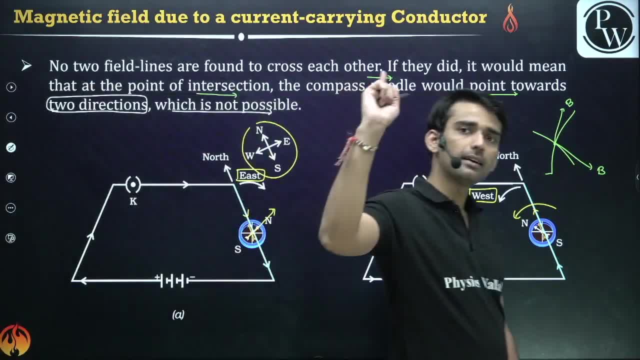 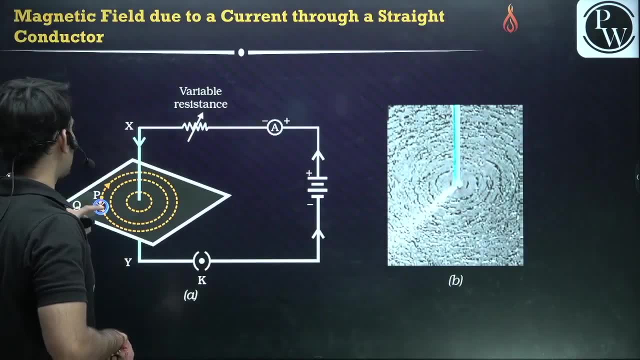 which is not possible clear guys only single point single direction at a single point fine now the question is how can we recognize the magnetic field due to a straight current carrying conductor 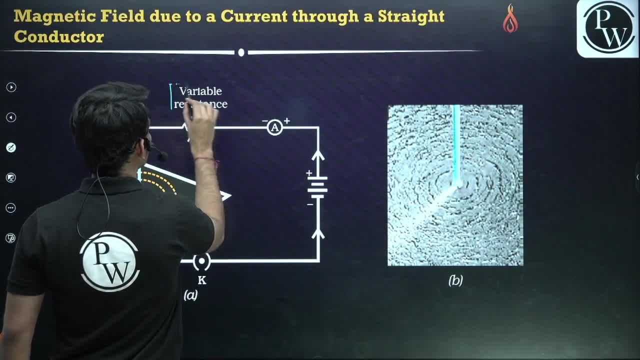 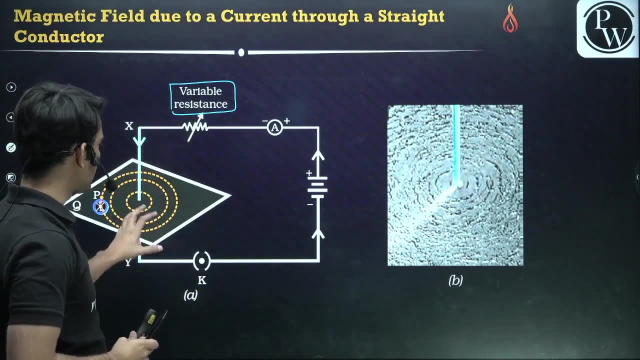 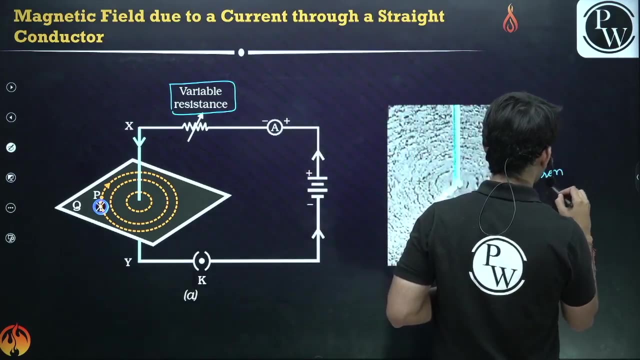 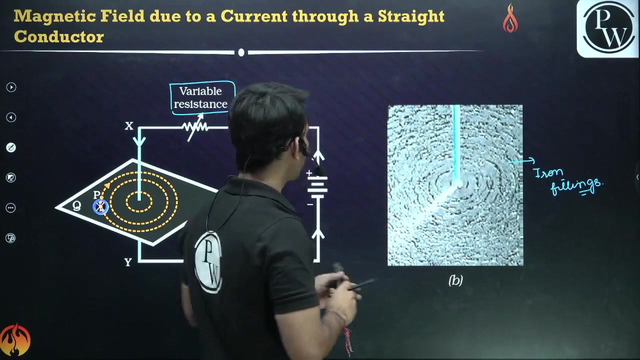 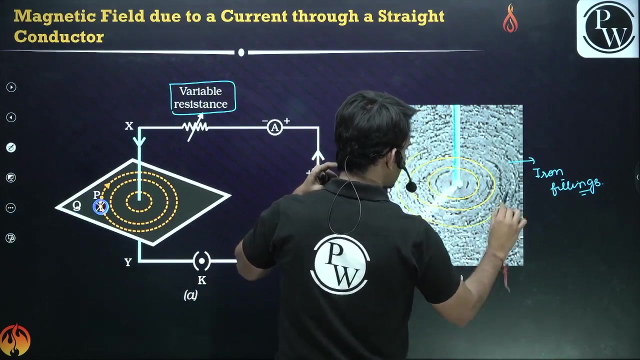 guys I have taken same apparatus we have a variable resistance to change the current we have emitter we have battery we have key I have what I have taken I have taken a cardboard right with right guys and on this cardboard I have sprinkled iron fillings I have sprinkled iron fillings fillings now guys what they had seen that after some time the iron fillings arranged themselves in this pattern in this pattern like this can you see it they kind of arranged themselves in a pattern like this now why is it so the magnetic field should be in this direction should be like 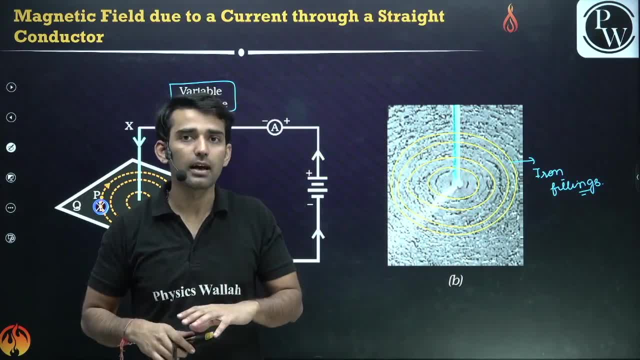 this that's why the iron fillings have experienced the some force in that direction and as a result arranged themselves like this so Singh is 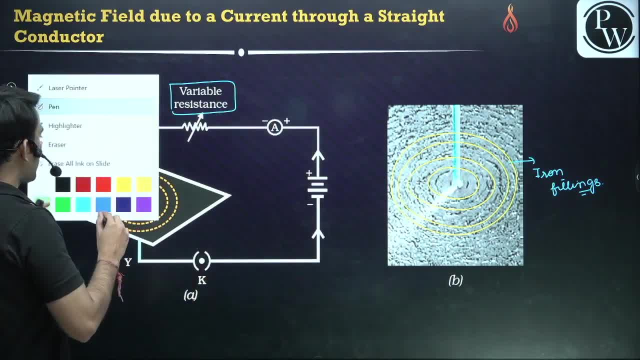 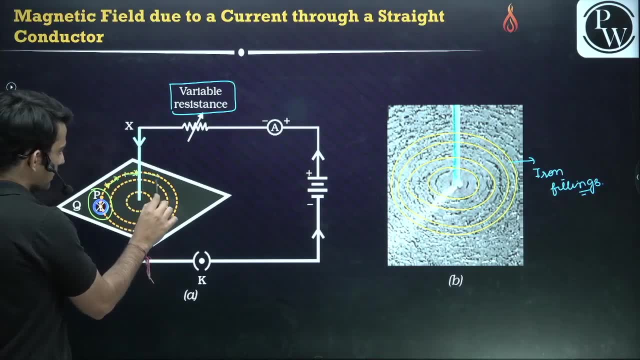 if you draw the magnetic field due to straight current carrying conductor or you can also check this with the help of a compass needle the compass needle would move like this the compass needle at every point would move like this that means guys the direction of magnetic field due to straight conductor is like this they are concentric circles what are they guys can you 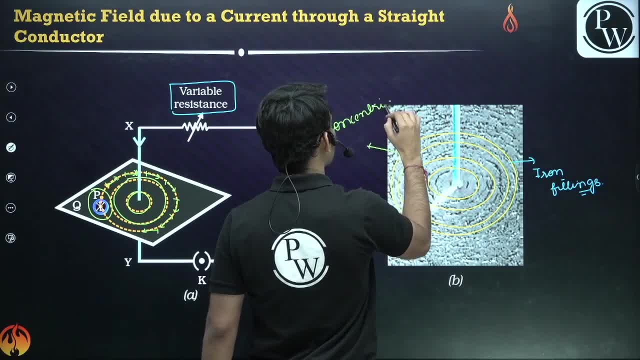 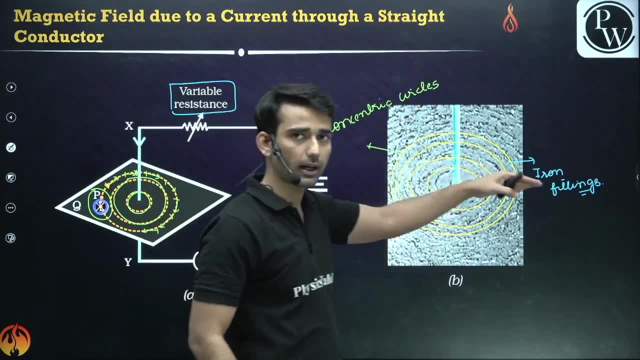 observe this they are nothing but concentric circles contraints contraint sale centric circle all circles are having a same center but their radius is different it is increasing right so 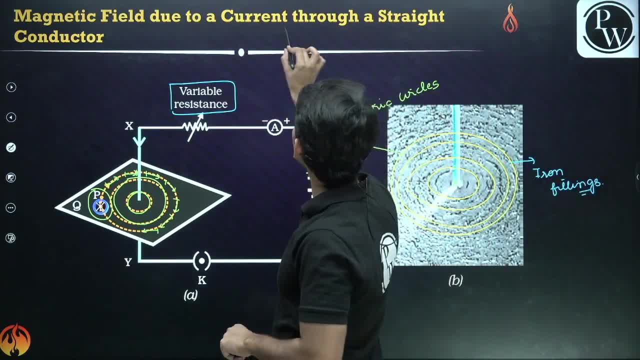 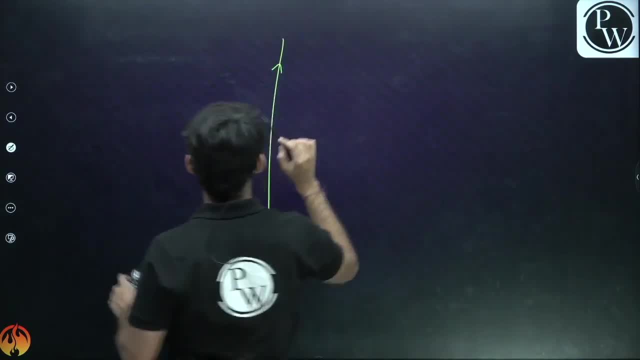 these are called concentric circles so magnetic field due to a straight current carrying conductor is concentric circles how how do they look like if I draw the any wire the magnetic field due to 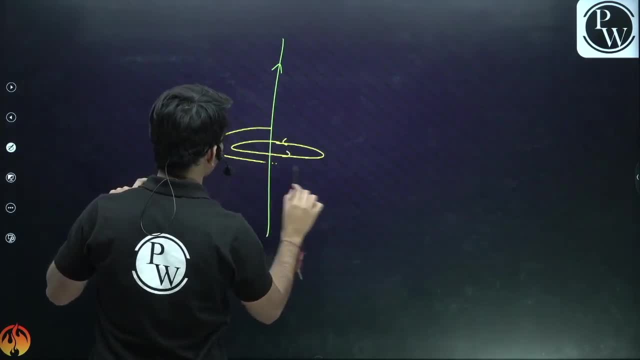 this will kind of look like this will kind of looks like this okay guys are you getting it the magnetic field kinds of look like this concentric circles okay so 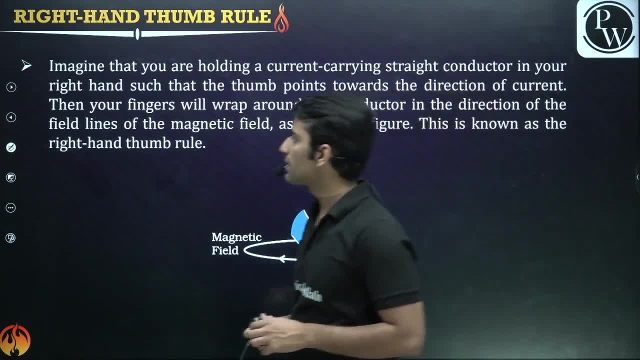 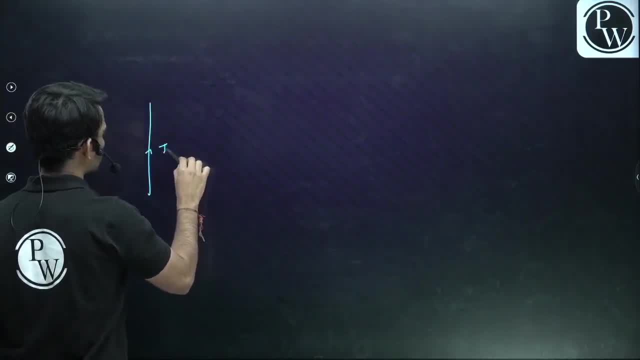 to the straight current gaining conductor now thing is how can we find the direction see basically guys thing is we can have two two direction let's say if current it upwards in the second case current is downwards so guys current is reversed so that means the magnetic 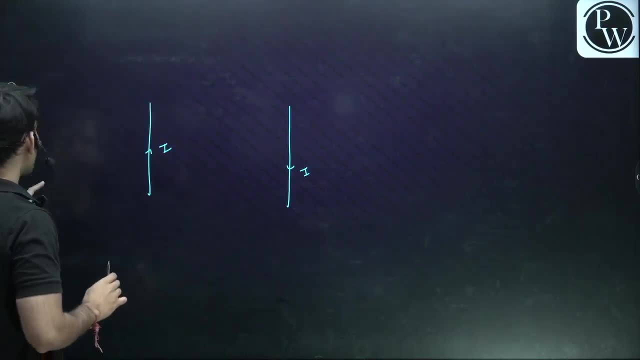 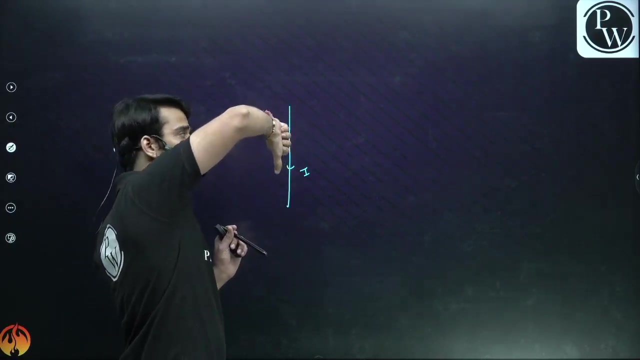 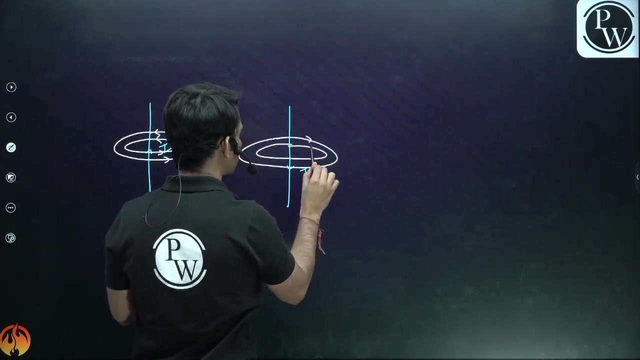 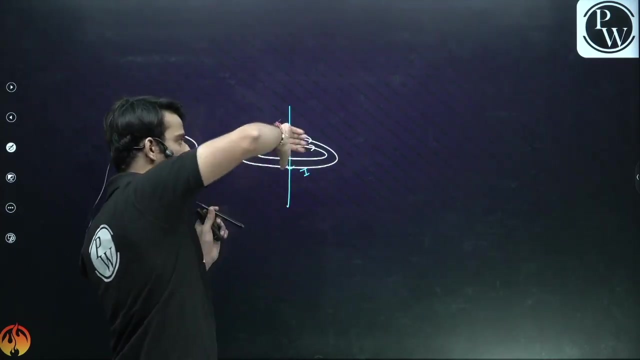 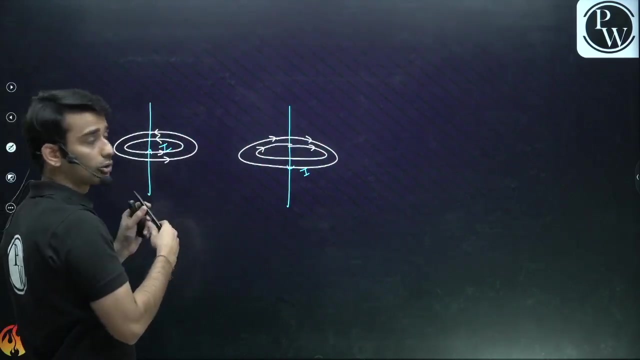 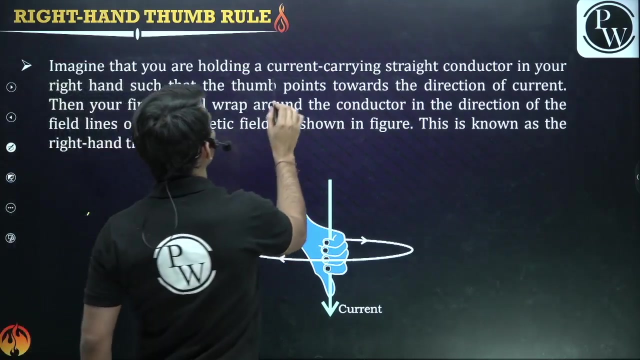 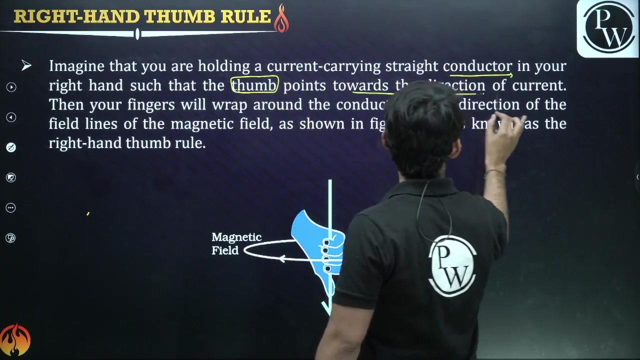 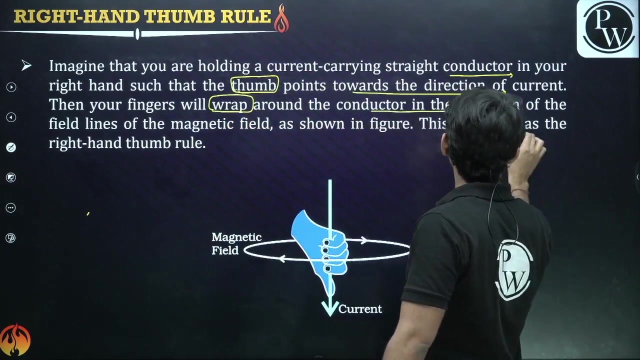 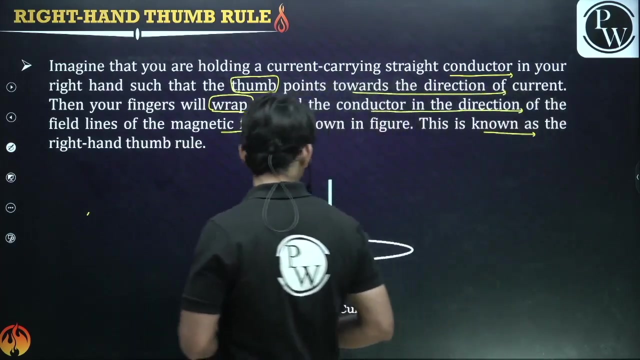 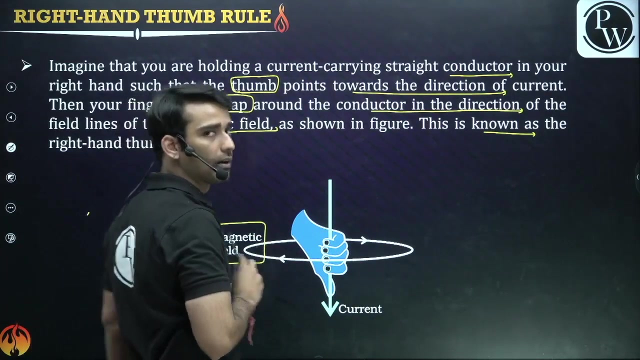 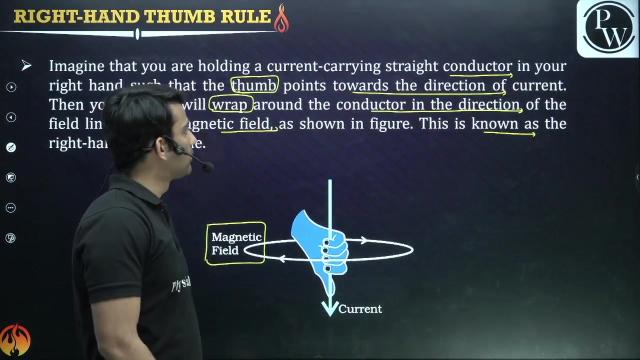 field would also have been reversed so guys what you have to do just take your right hand fingers and the thumb put the current thumb in the direction of the current so you can see the direction in which your fingers are curled your fingers are curled is like this it's it isn't it like this the direction in which fingers are curled is like this right but here put your thumb downwards so though they are same concentric circles but here if you draw the direction guys if you draw the direction they are kind of like this right they are kind of like this so here magnetic field okay bye bye okay so fine fine fine we have drawn right magnetic field is like this here magnetic field is like this so direction is reversed so guys this rule is known as right hand thumb rule what does it state that you are holding a current carrying wire straight in your right hand such that thumb points in the direction of the current thumb should be in the direction of the current then your fingers will wrap fingers will wrap like this around the conductor in the direction of field of in the direction of field lines or this is known as right hand thumb rules can you see it thumb is downwards the direction in which fingers are curled it gives you the direction of the magnetic field very very simple direction of magnetic field due to a straight current carrying conductor you can find by this rule okay fine 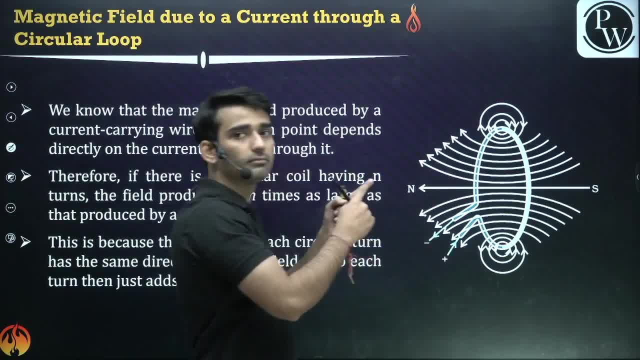 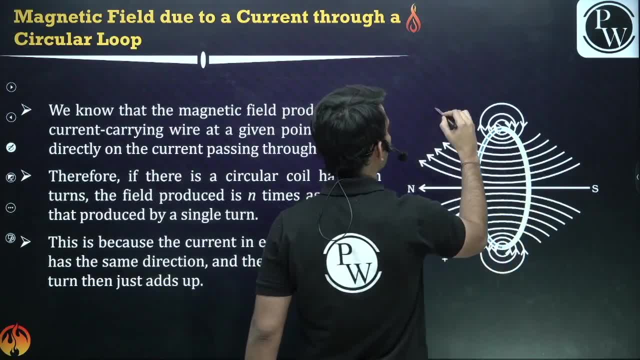 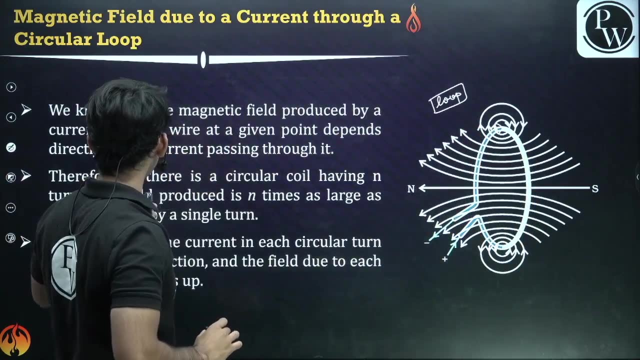 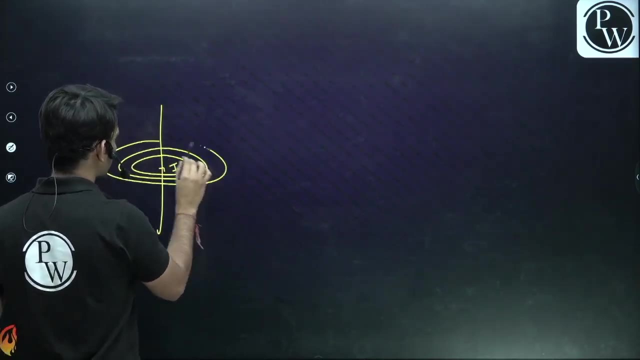 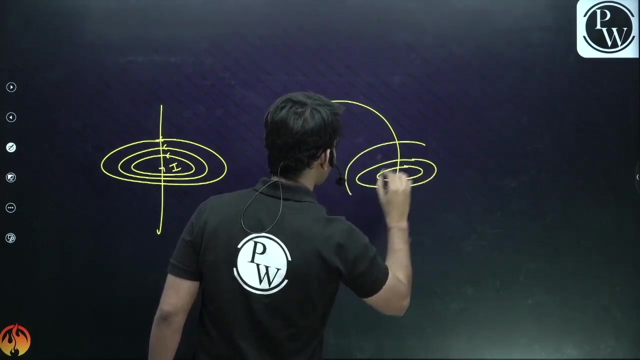 now question is what if i bend the wire right what if i bend the wire right so guys if you bend this wire in the form of a loop this is nothing but a loop this is not a straight current conductor now this is a loop now so guys here what what would happen see the wire would have been like this the and the magnetic field would have been like this right but if i bend this wire don't you think so the pattern of magnetic field is like this the pattern of magnetic field is like 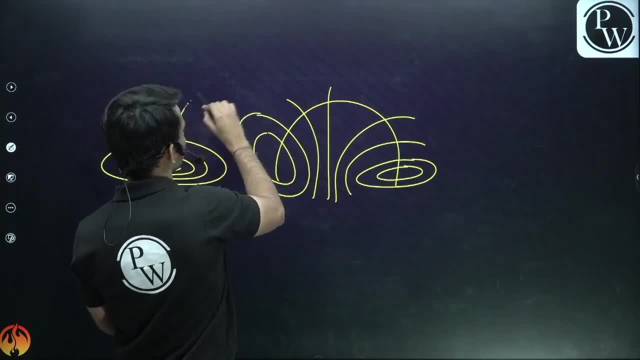 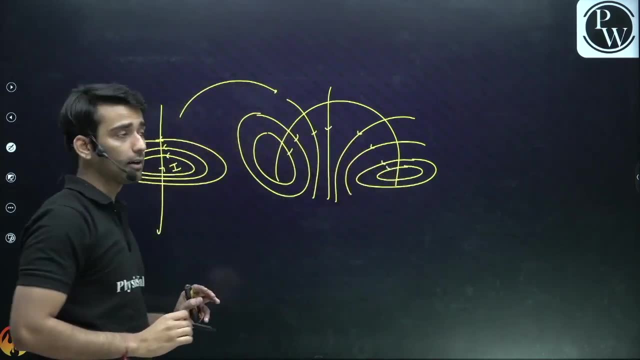 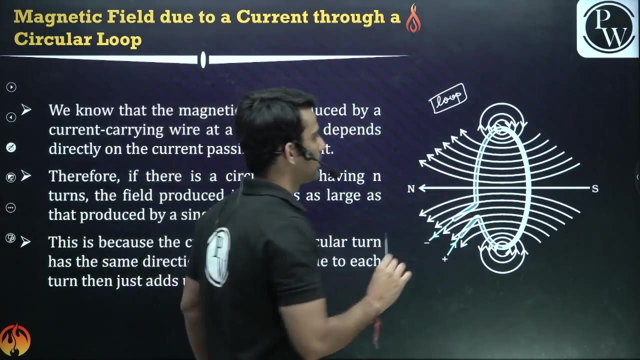 this isn't it guys right if you bend this wire the magnetic field the pattern of magnetic field is like this okay so that means if you draw the pattern of magnetic field due to a circular wire though they are same concentric circles and the pattern kind 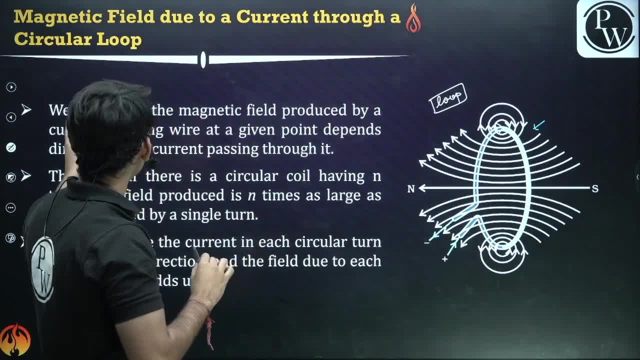 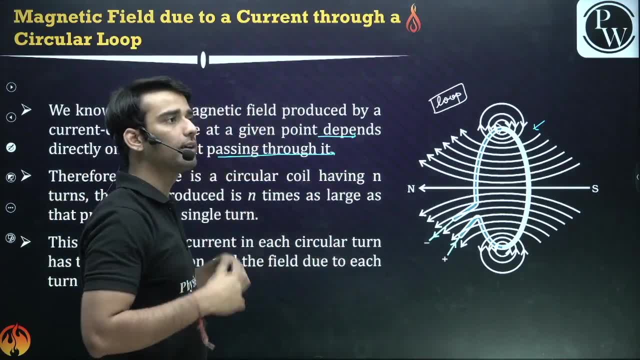 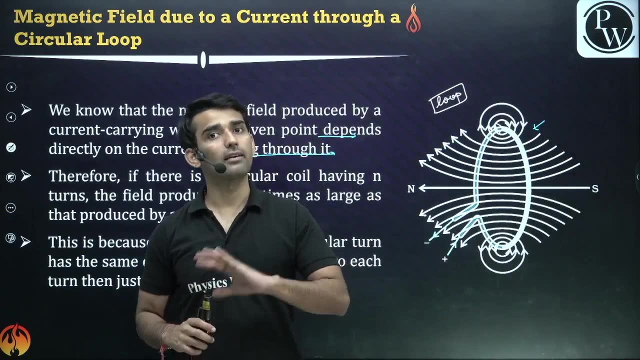 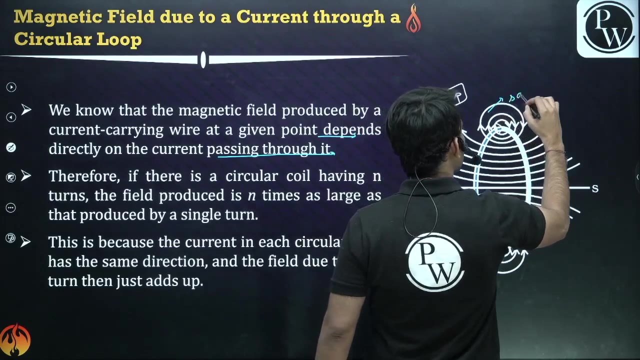 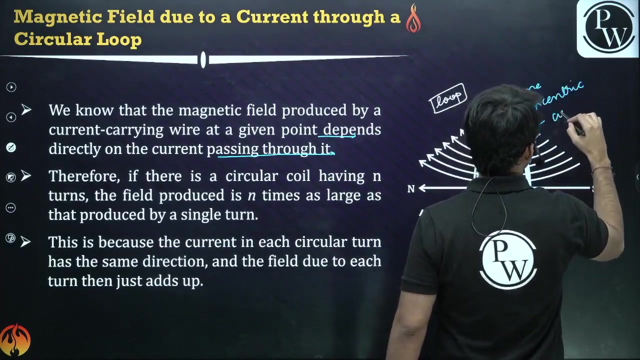 of looks like this you should be you should be knowing how to draw this so magnetic field produced by current carrying wire at a given point depends on the directly on the current passing current it depends on the current if you increase the current magnetic field will increase if you decrease the current magnetic field will decrease if you reverse the current magnetic field will direction right so it depends on the current okay guys so you can see they are same concentric circles the pattern is kind of same they are same concentric circles okay so therefore it is a 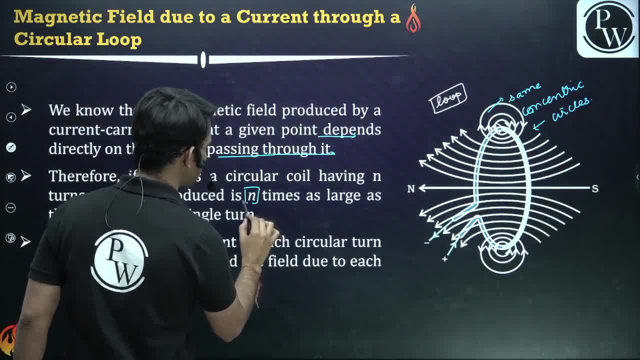 circular wire having turns the field produces n times see guys this is single turn what if i take 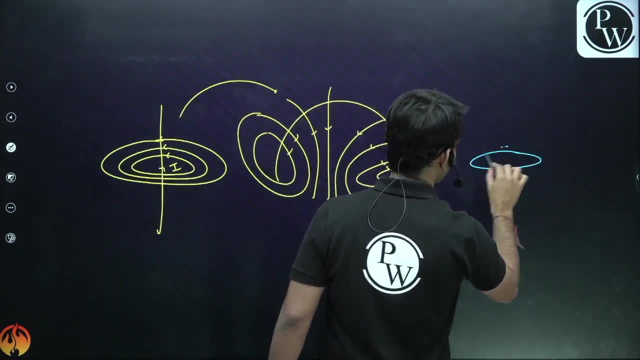 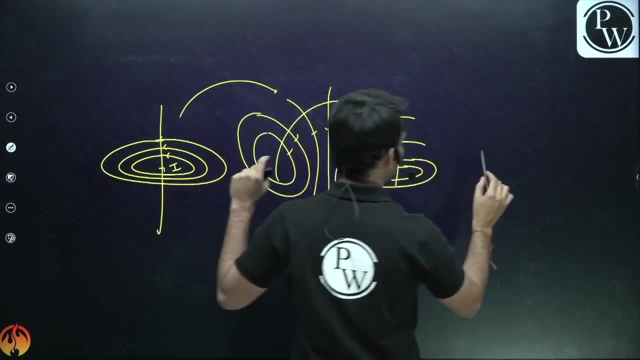 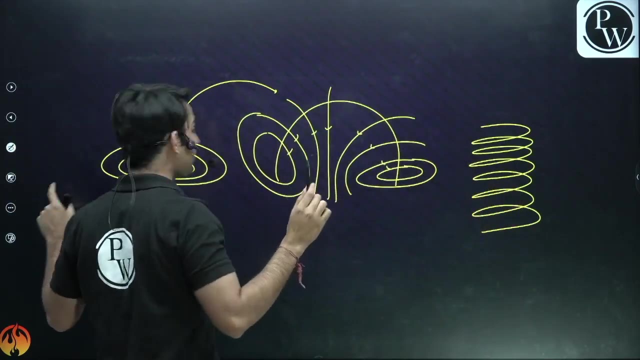 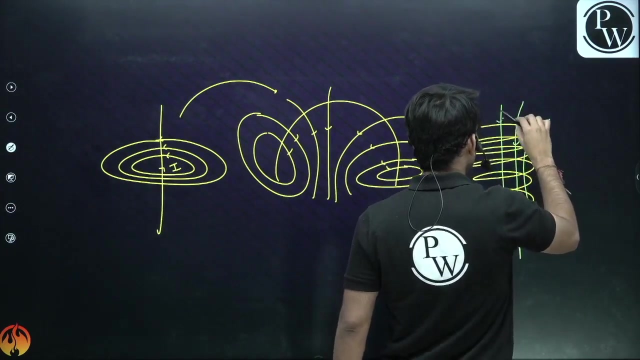 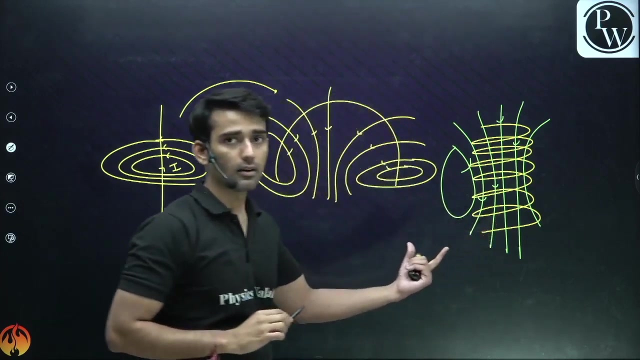 n turns what if i take n turns number of turns could be possible see this is the magnetic field due to a single turn but if i take n number of turns like this what would happen the magnetic field due to each turn would add up so they kind of looks like this isn't it due to each turn the magnetic field would add up okay guys so they kind of looks like this okay so n number of turns if number of turns is n the magnetic field total 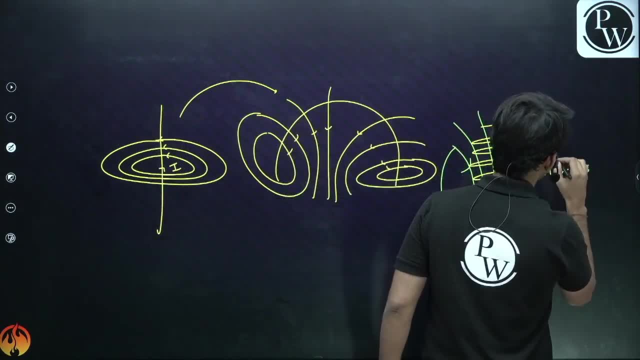 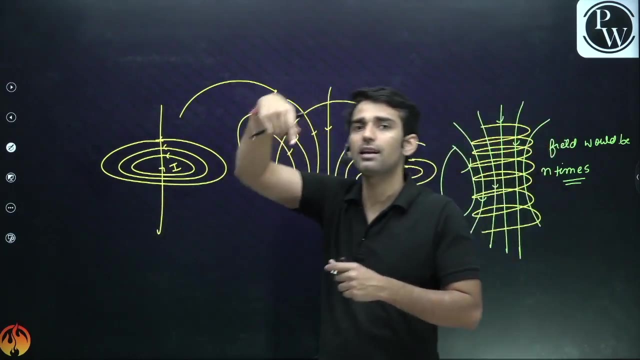 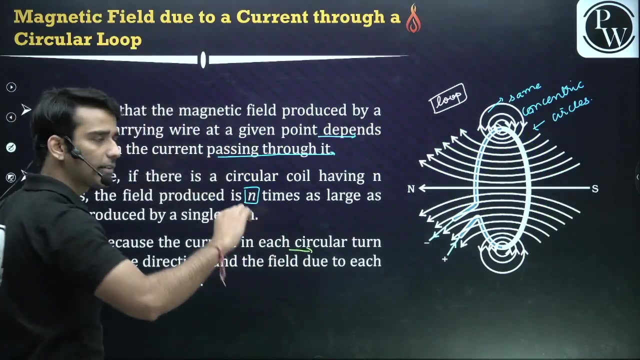 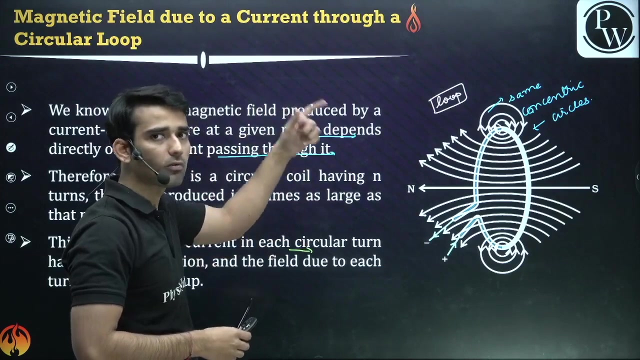 would be n times field would be n times field because field due to each turn is added up right field would be n times number of if you increase the number of loops or number of turns one turn two turn three turn four turn and so on okay fine so this is because current in each because see we have a current all in all the curve it's uh because basically the current in all the loop is clockwise clockwise clockwise let's say so the magnetic field due to each turn would add up 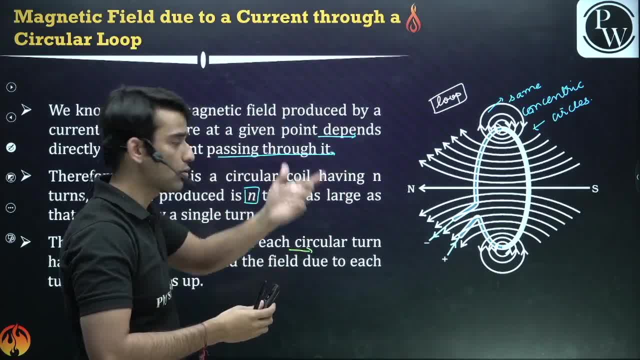 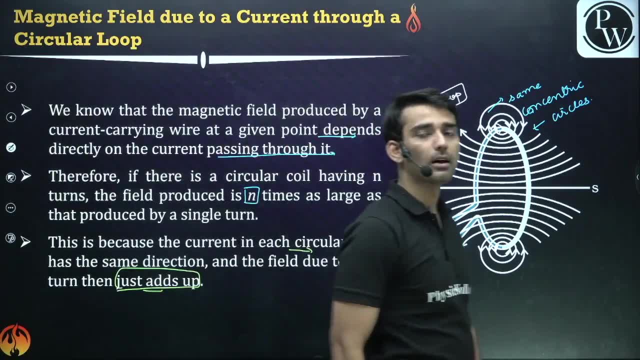 so that we will getting we will be getting stronger more strong magnetic field right and the field line just add up the magnetic field lines just add up okay clear guys 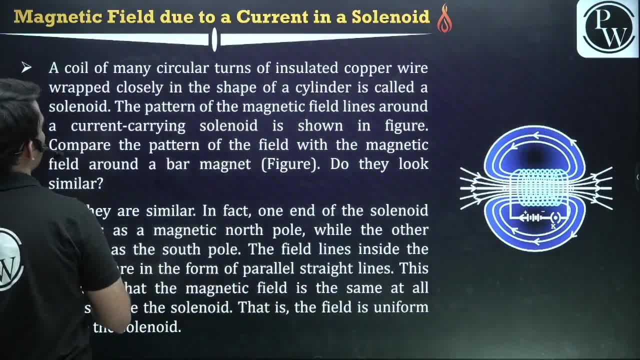 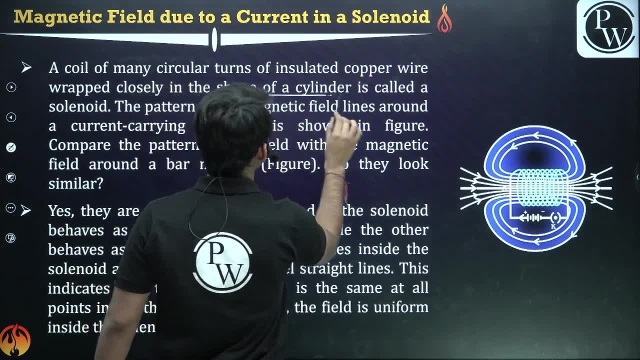 now what is the magnetic field due to a solenoid what is the solenoid guys basically if you take any coil and wrap it around any soft iron core or wrap it around in the shape of a cylinder best is known as the solenoid guys what do we call it solenoid so the pattern of the magnetic field 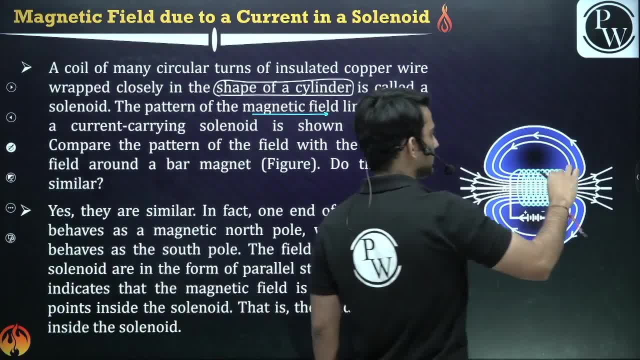 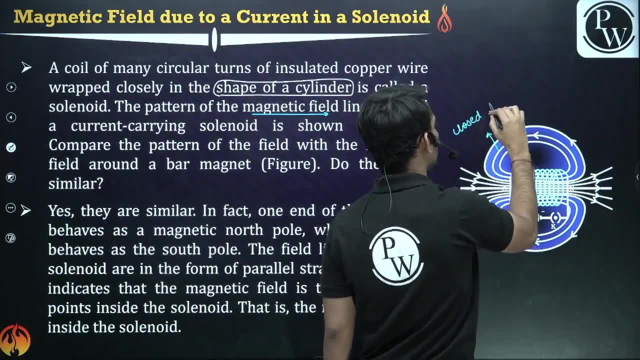 lines around a current carrying solenoid is shown can you see it guys the field lines again are concentric they are closed loop just remember this line the field lines always form closed loops 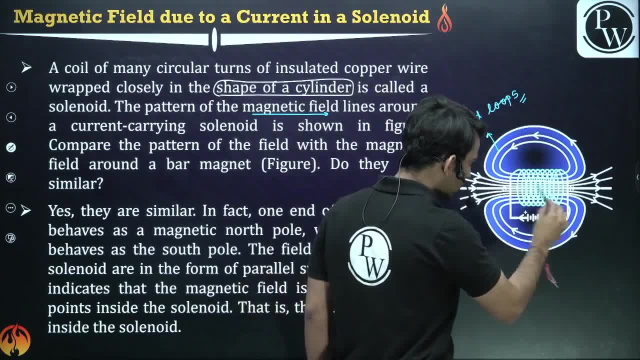 whatever the shape of the conductor is you can see they are forming closed 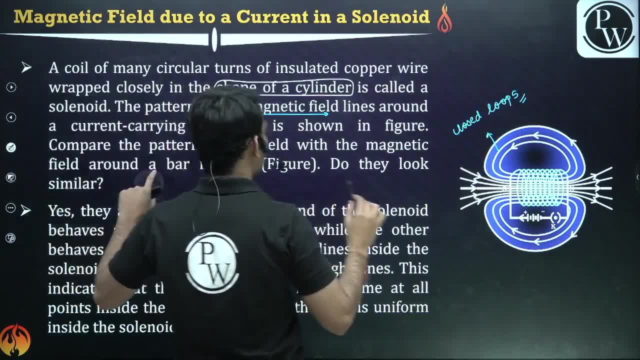 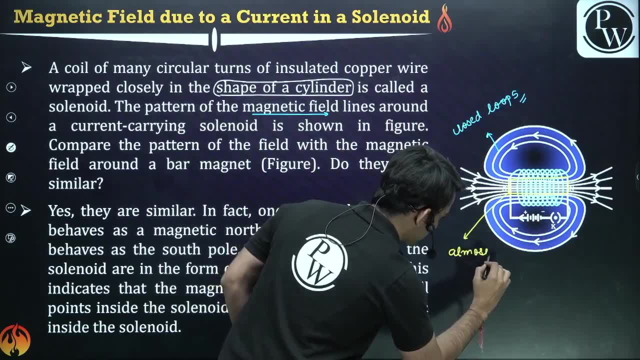 loop but there is one thing to notice is at the center can you see the field lines are almost can you see it guys the at the center the field lines are almost parallel 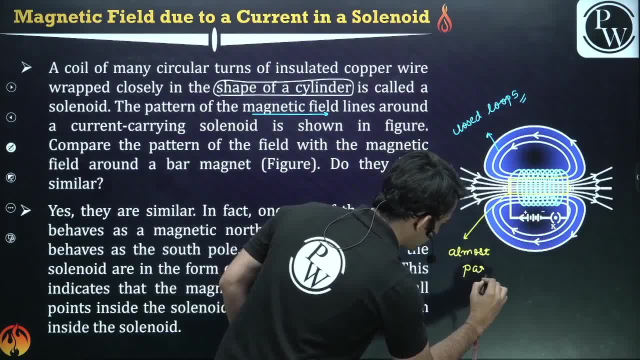 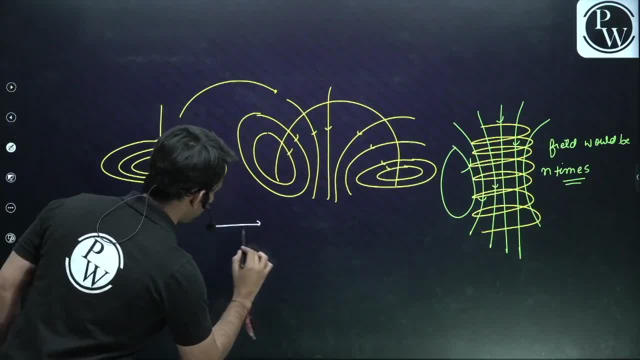 parallel means the magnetic field is uniform guys if field lines are equidistant and they are 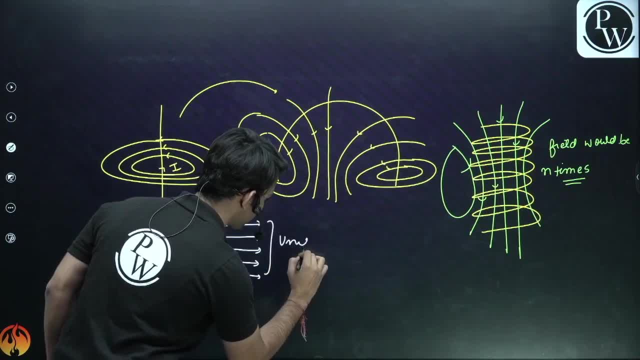 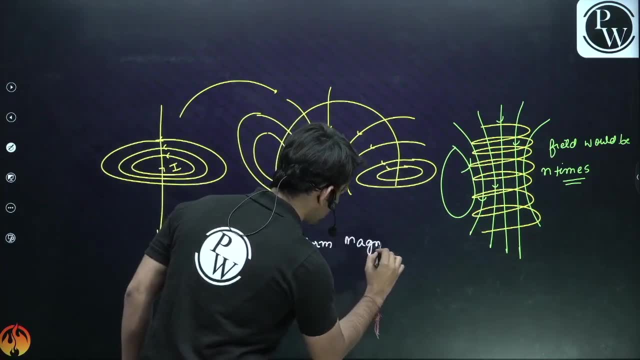 parallel this represents uniform magnetic field that means it is constant at every point in this region this represents uniform magnetic field this represents uniform magnetic field 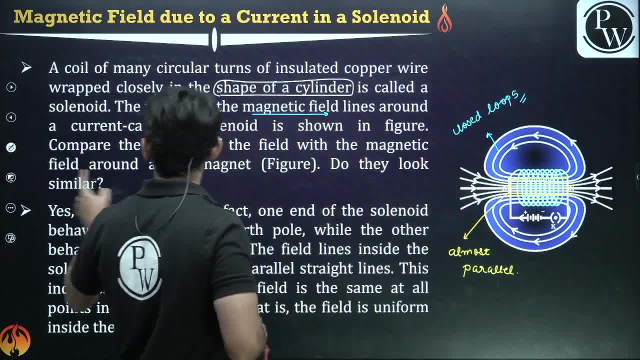 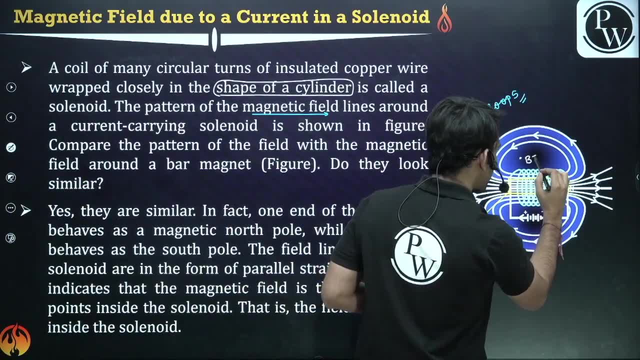 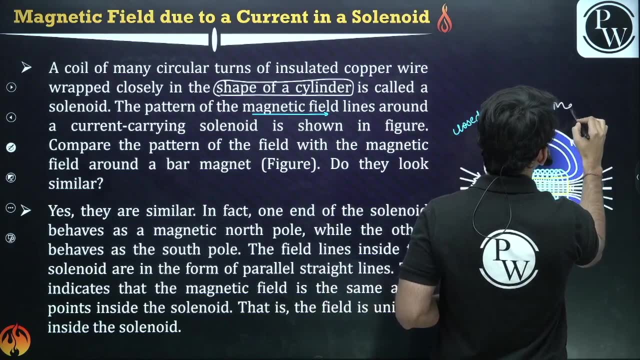 so magnetic field inside a solenoid is uniform but guys what if i ask you what is the magnetic field at this point if are there any field here no that means at this point magnetic field b we denote b magnetic field by b so guys at this point magnetic field is zero can you see it 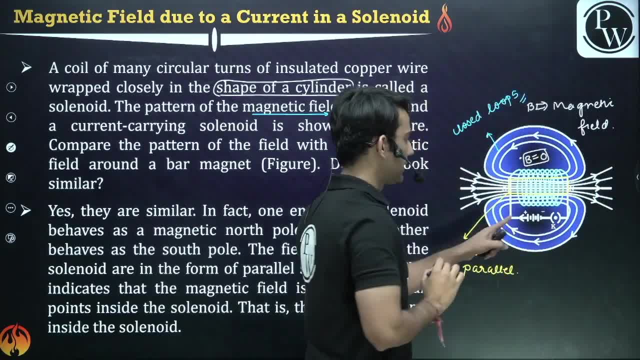 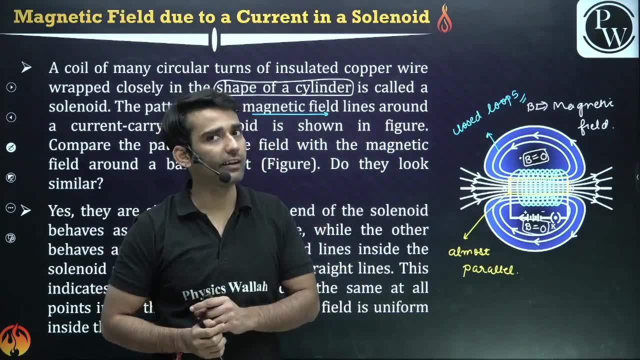 at this point magnetic field is zero here also here also magnetic field is zero so outside solenoid we have a very very weak magnetic field but inside we have uniform and stronger magnetic field 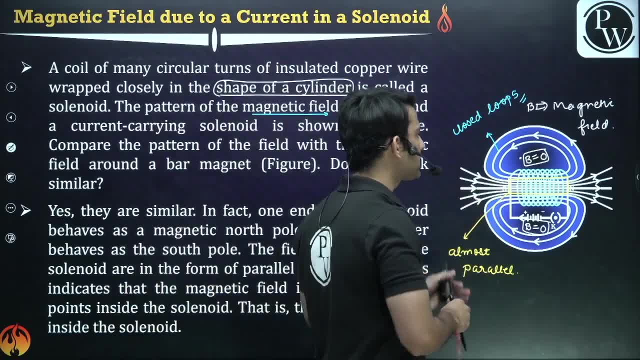 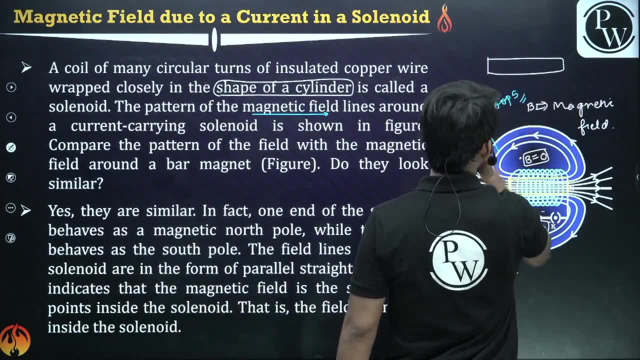 where does where will it be maximum near the poles can you see it guys isn't it resembles you of the bar magnet right what is the pattern of field of bar magnet this kind of resembles it 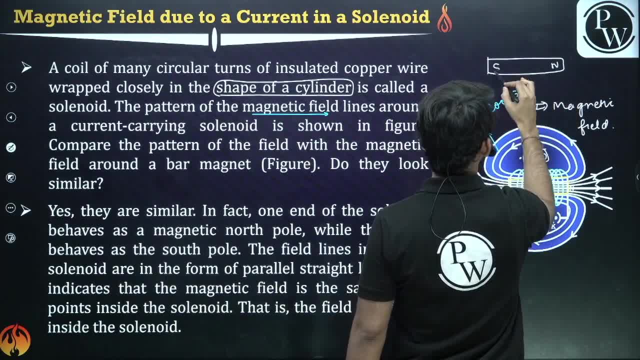 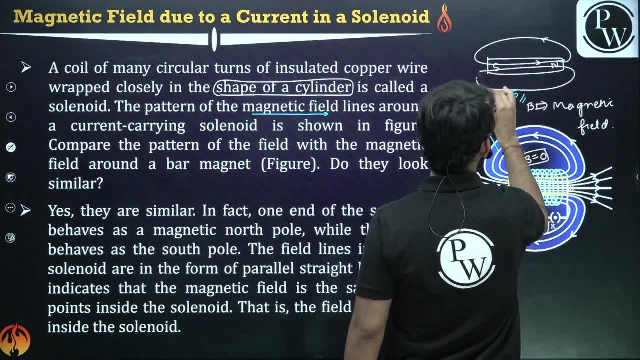 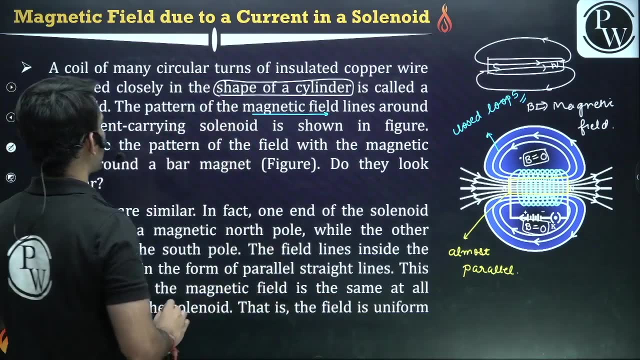 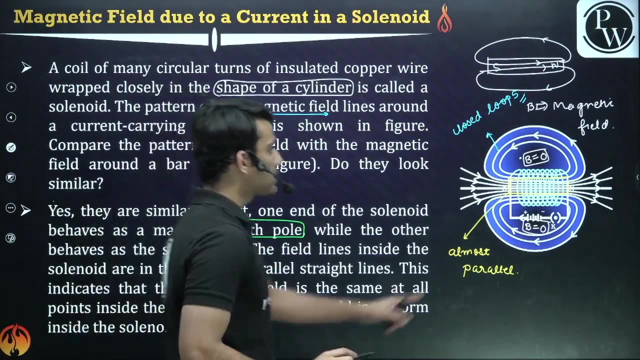 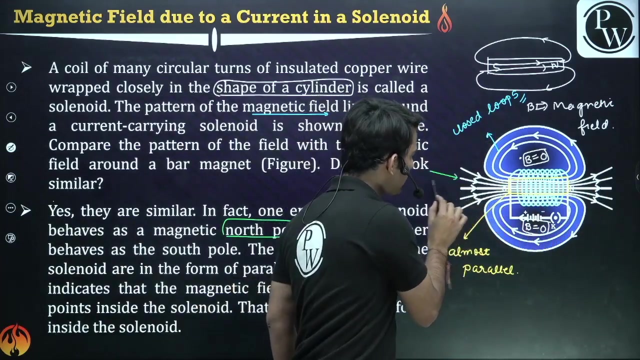 let's say uh this is north this is south so guys the pattern kinds of resembles that of bar magnet right it kinds of resembles that of bar magnet okay pattern for both is same so can you compare the pattern of field with bar magnet you will find they are similar one end of the solenoid acts as a magnetic north pole you can see from this pole of the solenoid the magnetic field is emerging so this is north pole and at this point the field is terminating it is entering into the magnet or the solenoid so this is south 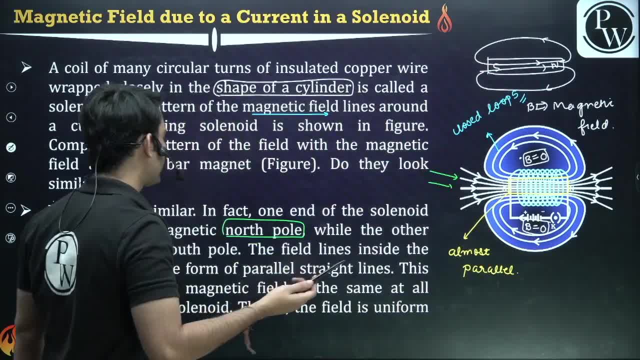 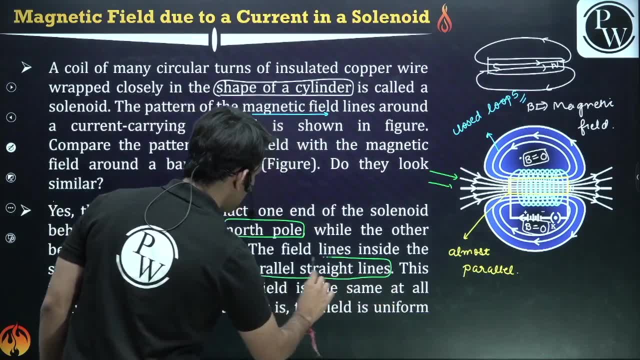 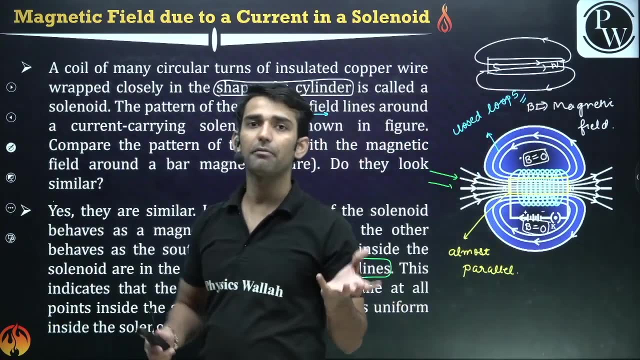 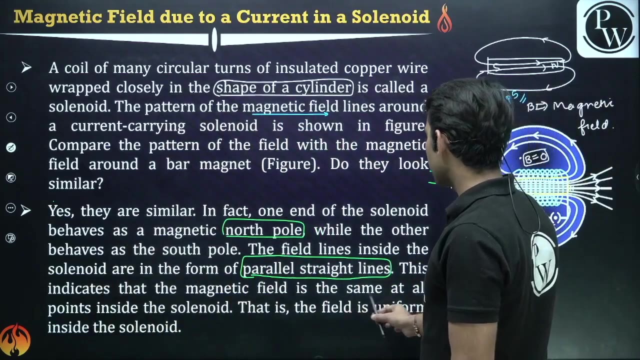 s same here right so pattern is kind of same the other behaves the south pole the field lines inside solenoid are in the form of parallel straight line this question is asked guys in most of the exams what is the pattern of the magnetic field inside the field lines on what do you how do you tell me uh tell the pattern of magnetic field are they uniform or the non-uniform inside the solenoid the answer would be yes this indicates magnetic field is same at all the points in the 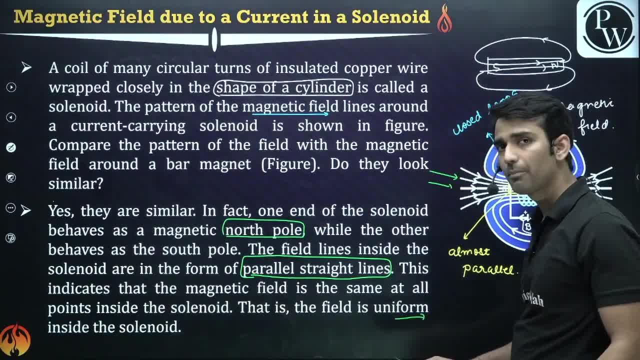 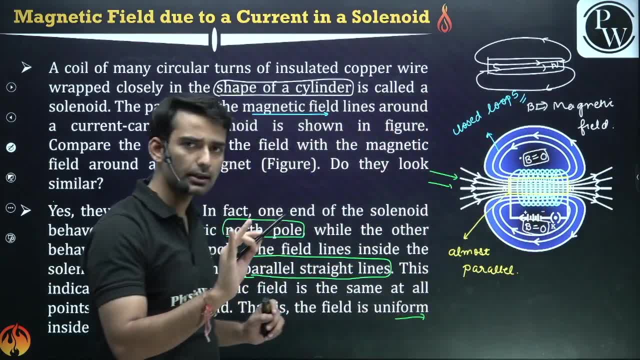 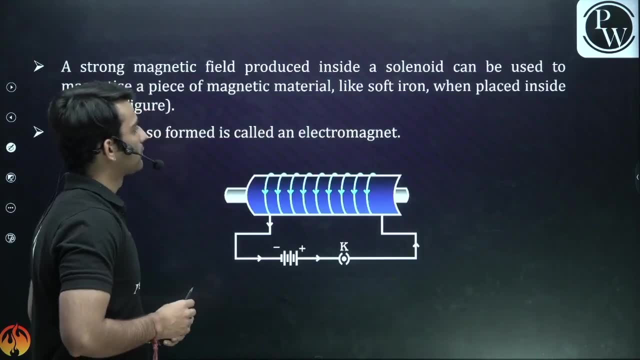 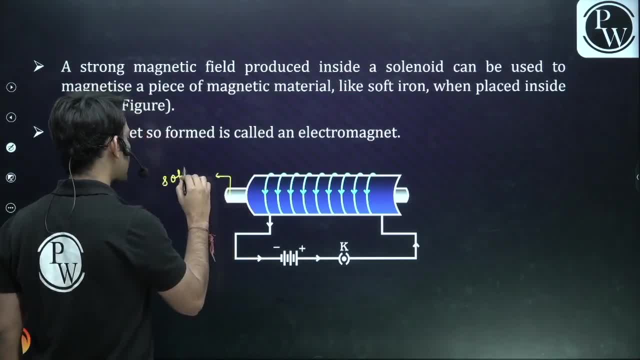 on a soft iron core see guys iron is a magnetic material right basically if you place what happens 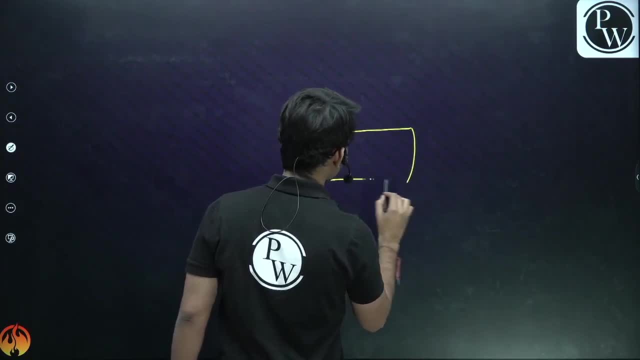 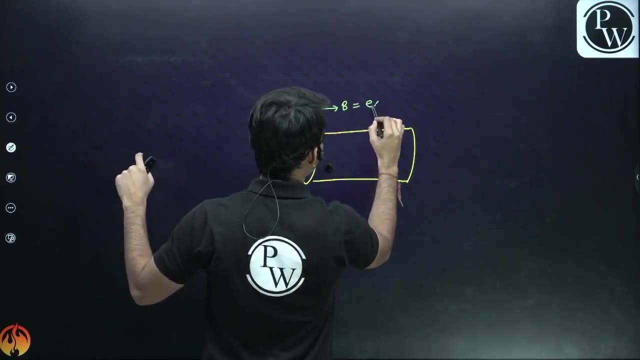 is let me tell you see basically if you place any iron rod or iron in some external magnetic field this b is the external magnetic field external magnetic 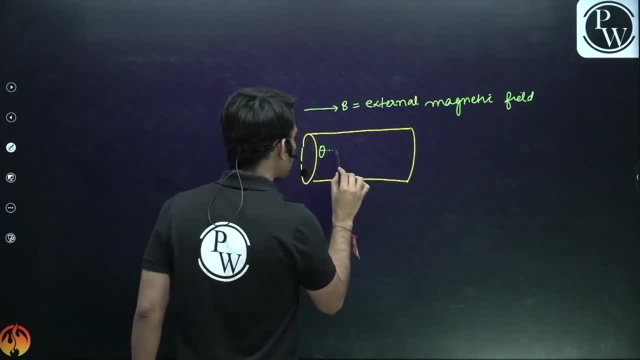 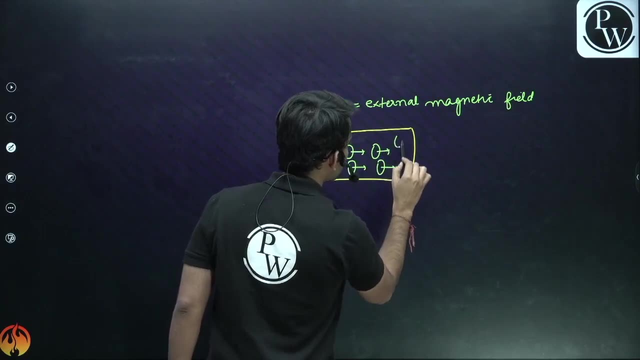 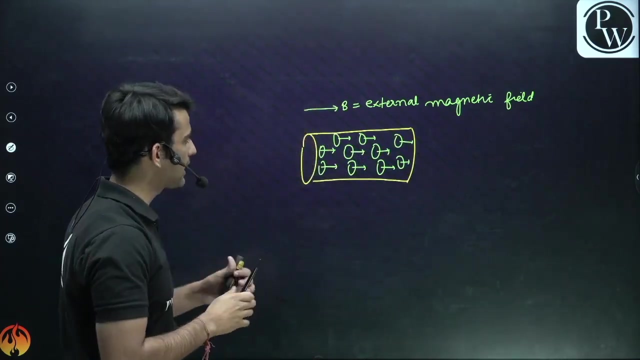 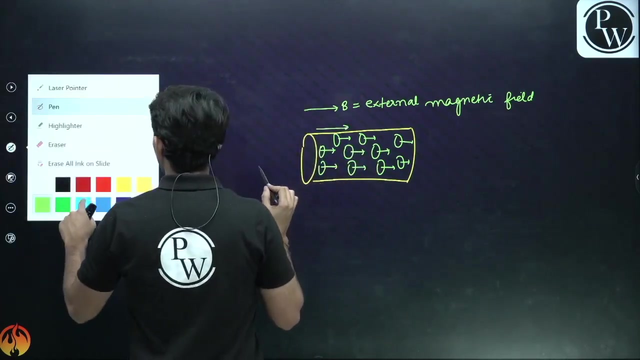 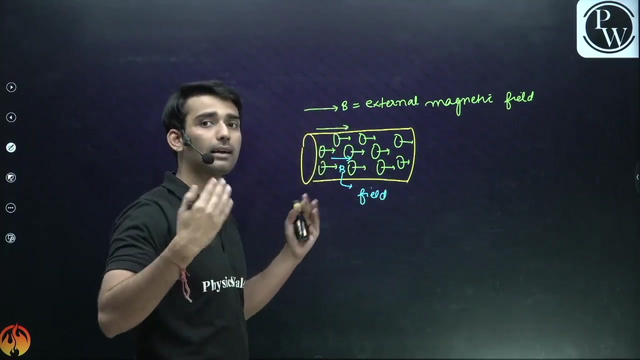 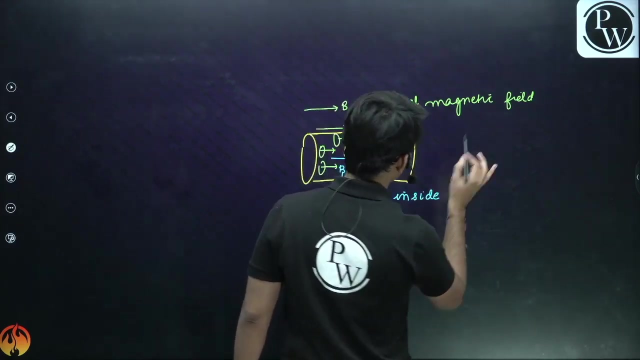 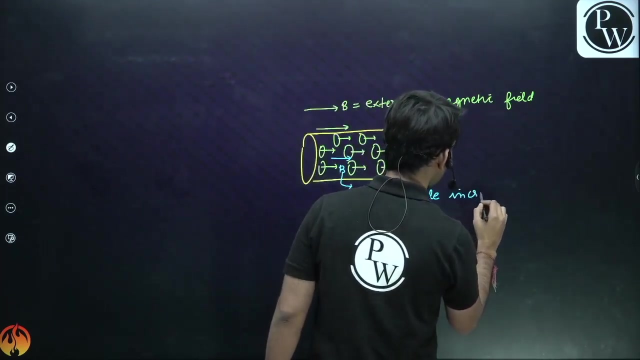 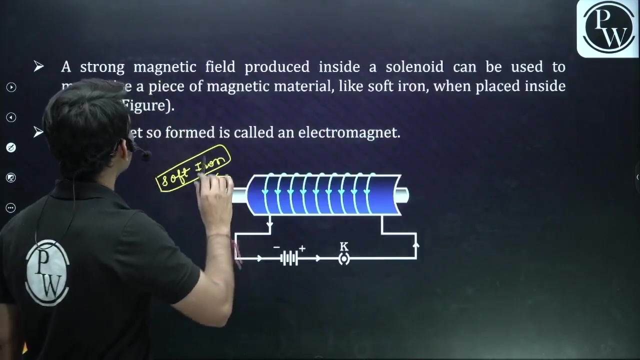 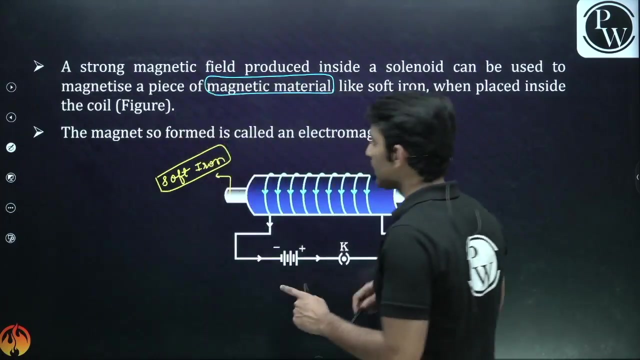 field so guys what would it do it basically magnetizes these are the small dipoles every iron has some dipoles so basically this field aligns the dipole all these dipoles in the same direction dipoles means and they basically we have two poles positive and negative so all the dipoles align themselves in the same direction therefore magnetic field inside increases field inside iron core increases or it magnetizes now it will become a magnet it will become a magnet so basically if you want to increase the field inside just put the put wrap the solenoid on a soft iron core because field inside increases because iron is a magnetic material it shows its strong magnetic nature when it is put ... kept in the magnetic field so strong magnetic field can produce inside solenoid can be used to magnetize a piece of magnetic material now if you want to magnetize any material because we have a strong field inside the solenoid if you want to magnetize a material 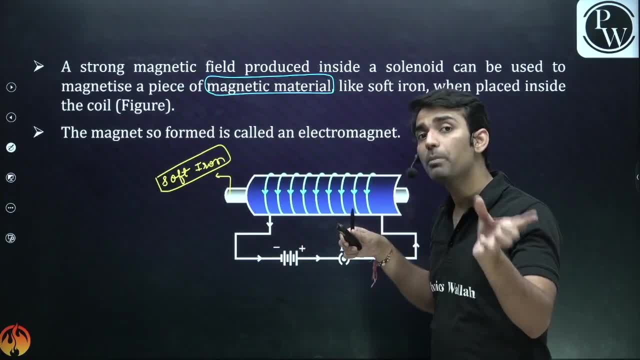 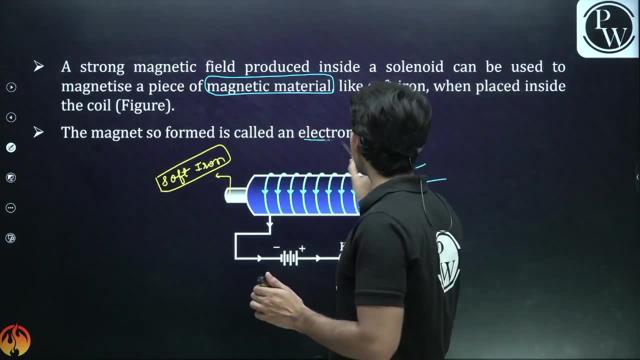 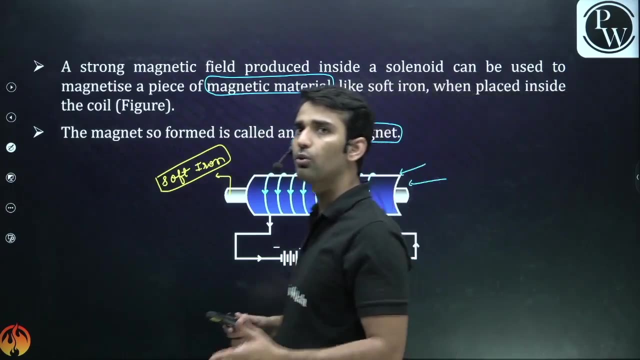 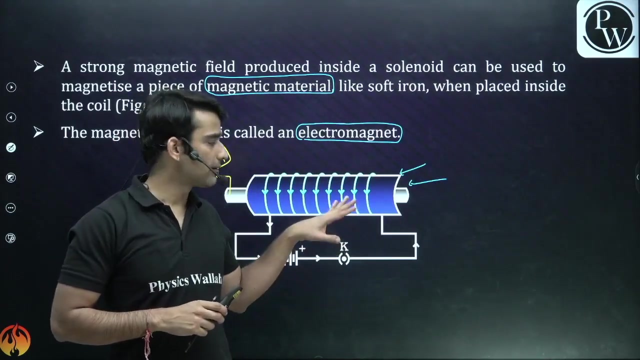 just put it in a solenoid that material will now behave as a magnet and it will attract the iron fillings or iron material this magnet is called electromagnet we have we use this in the cranes in the scrap yards yeah right so now right now we use these electromagnets right which is just switch on the current it will work as a magnet because we have current switch off the current right it will lose its magnetic ability so it's in it's a basically it's artificial magnet you can call it 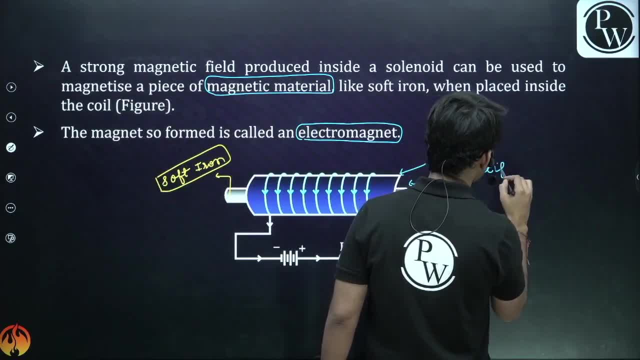 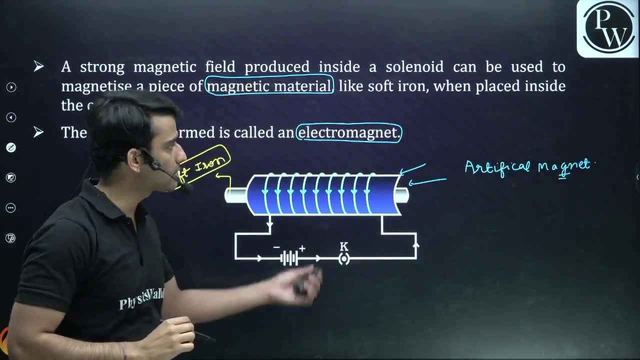 electromagnet is nothing but artificial or man-made magnet artificial magnet you can call it electromagnet right or magnet magnet it depends on the current the field due to electromagnet it 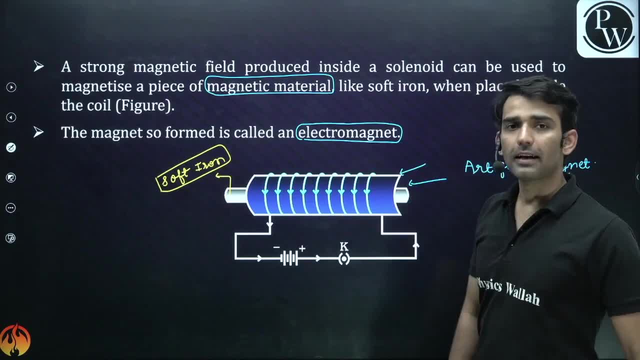 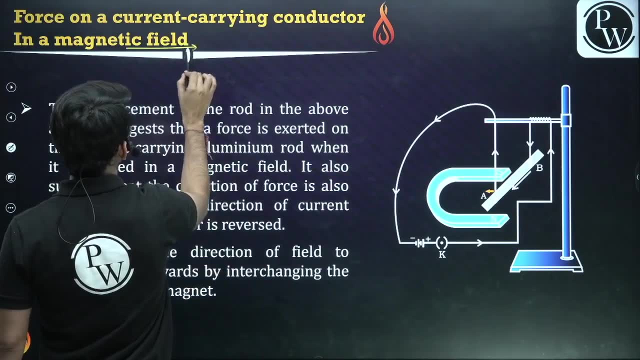 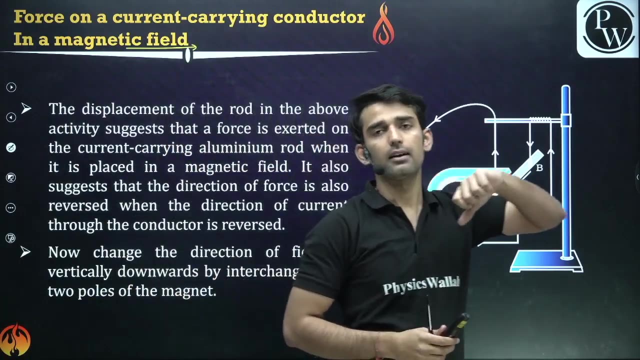 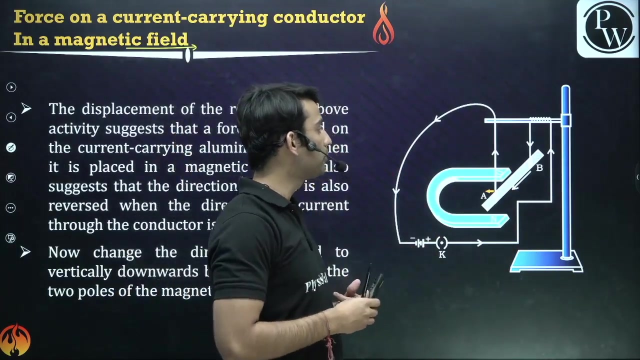 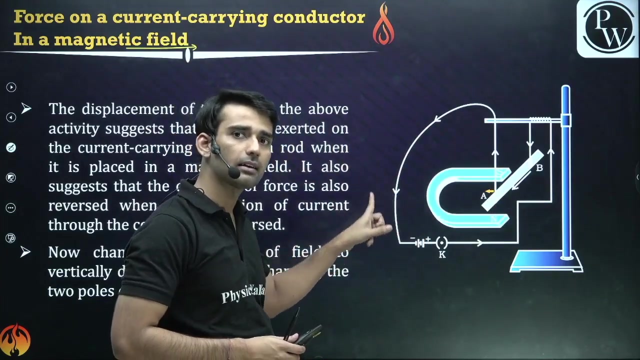 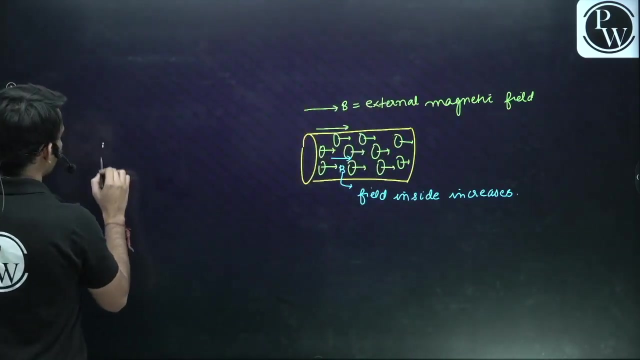 basically depends on the direction of the current clear okay now next is how can we observe the force on a current carrying conductor in magnetic field now thing is i had told you when you put the compass needle in current carrying wire near the current carrying wire the compass needle had experienced some magnetic force because of the field of the wire now question is if you place any current carrying wire in external field any current carrying wire in external field will it experience some force so the answer is yes guys answer is yes see what happens is suppose we have some amount of current in the wire let's say electrons are moving electrons are moving like this right guys so what is the direction of the 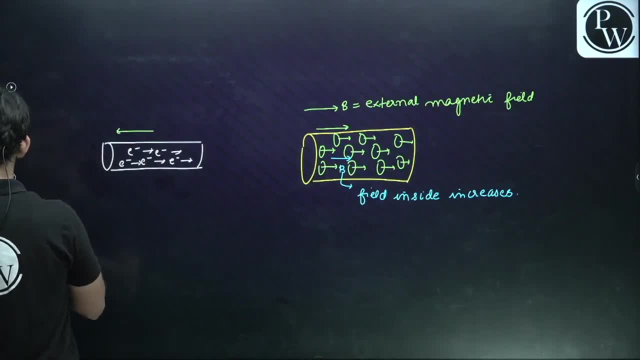 current the current direction of the current would be like this the direction of the current would be like this okay guys so guys if you place any current carrying wire in external field will it experience 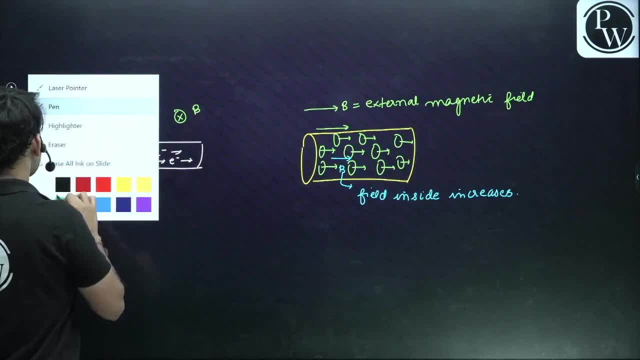 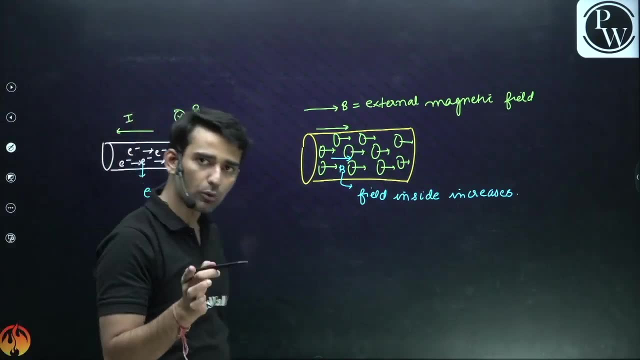 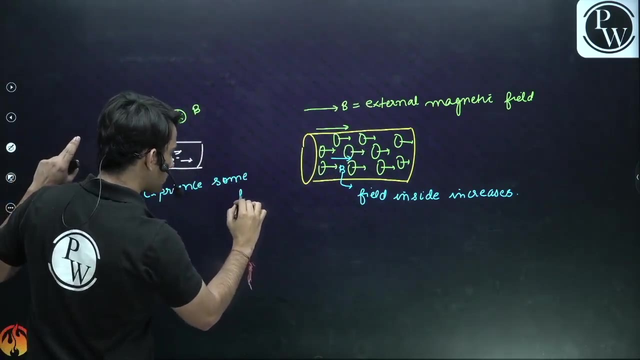 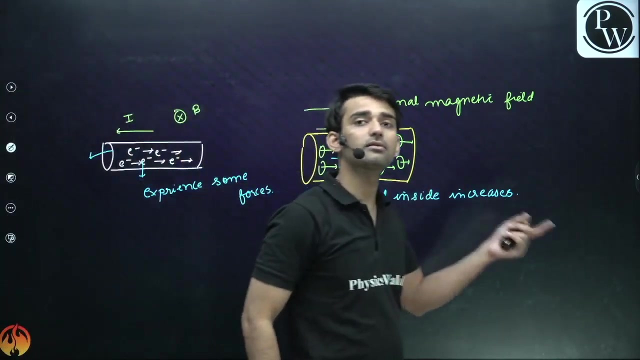 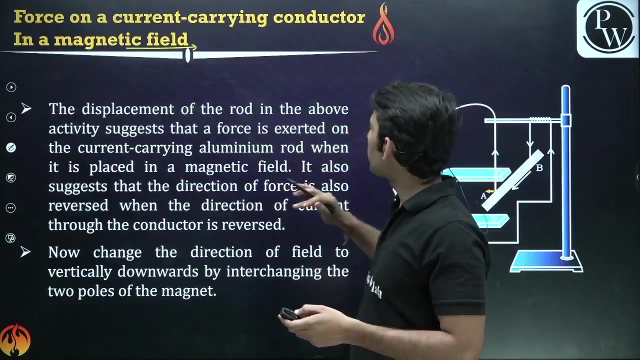 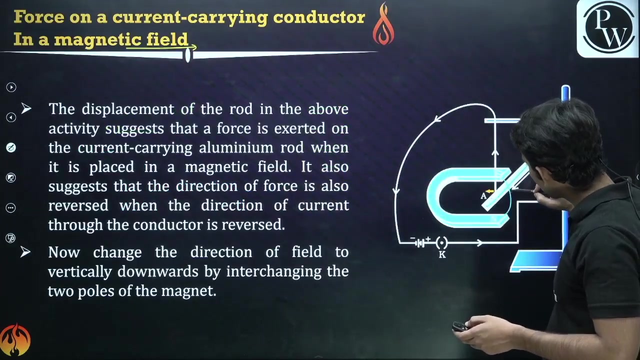 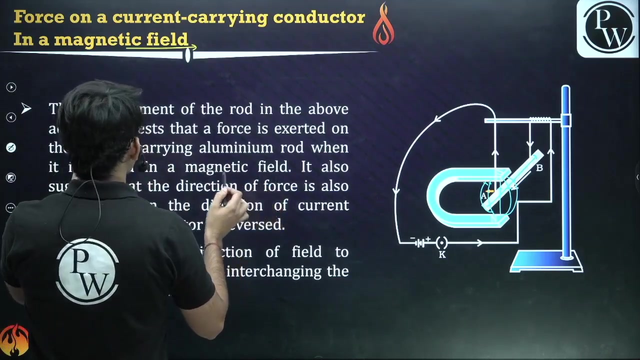 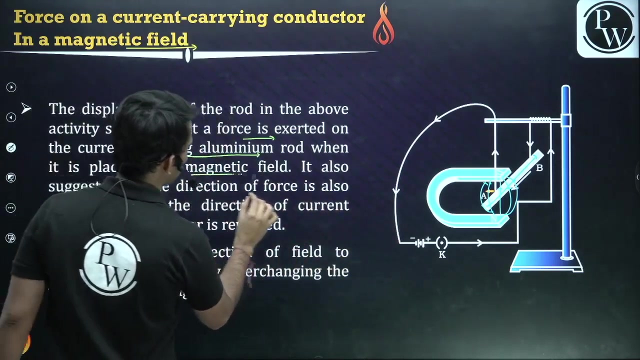 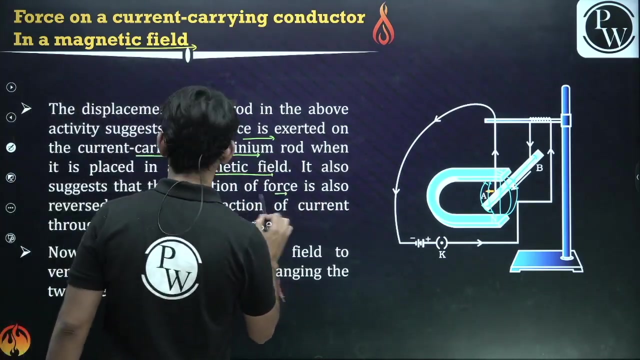 some force so if you place any current carrying wire in external field what is this wire is in external magnetic field these electrons will experience some force because whenever there is a moving charge in magnetic field that moving charge experiences some force so all these electrons will experience some force so the force will be added up all the force will be added up and as a result this wire will of experience some force in the magnetic field right because it has moving charges inside it right so that means if you place any current carrying wire in external magnetic field we have horseshoe magnet here and for horseshoe magnet the magnetic field pattern would kind of look like this it kind of look like this so if you place this current carrying wire here the wire will experience some field right you can perform this activity now it would suggest that the force is exerted on current carrying wire aluminium rod we have taken when it is placed in magnetic field the wire will show some deflection aluminum is obviously a magnetic material it also suggests that direction of force is also reversed if you reverse the current you 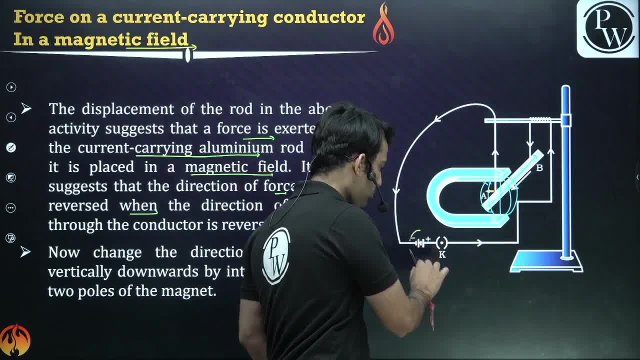 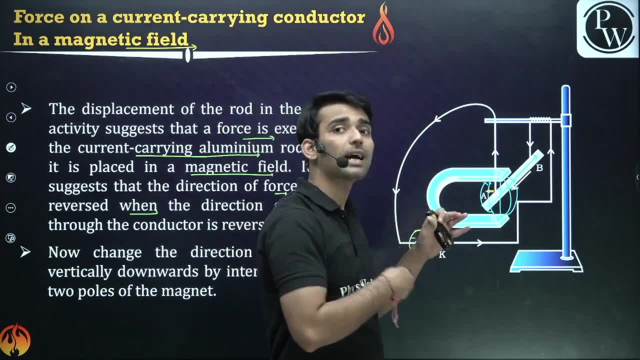 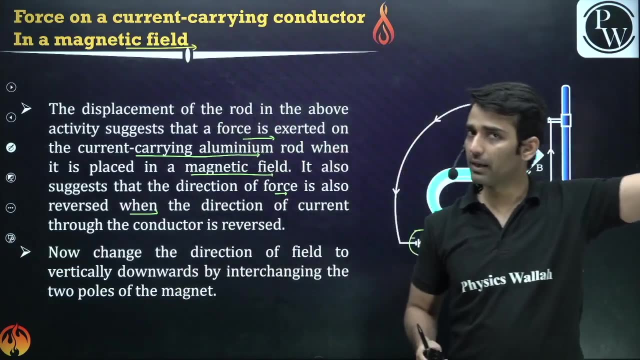 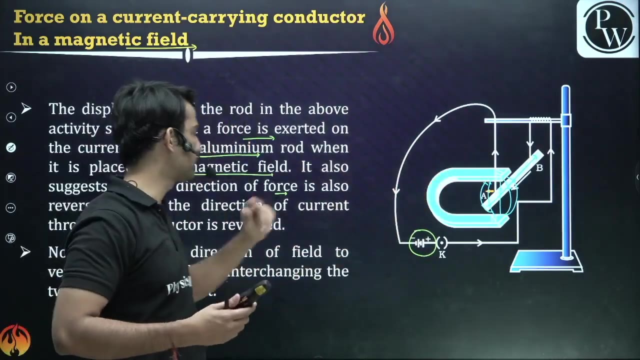 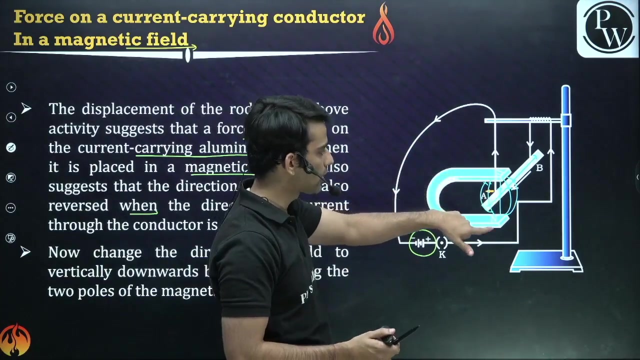 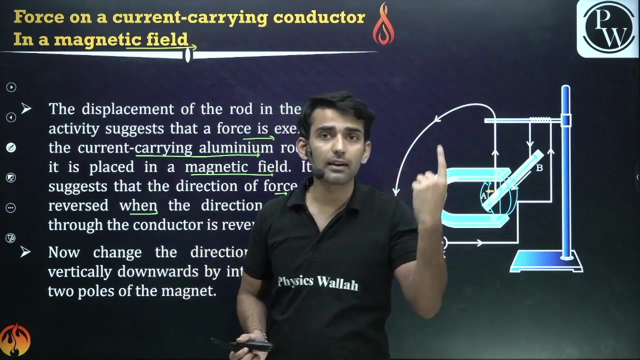 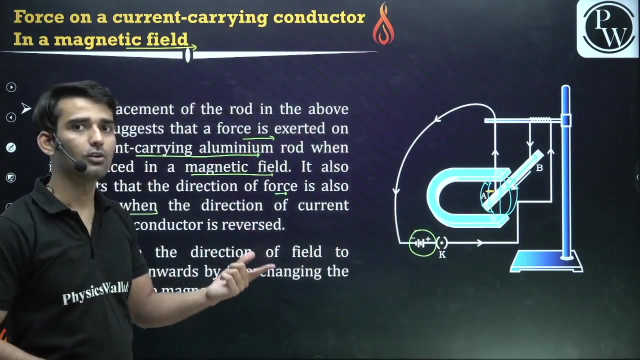 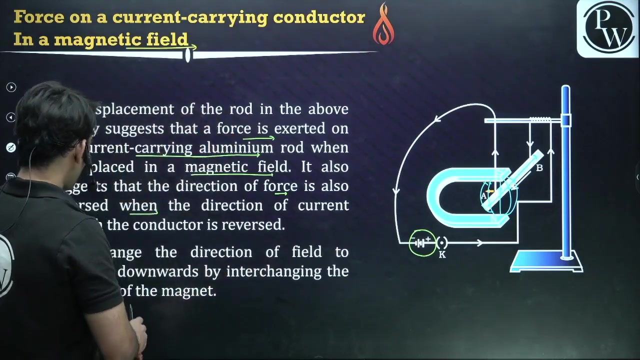 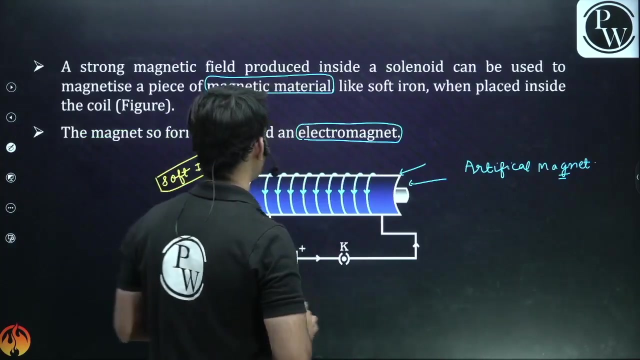 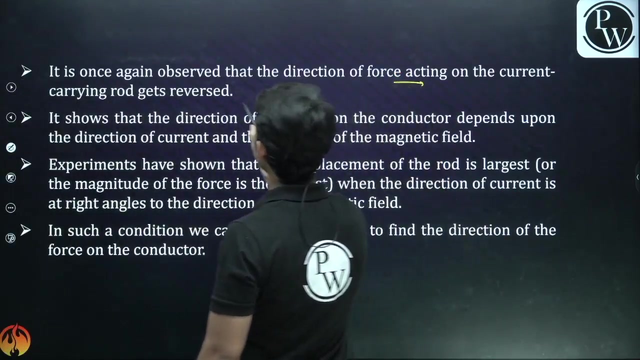 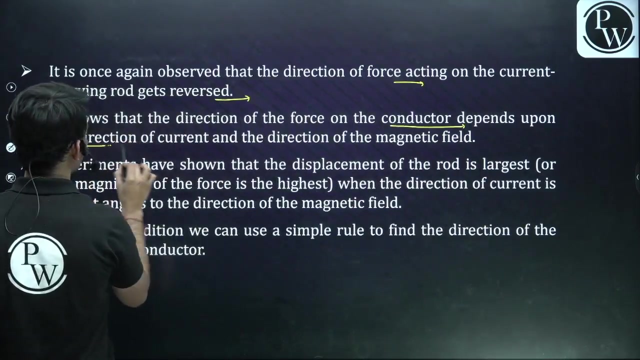 can see the current is going here like this but if you reverse the polarity of the battery the direction of the magnetic field or the current would be reversed so that means the diffraction would be reversed because now the force is also reversed so if you reverse the direction magnetic full field would be reversed if you reverse the magnetic field the direction of force on this wire would be reversed this has been observed experimentally now if you change the direction of the field also that means you have inverted the horseshoe magnet north upwards and south downwards so that in that case also the force would be reversed so if you reverse the magnetic field or external magnetic field also the direction of the force would also reverse so force depends on the external field also on the direction of the current inside the wire right so the if you interchange the pole the direction of the magnetic field would also be in would also be reversed so guys what can you conclude from this you can conclude that the direction of force would be reversed if you uh if the current is reversed it shows that direction of force depends on what factors the force force depends on the current right guys force depends on the current and on the external magnetic field the 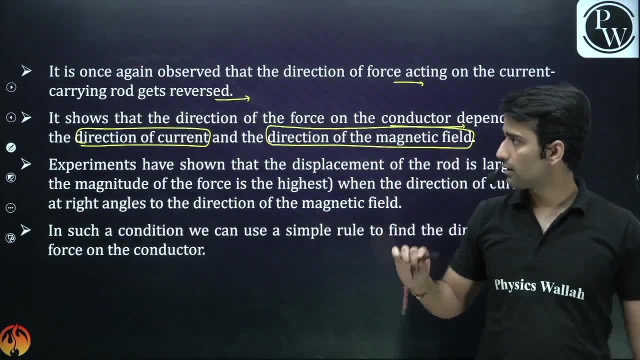 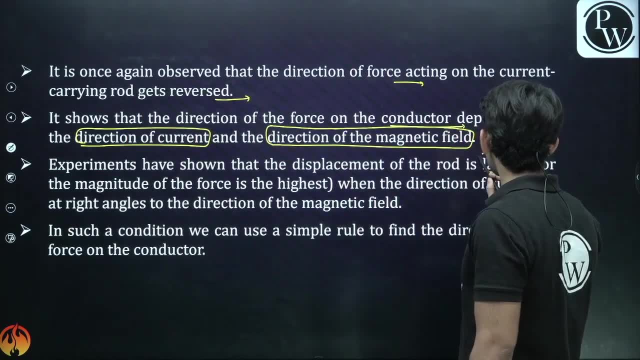 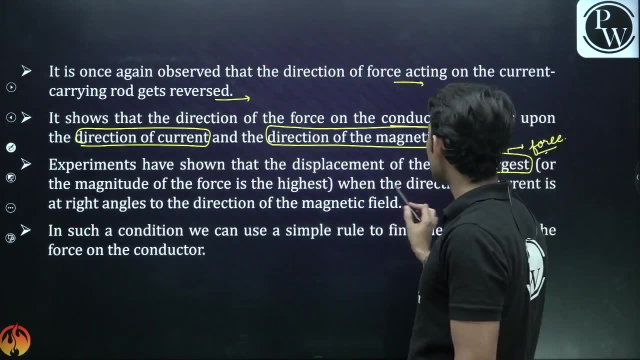 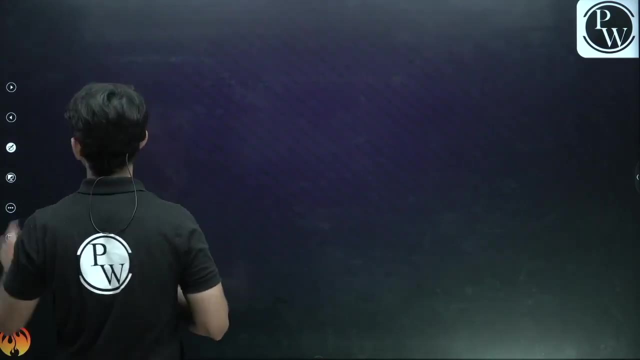 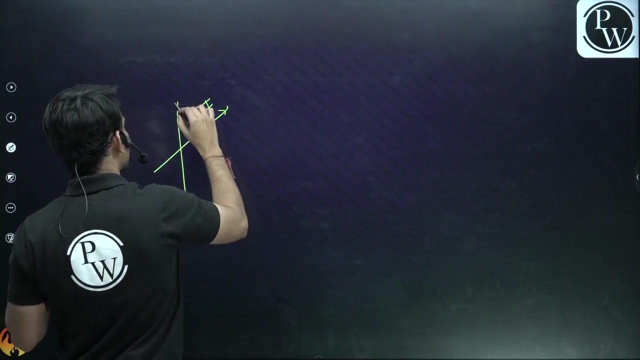 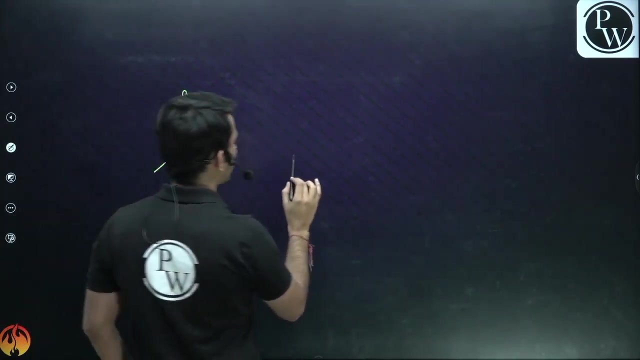 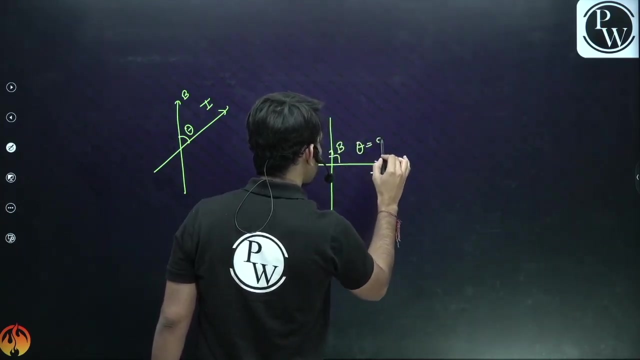 force on any current carrying wire it depends on the current and the magnetic field external magnetic field right so basically when will the force will be largest there will be a situation when the force on the wire will be largest when is that when the current is perpendicular to the magnetic field let me tell you what is the meaning of this suppose wire is like this right and magnetic field is like this the magnetic field is not perpendicular to current this angle is theta this is not obviously 90 degree but let's say current is like this and wire is like this here magnetic field and current or the wire are at 90 degree 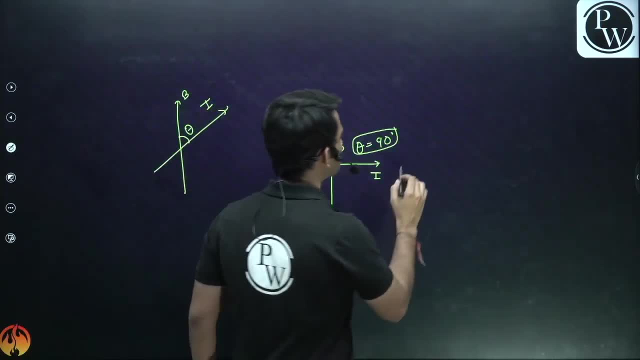 so guys in this case force experienced would be maximum in this case force experienced 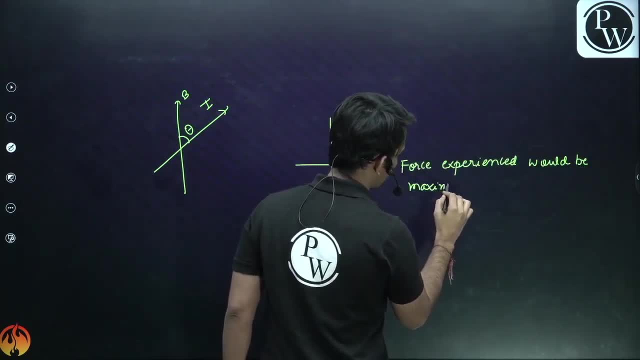 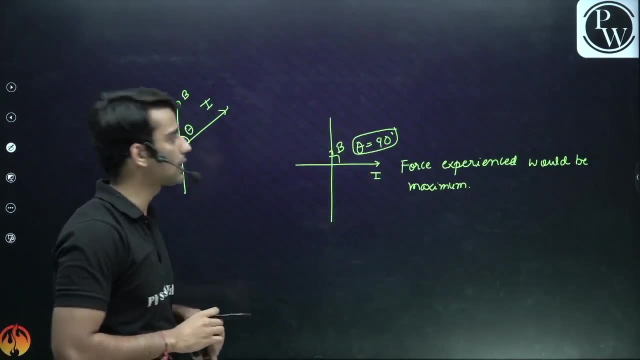 would be maximum force experienced on the wire would be maximum when magnetic field and the current are perpendicular to each other when both are perpendicular to each other okay guys so 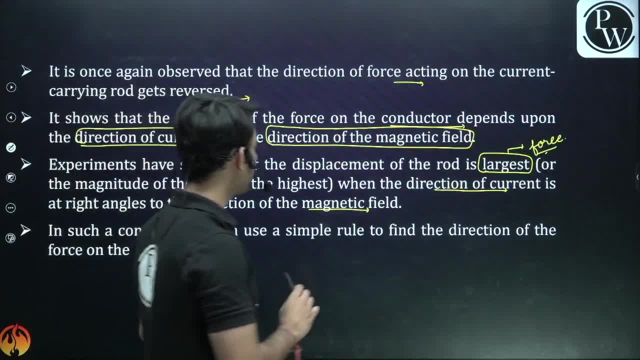 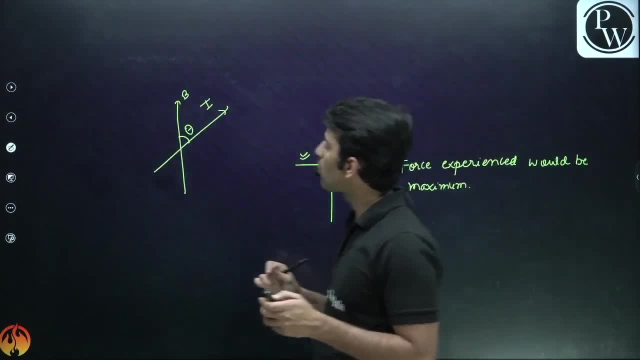 thing is uh in such a condition we use simple now question is how can we find the direction of the force obviously we have to find the direction of the force but to find the direction of the force can cannot see it so we have a rule for that known as fleming's left hand rule we have a rule for 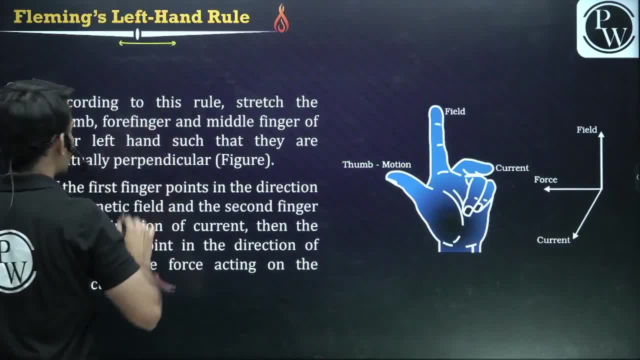 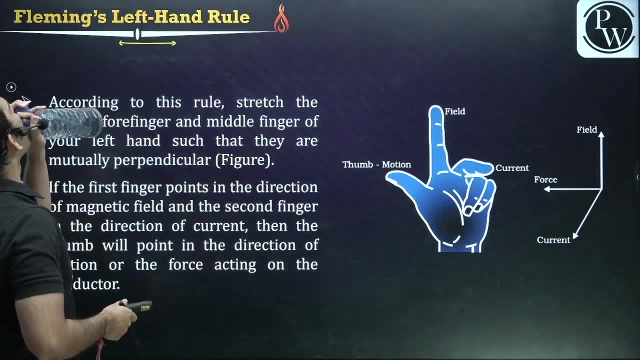 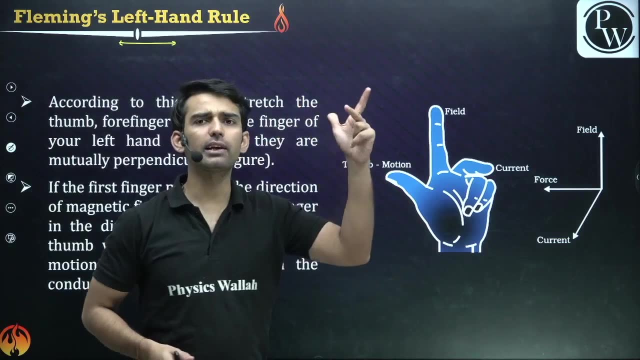 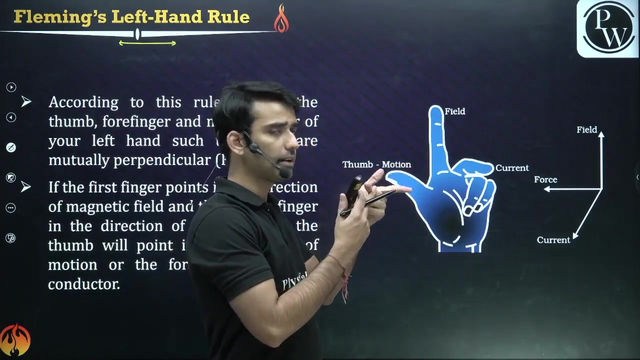 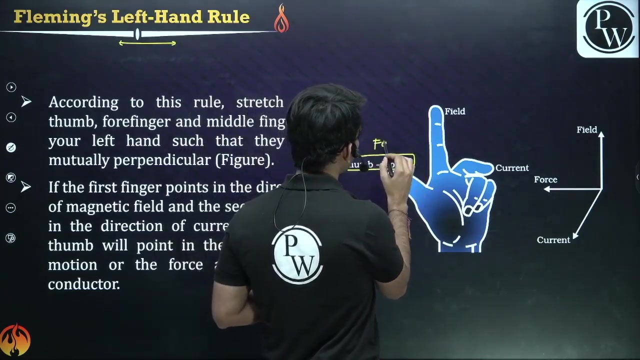 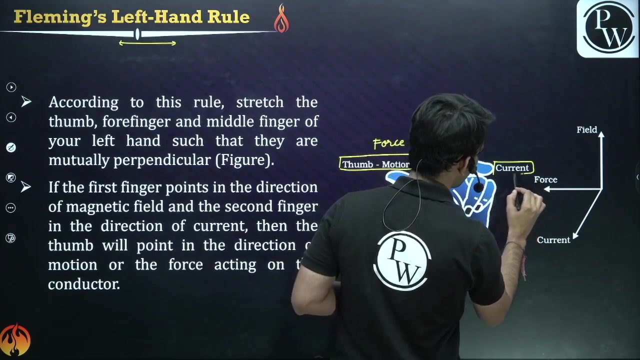 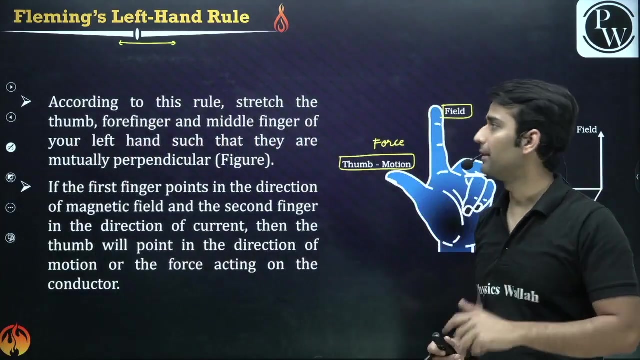 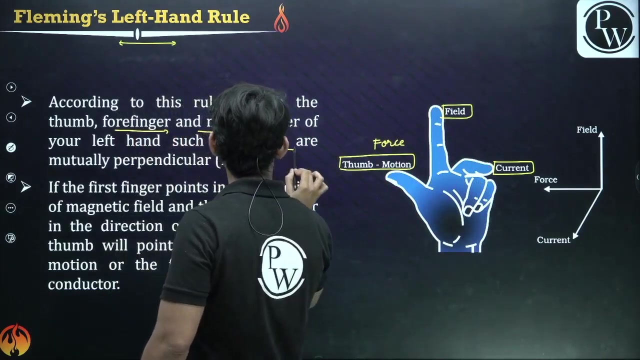 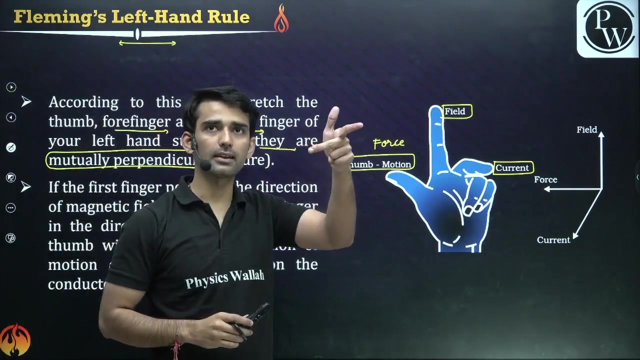 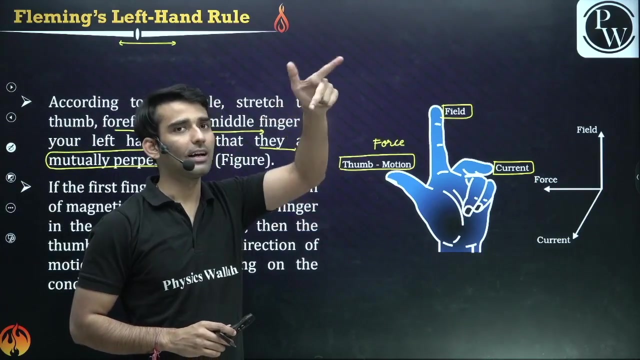 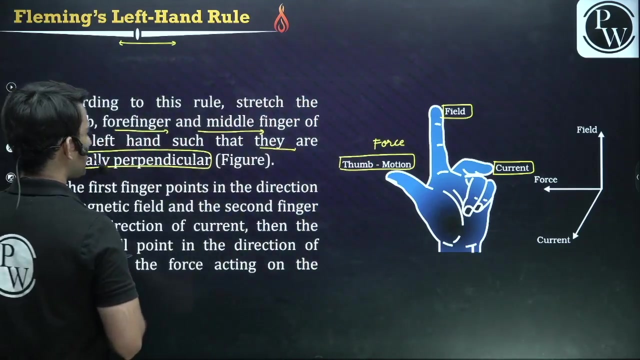 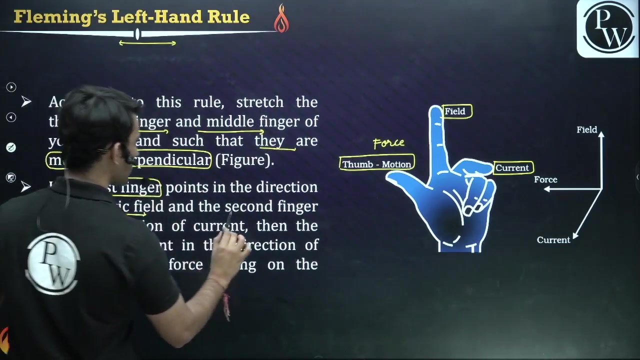 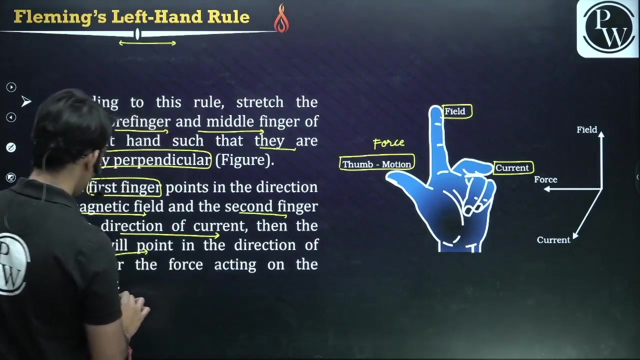 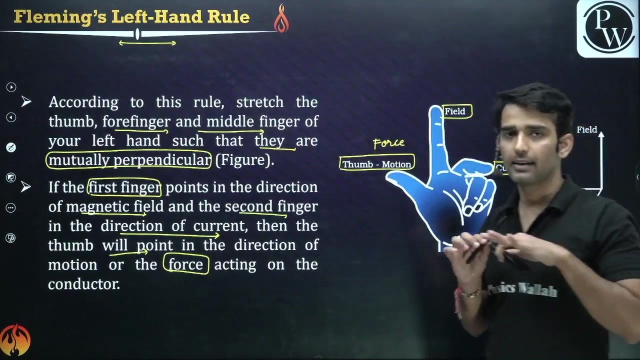 that known as fleming's left hand rule what does this rule state just read it out what does this rule states this rule states that if you take your left hand right if you take your left hand and just take your thumb your middle finger and your forefinger so guys your thumb will point in the direction of force direction of motion means direction of force middle finger your forefinger will point in the direction of magnetic field middle finger would point in the direction of the current just use all your left hand to find the direction of the magnetic field so according to this rule if you stress the thumb forefinger and the middle finger of your left hand such that they are perpendicular mutually perpendicular all the forefinger the middle finger should be mutually perpendicular like this like this it's not like you can put the forefinger like this or you can put the thumb like this no you cannot do like this it all three should be perpendicular light like x y and z axis okay so that means in the in such a case the uh first finger the forefinger would point in the direction of the magnetic field second finger or the middle finger would point in the direction of the current and thumb will point in the direction of the force this is fleming's left hand rule to find the direction of the force on any current carrying conductor placed in a magnetic field here placed 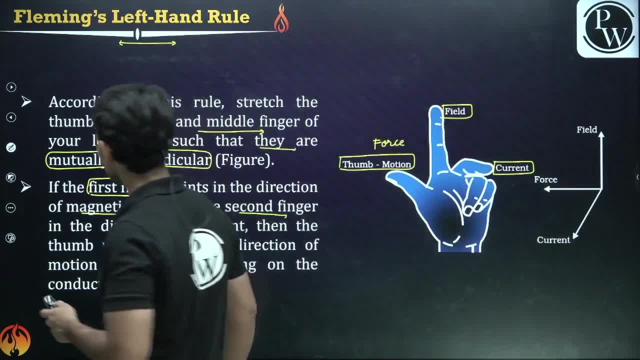 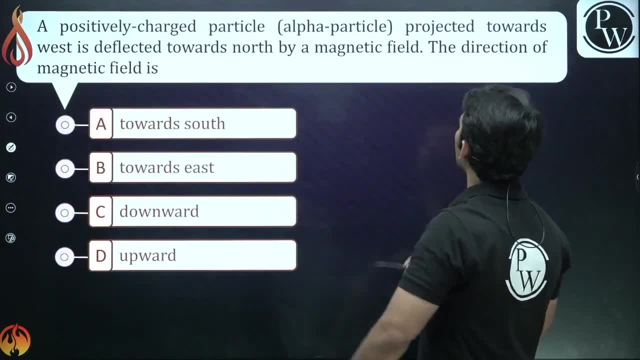 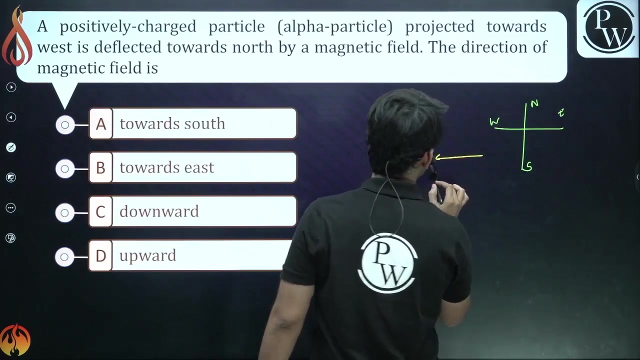 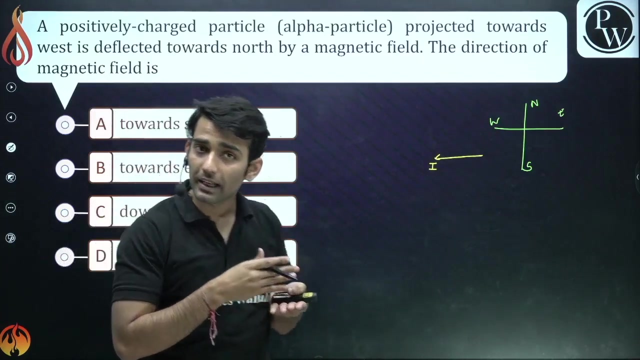 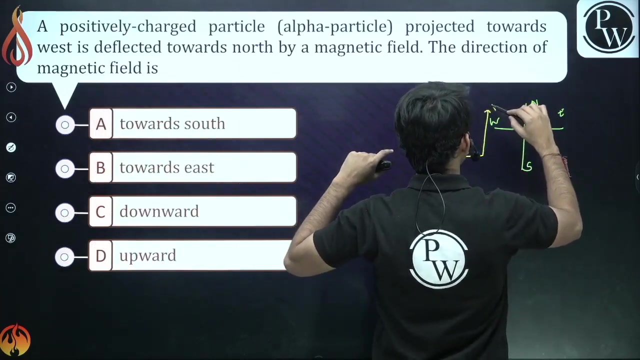 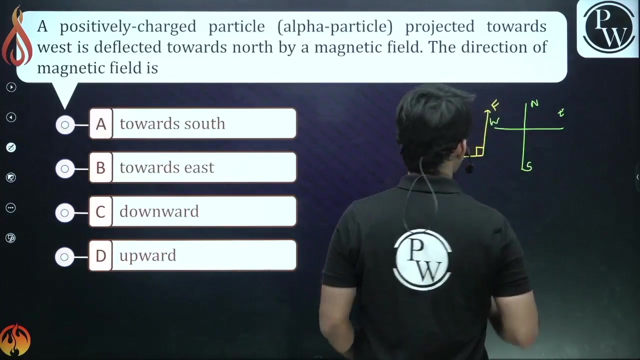 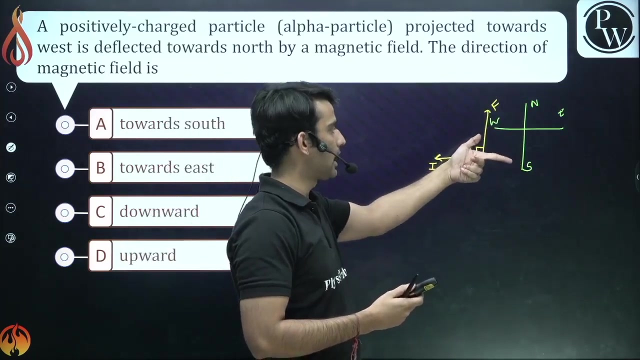 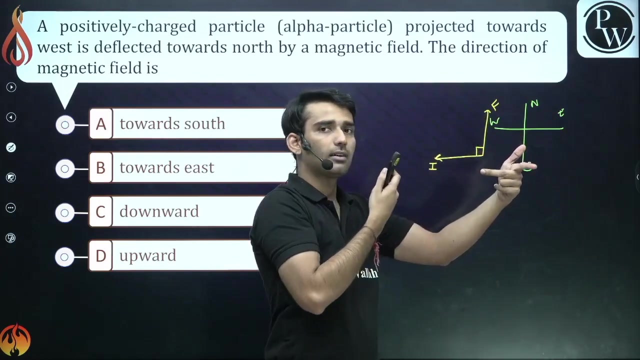 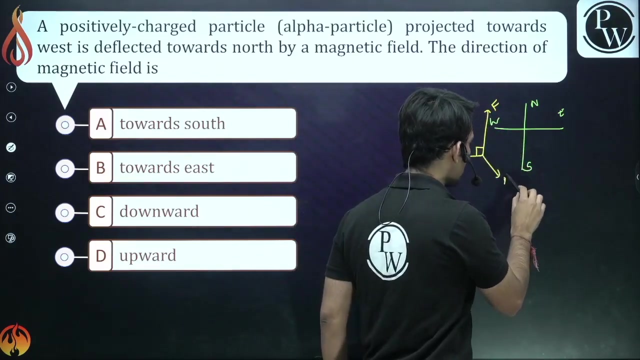 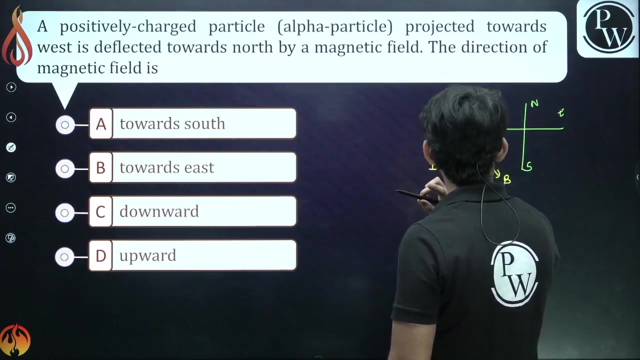 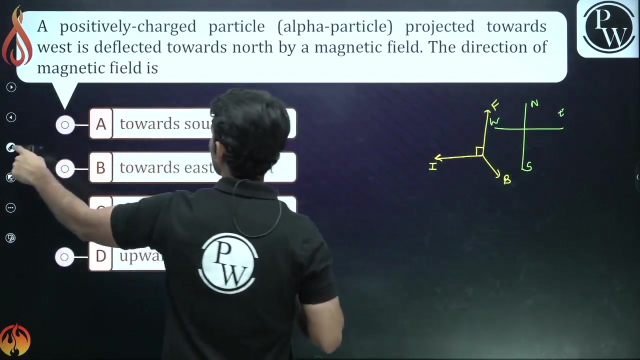 in a magnetic field fleming's left hand rule okay now let me tell you a question on how to apply this tool read the question a positively charged particle alpha particle projected towards have a direction north south west and east so alpha particle has been projected towards where towards west this is a moment of alpha part this means this is the direction of current alpha particles are positively charged particle so positively charged particle move in the direction of the current right and deflected towards north the particles are deflected towards north that means force is towards north right so you have to find the direction of magnetic field just take your left hand middle finger up middle finger here and see just thumb is upwards and middle finger is like this middle finger towards me thumb is upwards because force is towards north middle finger in west so where is the forefinger pointing out of the screen out of the screen that means magnetic field would be out of the screen which option is correct uh let's say it is 3 degrees right of square it's 3 degrees right of square whatом we did and if we took the magnitude from our weight that means количество was in our weight where is the direction of this force and it would be at the top 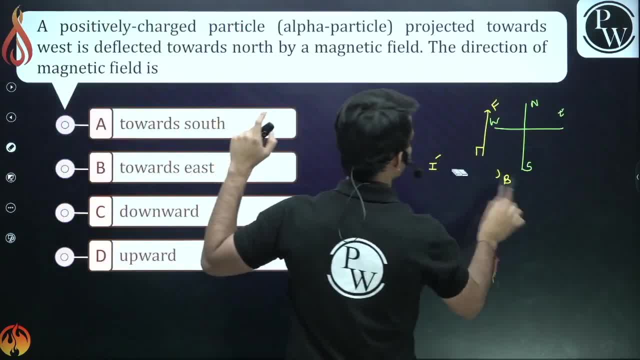 i feel like the method we have learned at least may be at a very anywhere mild degree but so basically we can use it that way just do not even think about the case but the this is to give you an example what is the direction of this force right of square it should be at this point in the fahrenheit for example 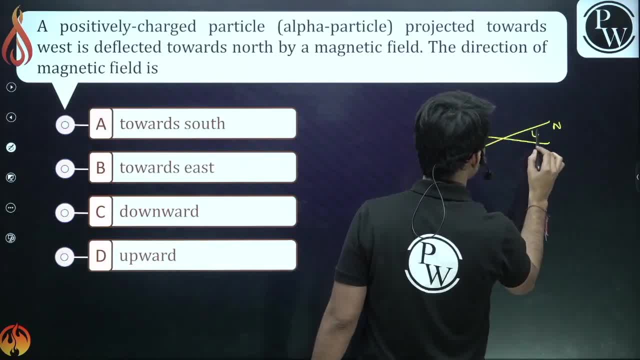 whether you are a Microbiologist you could call this a magnetic field mode of the force and you will notice you will see the direction here let me say from this side let me tell you what the direction here is in this direction here in the direction of this force let me tell you what the direction is because 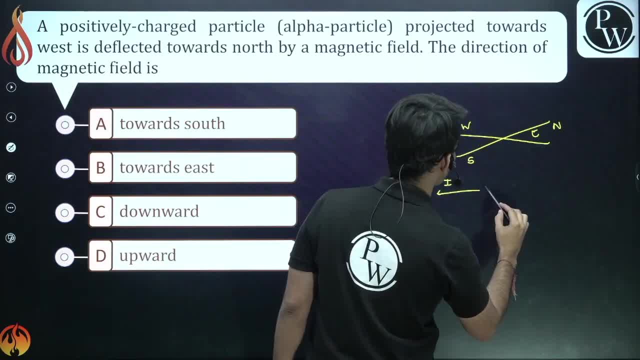 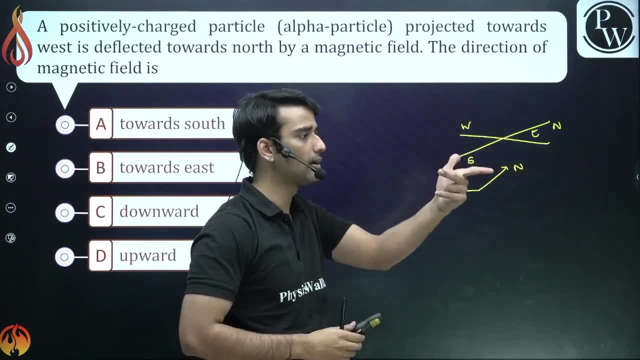 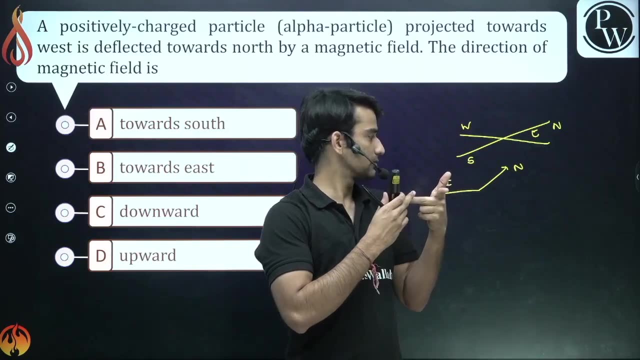 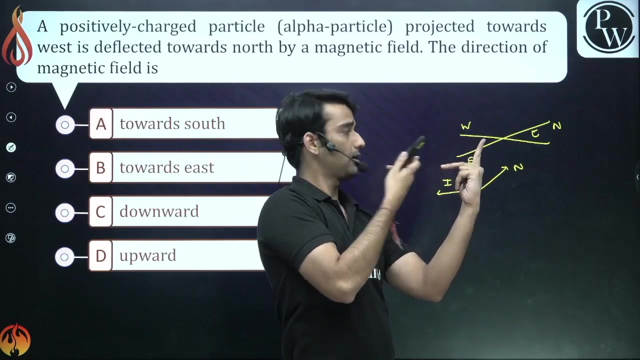 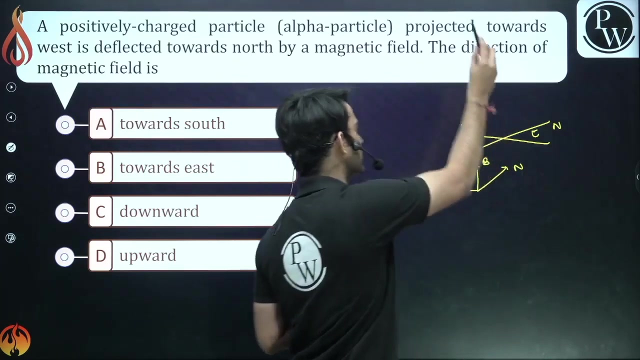 as you see it is coming from the Davini in so this part of know what to do and the force is along north right now take it's a it's in the it's it's horizontal it's in the horizontal plane so middle finger towards me thumb towards where middle finger towards me and thumb in the north right this is the north is here into the board right and the middle finger towards me so where is my forefinger pointing upwards that means magnetic field would be in the upward direction upwards so which option is correct d magnetic field will point in the 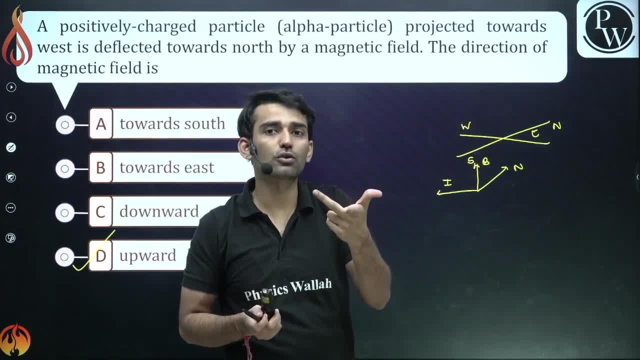 upward direction they just make the sense you should be knowing which sense you have to make 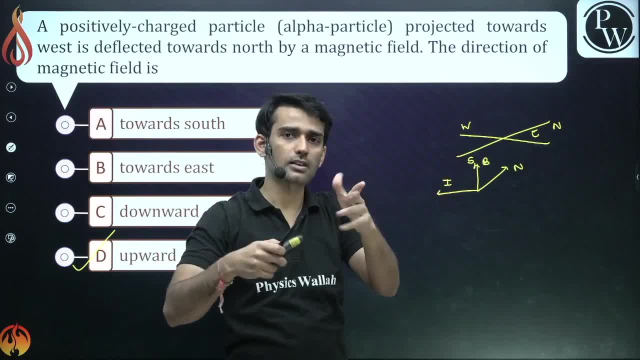 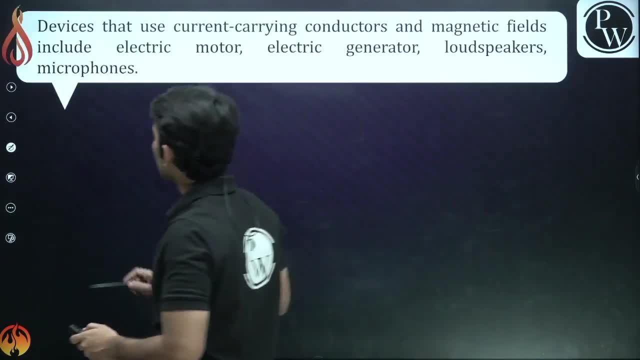 if you're dealing with the horizontal plane so take just put put your fingers like this that that they lie in the horizontal plane clear right so what are the various 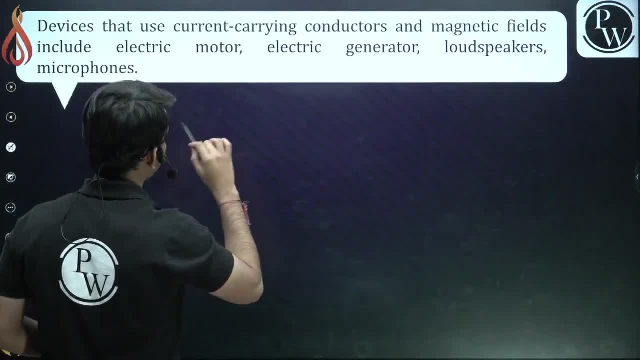 patterns that depends on what are the various devices we use on the magnetic field we have basically electric 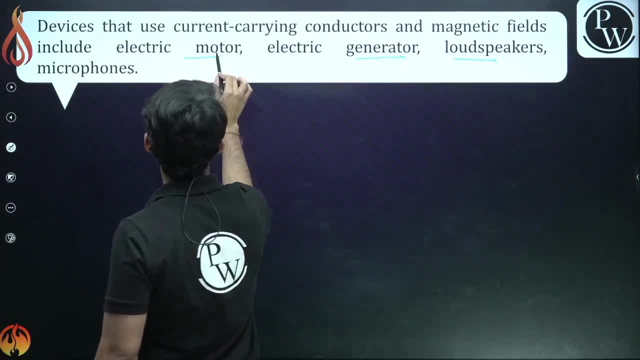 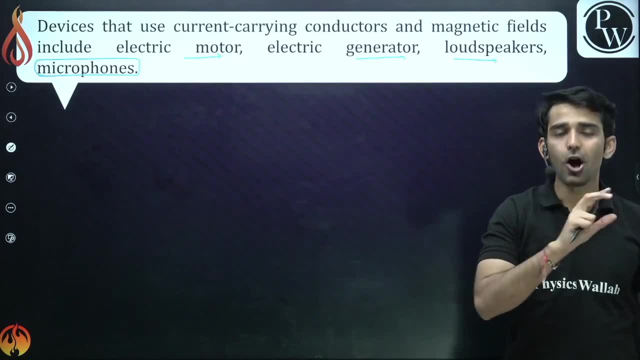 generator we have loud speakers we have electric motors we also have microphones these are based on the magnetic effect of electric current right we have magnetic effect in all these devices all 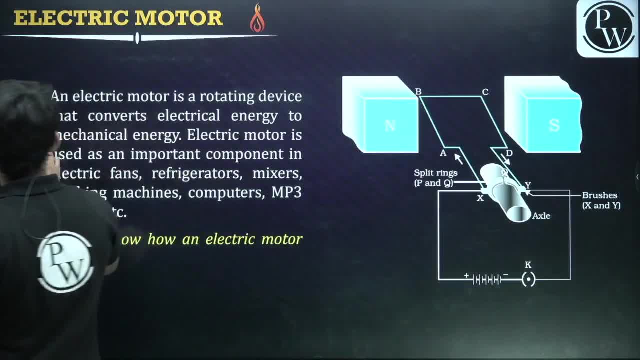 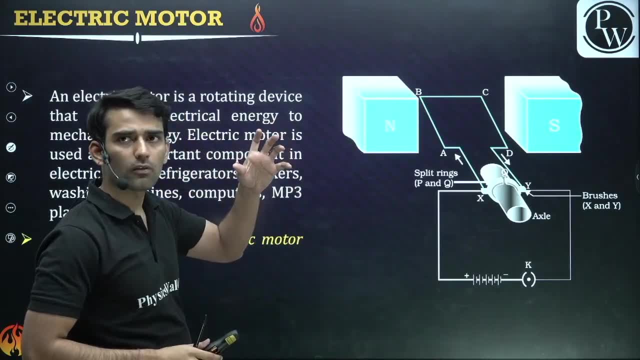 these devices now question is what is electric motor guys what is electric motor see we have motor in our fans right so that rotates whenever there is a flow of current through that the that 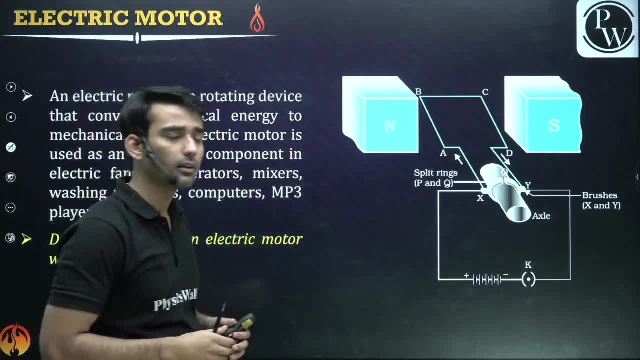 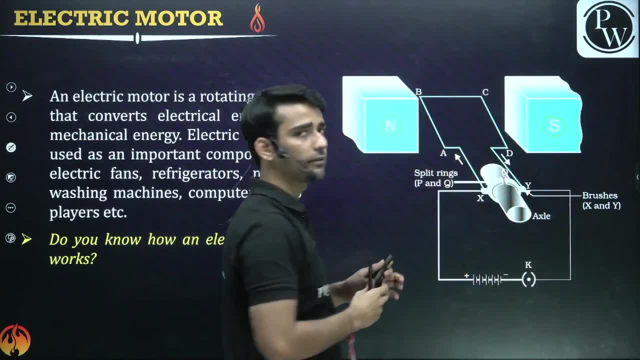 rotates whenever we have a flow of current through that now guys if you take if you have taken two magnets a north pole and a south pole you have bring you have put this 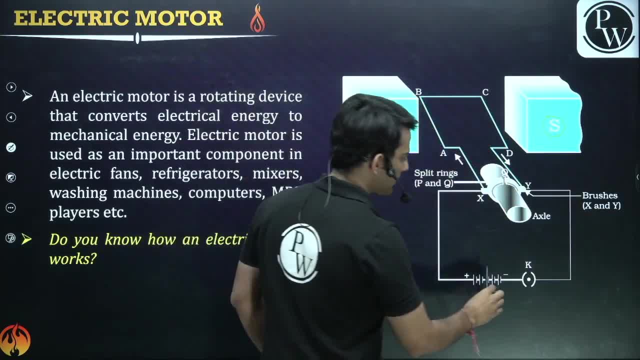 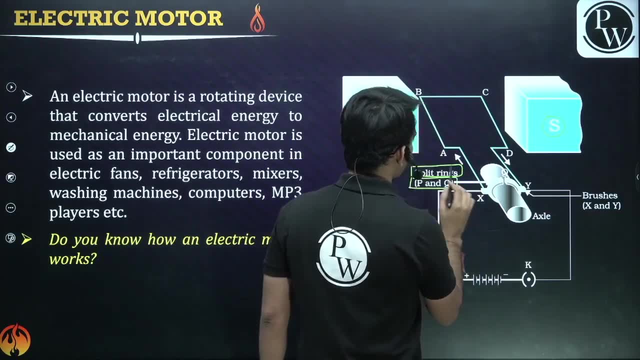 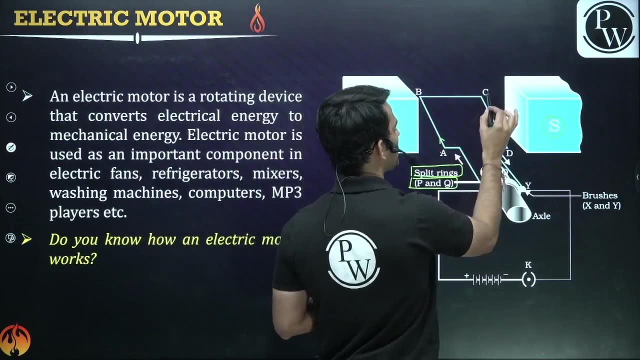 coil in between the magnets we have a current we have a key we have a battery to make the current we have split rings i will tell you the role of split rings right guys so we have a current carrying current here now guys in this part the current is from a to b here the current is from c to d 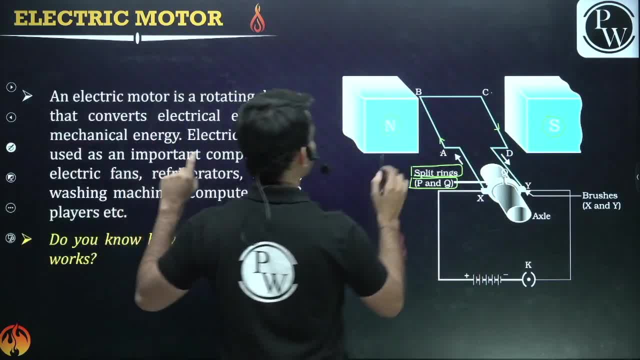 now you have to find the magnetic field direction sorry uh the direction of the force so this is the direction of the magnetic field here 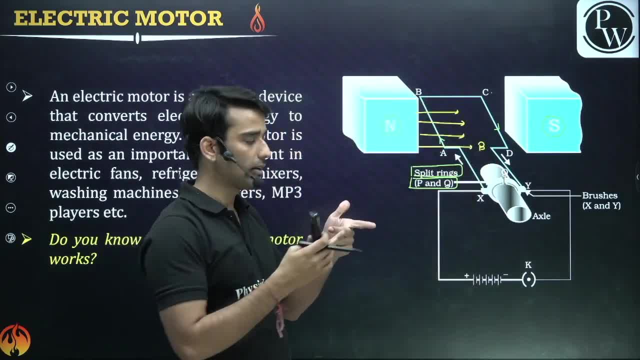 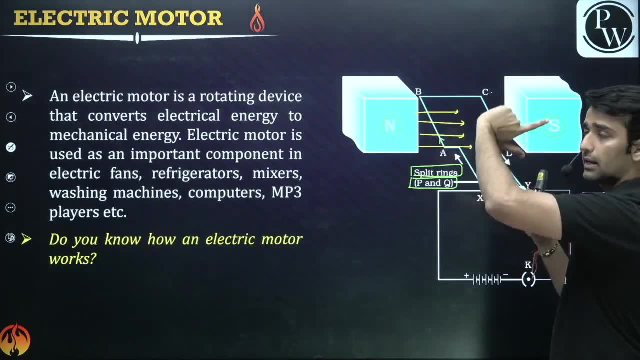 here the direction of magnetic field is this just take your left hand current into the screen and forefinger towards me so where is my thumb pointing is it pointing downward just do with me 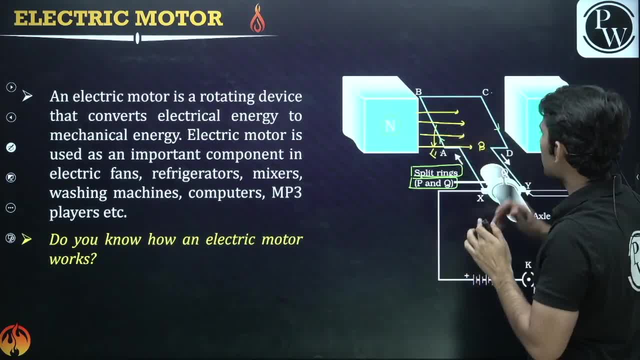 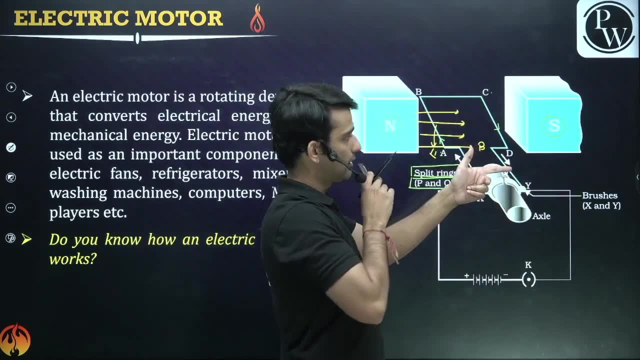 so that means this will move downwards and what about cd current is what current is out of the screen and magnetic field into the uh from left to right that means the thumb is 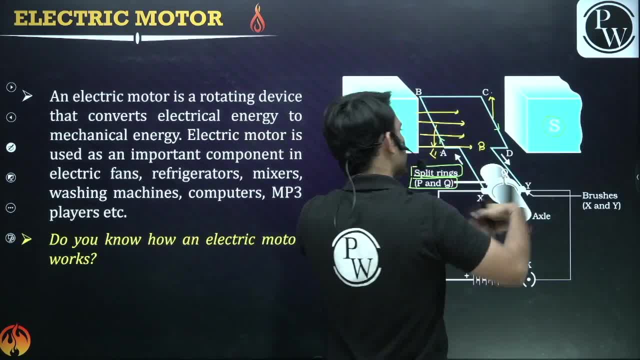 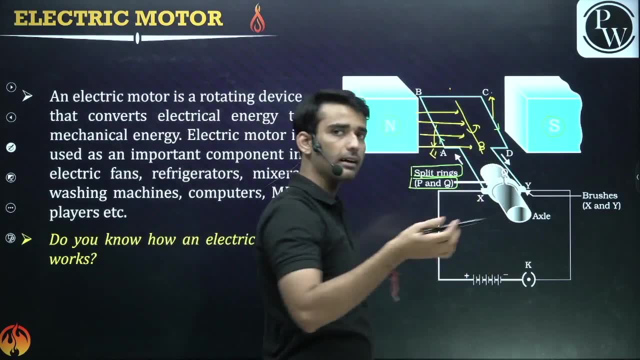 pointing upwards cd would move upwards don't you think it will rotate it will rotate so guys basically this is the principle of electric motor when you place a current carrying wire in magnetic 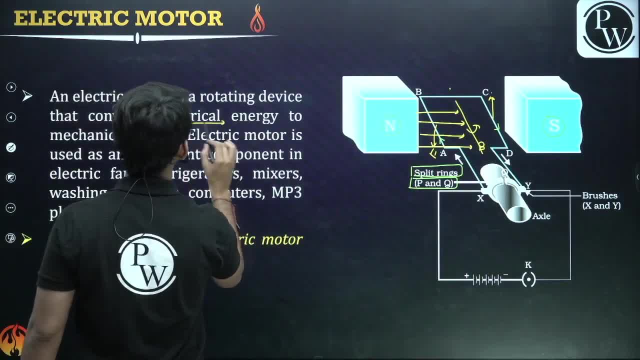 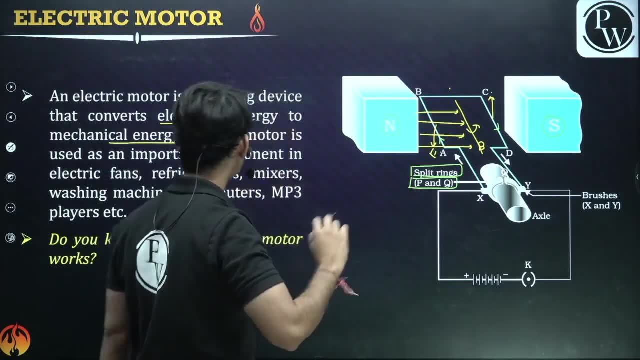 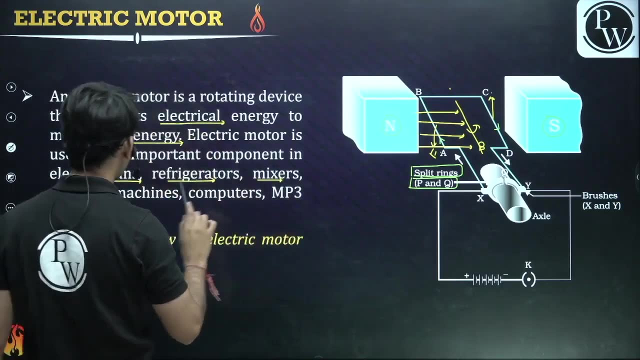 field it rotates so it is device that converts electrical energy into mechanical energy current is through current is flown and it is moving mechanical energy is provided so important is it is used in electric fans it is used in refrigerator grinder mixer we all have that in home right washing machine is used in refrigerator grinder mixer we all have that in home right washing 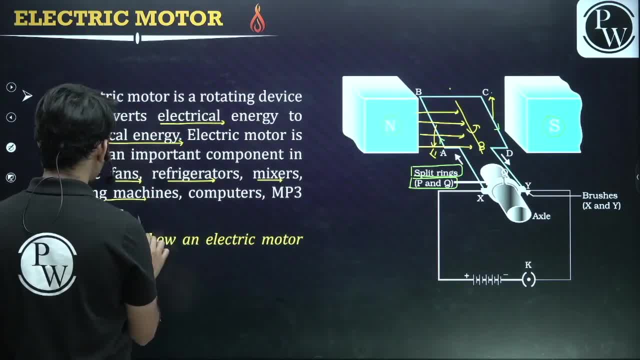 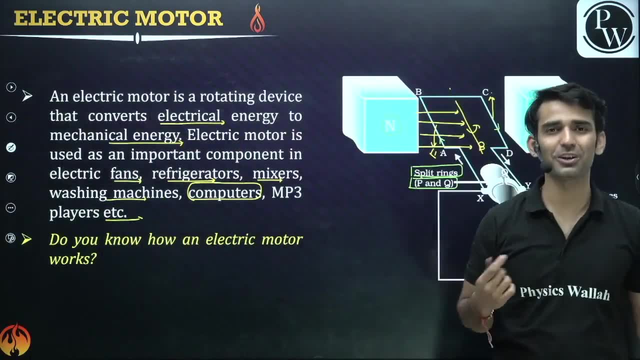 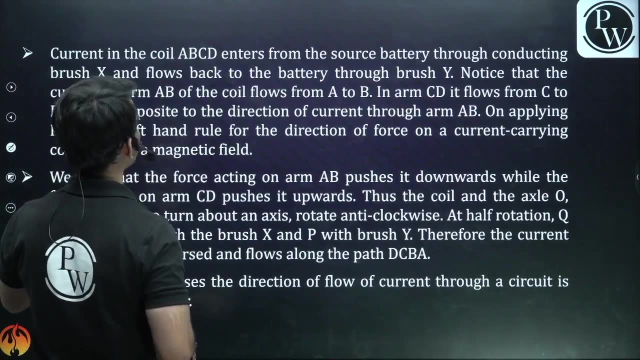 machine it also rotates that is electric motor mp3 players we used to have the other them in computers we also have electric motor the fan right the cooling fan it is also an electric motor so we have this application in many cases now question is how does it work as i have told you if you place the coil in external magnetic field so the current flows the theory is completely 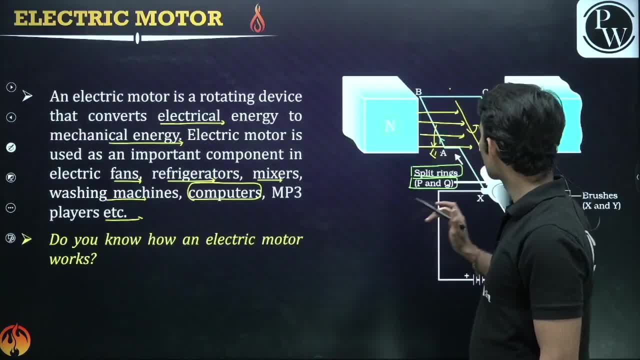 written i have what i have told you just use the fleming's left hand rule to direction the find 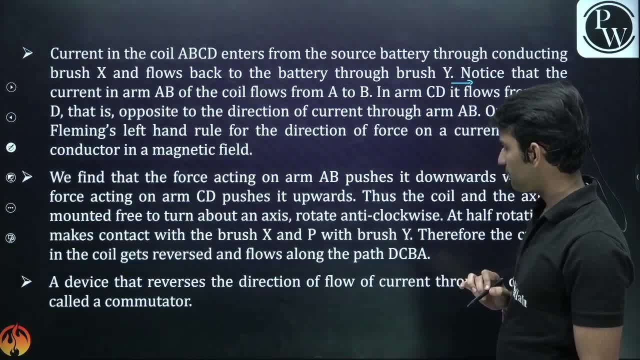 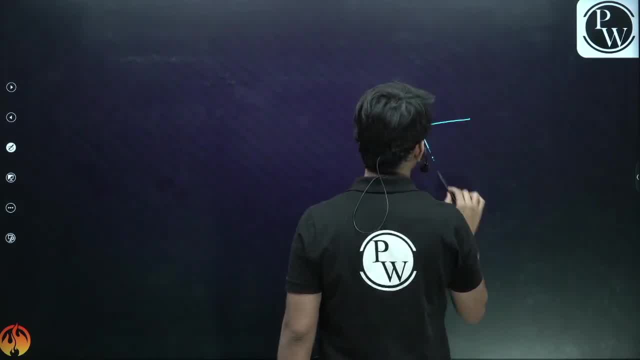 the direction of the current now guys thing is basically after half rotation cd would be here a b would be here so after half rotation the situation kind of looks like this cd would be here and a b would be here this is the situation after half rotation after 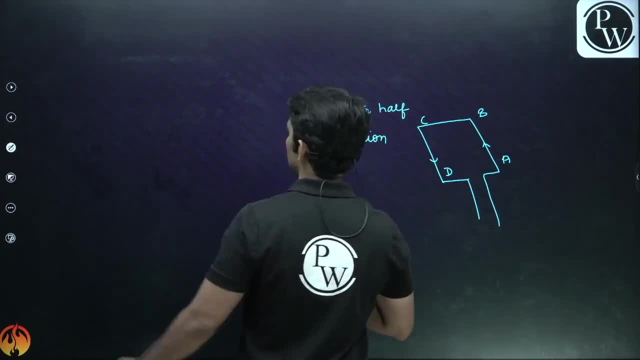 half rotation the situation would be like this okay guys now if i want to find the direction of the current on cd 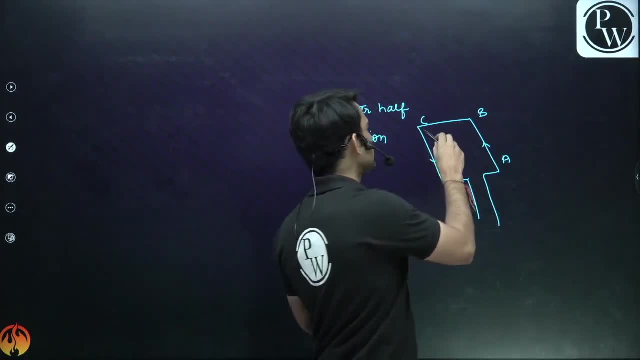 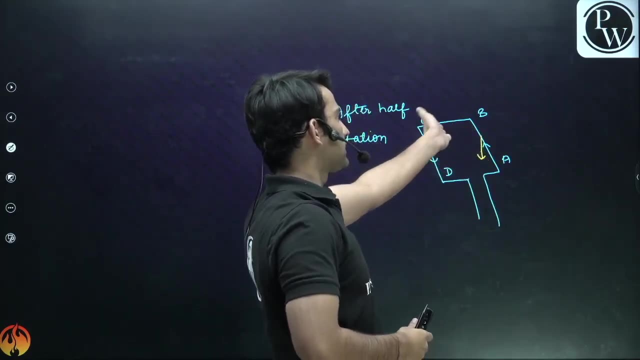 just middle finger towards you right forefinger here so you can see cd is going upwards and a b is going downwards that means initially the coil is rotated like this 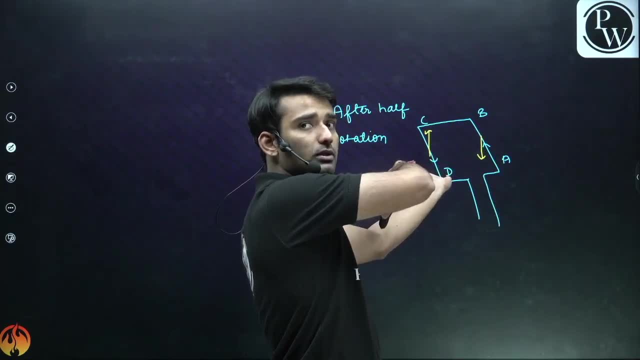 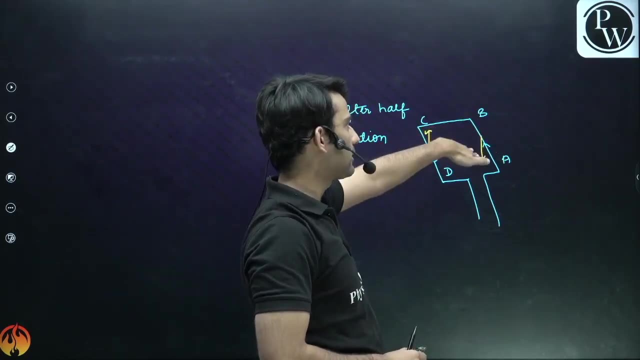 but now left hand is up experiencing force upwards the coil will rotate like this so has it completed one revolution no like this and like this like this and like this but this does not happen why because 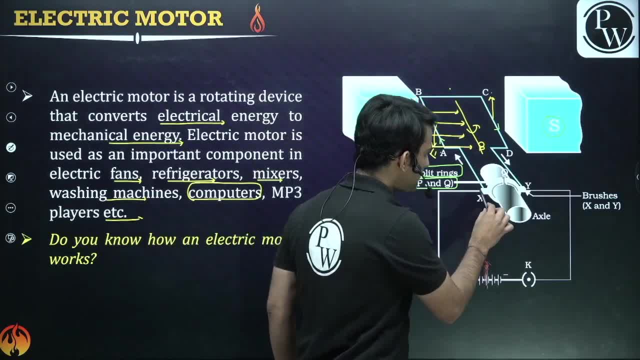 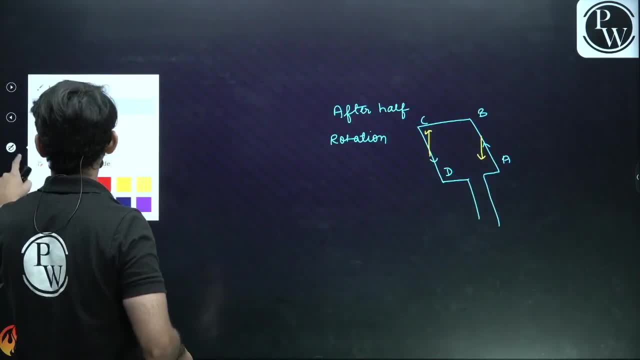 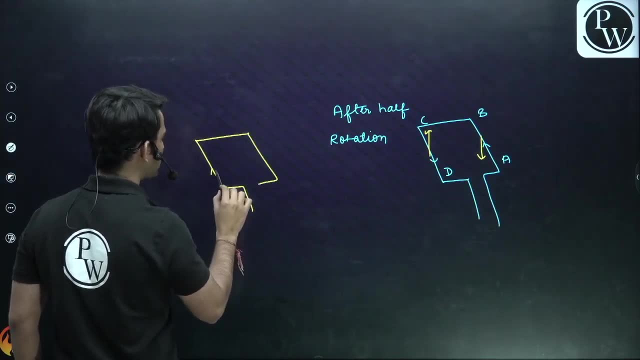 guys we have split rings here basically they change the direction of current after every half rotation they just reverse their connection that means after half rotation guys after half rotation the current in the arms will be interchanged in cd it would be upwards and in ab it would be downwards now they can complete one rotation like this and now now they can complete 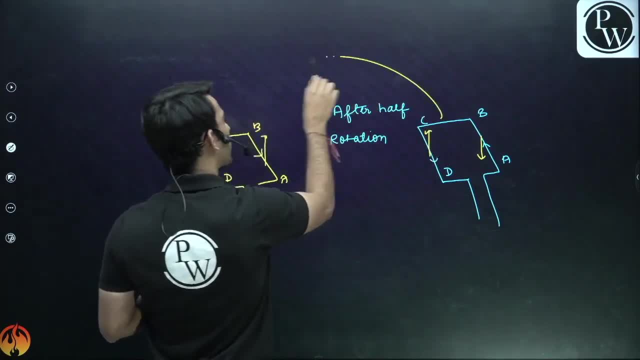 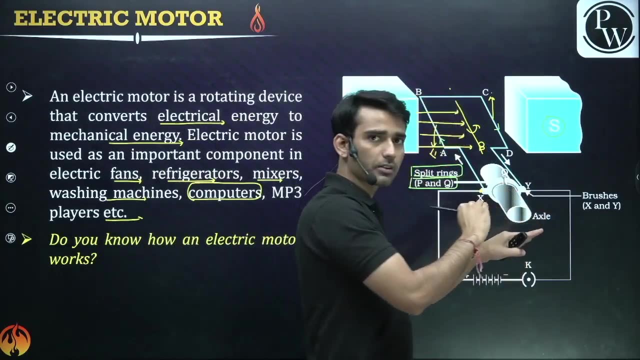 one rotation so this change of direction after every half rotation is performed by the splitting their brushes carbon brushes so this just interchanges the connections the brushes kind of when they move the interchanges the connection right so this is the role of the split rings 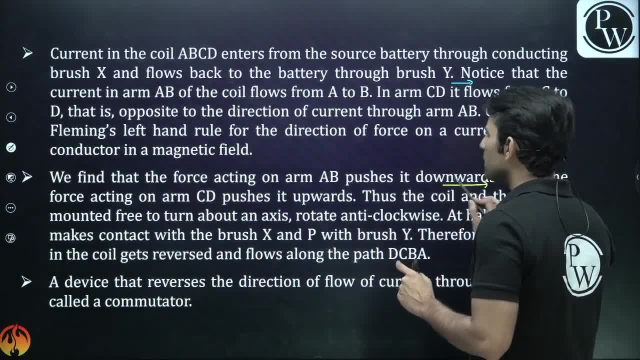 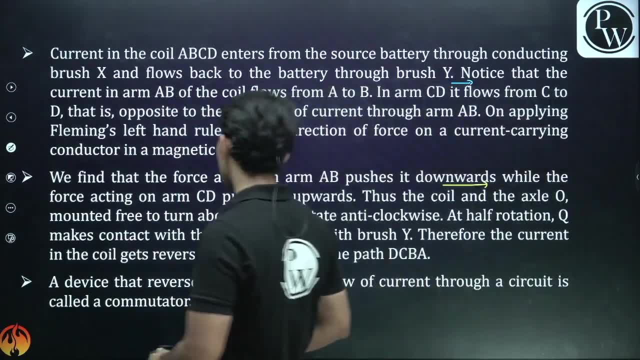 so the force acting on the uh the complete theory has been written what i have told you this is from ncrt so just rotate the clockwise after every half rotation the direction of the current has to be and this is uh 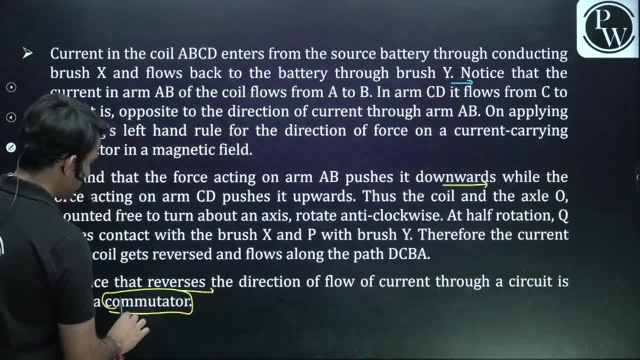 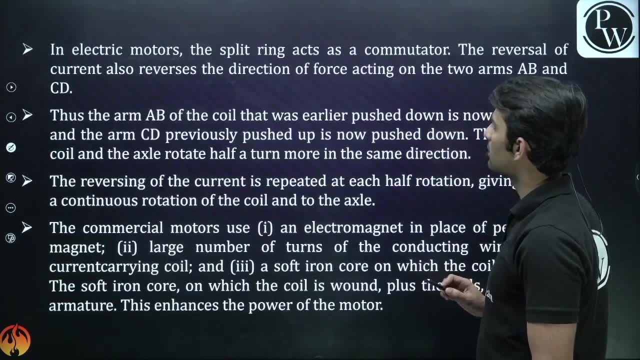 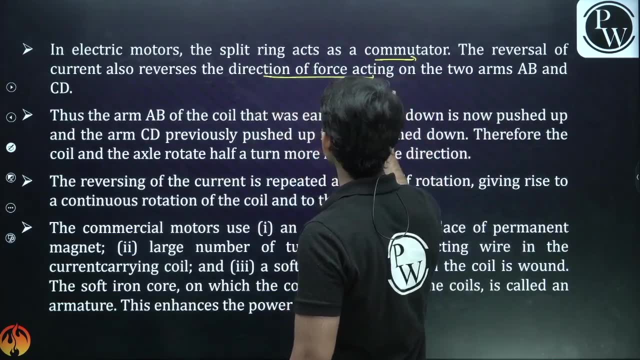 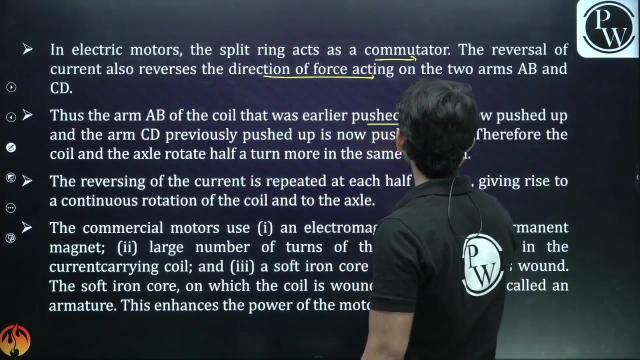 performed by the commutator this is performed by the commutator or splittering after every half rotation so this is on which the uh this motor works so electric motor split ring act as a commutator and reversal of current also reverses direction of force and we can we can have a complete motion complete rotation arm ab of the coil that was earlier pushed downwards now it is 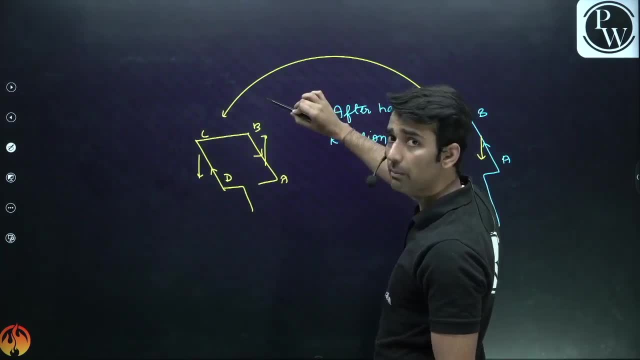 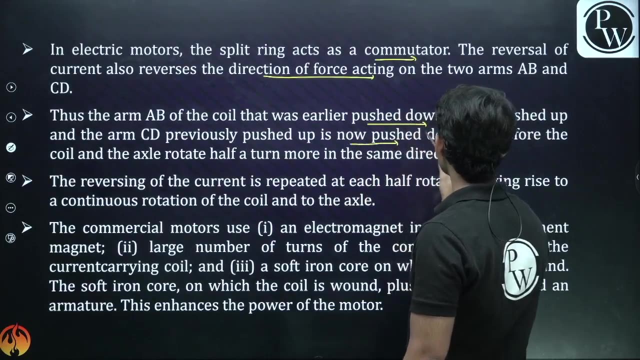 pushed upwards can you see it now it is pushed upwards arm ab initially it was pushing downwards now it is pushed upwards right guys so cd previously pushed up now is pushed downwards therefore excel rotate half a turn more in same direction it will more than half a turn 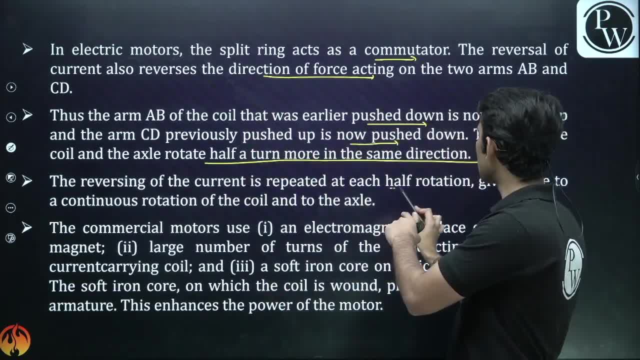 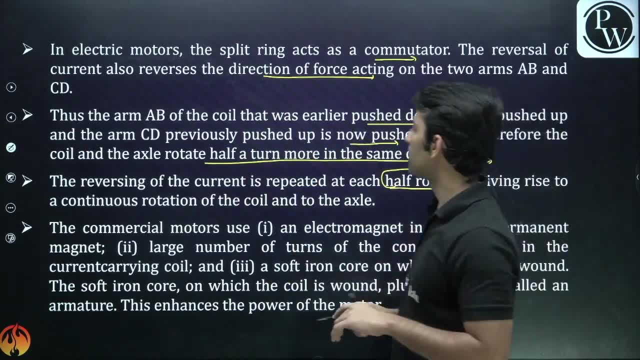 complete turn so reversing of current is repeated at each half rotation after every half rotation the direction of current has to be reversed to make the continuous rotation so commercial motor 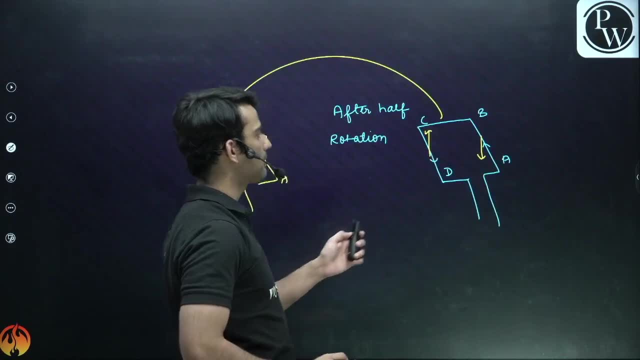 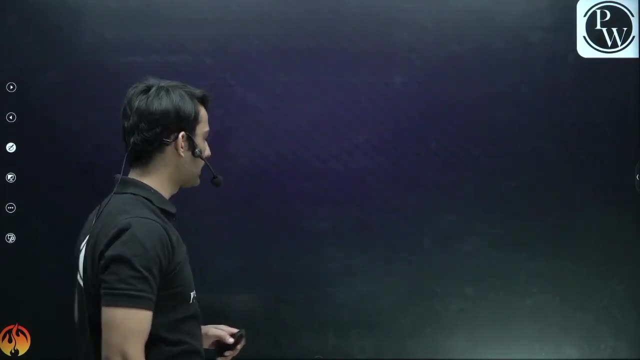 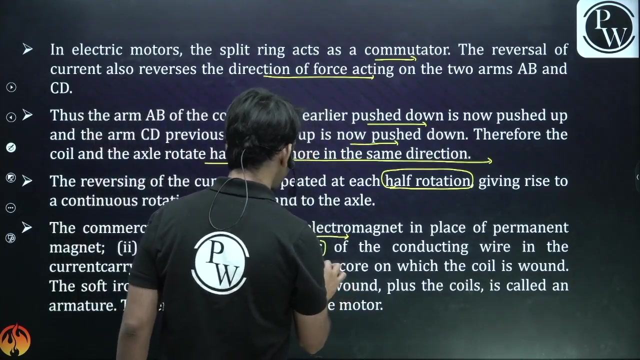 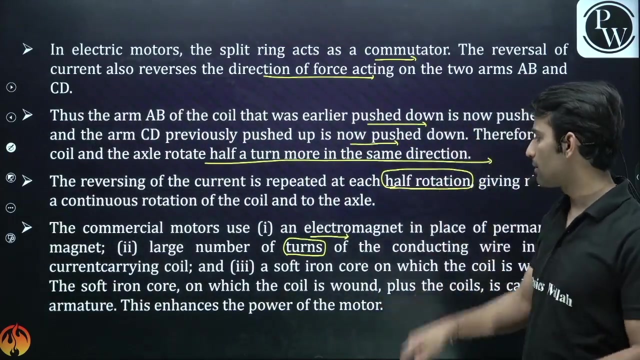 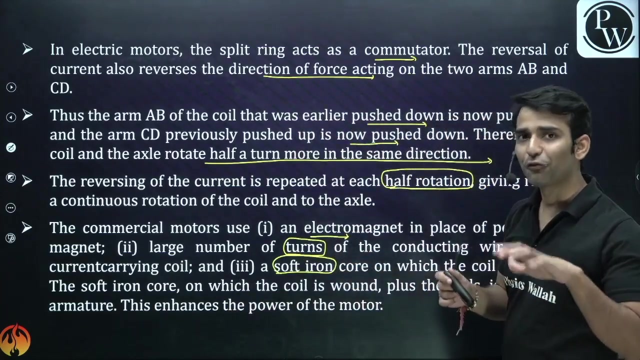 use electromagnet in place of c we have normal magnet here but in commercial motor nowadays we have a electromagnet in place of these two magnets right guys and okay also we have a basically large number of turns if you want to increase the field i had told you just increase the number of turns if you want to increase the field increase the rotation just increase the number of turns also if you play the soft iron core guys i had told you it will increase the magnetic field and as a result the force experienced will be increased so this enhances the power of the motor so guys 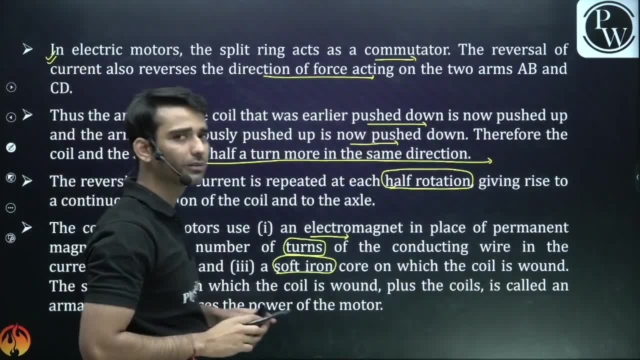 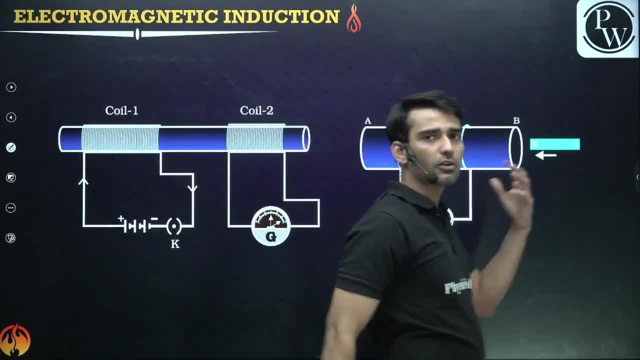 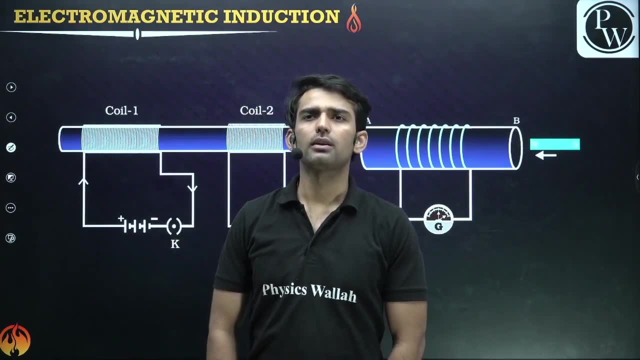 this is the complete working or the construction and the principle of the electric motor now next part of the chapter is electromagnetic induction so guys farazdeh was the physicist which uh who told us about this phenomena of electromagnetic induction now question is how does it perform 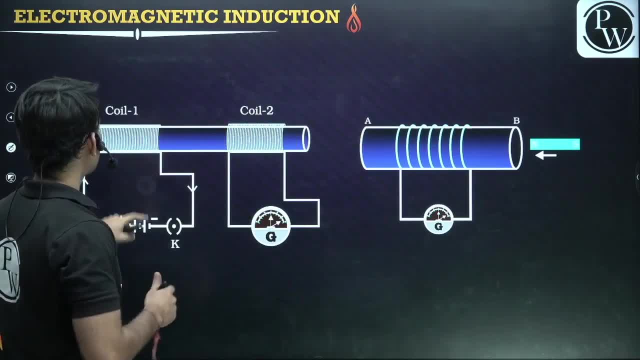 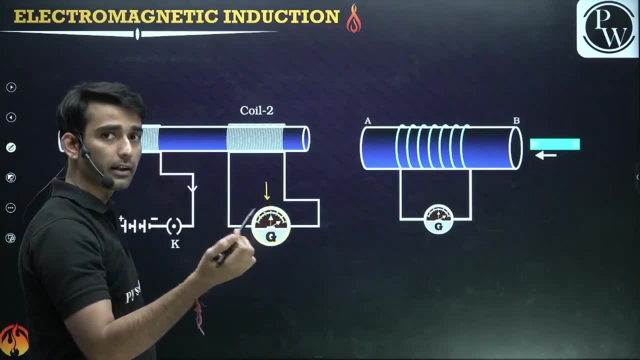 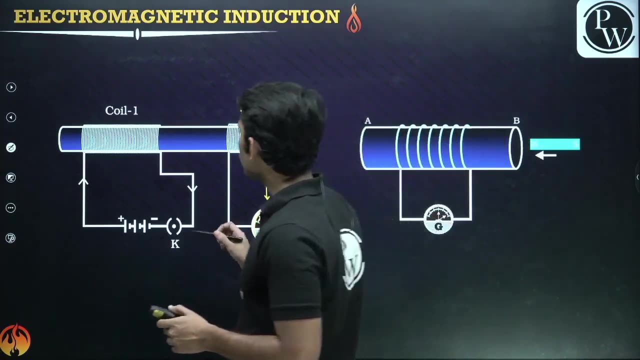 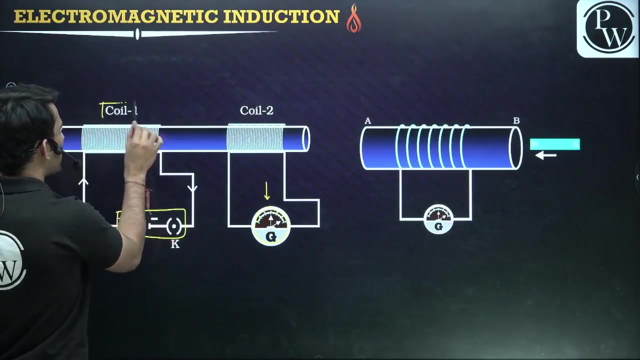 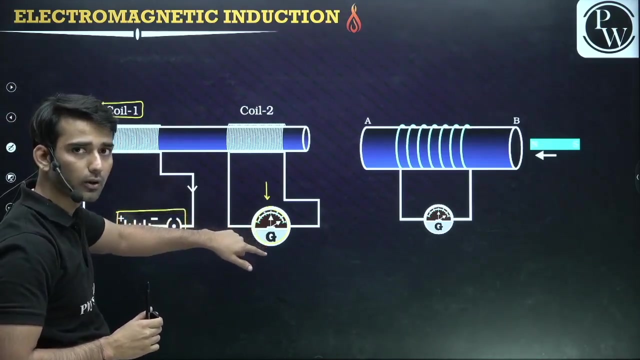 see basically what he had done he had taken a coil two coils nearby each other and had connected galvanometer galvanometer just deflects the def is deflected this needle is deflected as soon as some amount of current passes through this okay guys now what he had done basically he s he had taken uh this uh battery and the key in the coil one he had observed as soon as he had plug in the key the deflection there is some deflection in the coil not for a long time as soon as he plugged after some time it is zero deflection is zero but 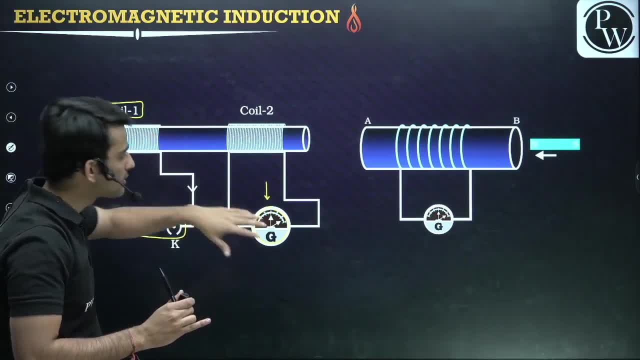 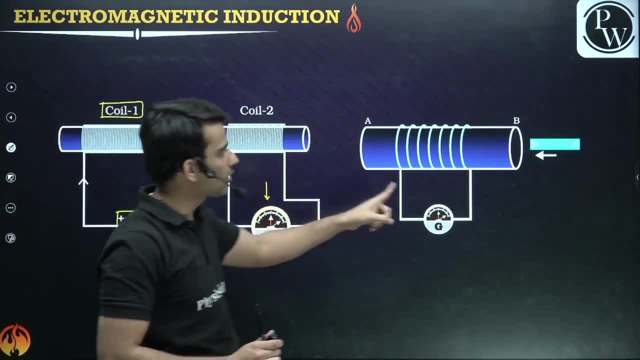 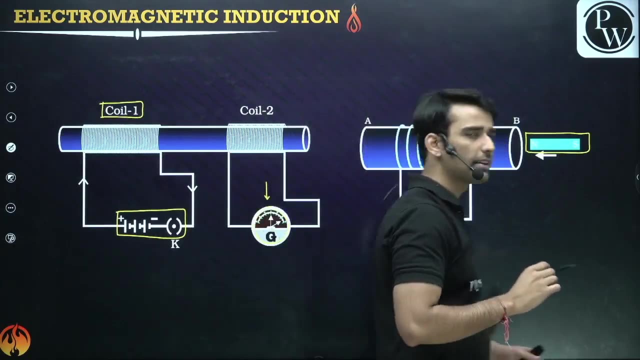 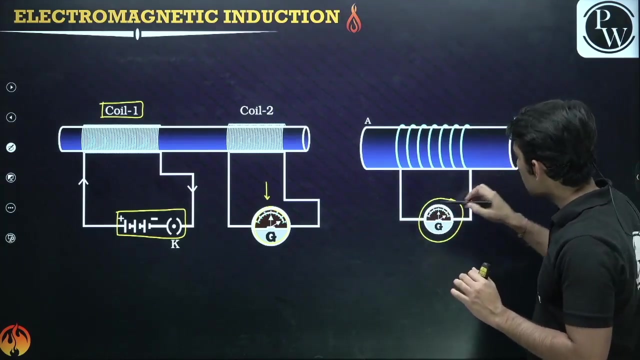 and also as soon as he plugs plugged out the key there is some deflection but not for long time after some time the reflection would be again zero same here also he had taken instead of coil one he had taken a bar magnet what he had observed that if you bring this bar magnet near the coil there is some deflection in the galvanometer now thing is we don't have any battery here but still we are getting any deflection we are getting some current why is that 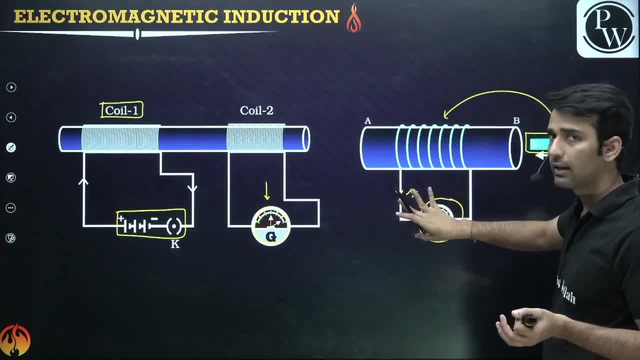 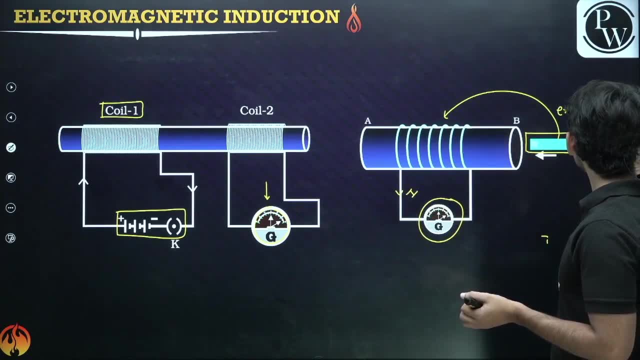 because this is how you induce the current in this circuit by some external source so guys this phenomena is known as electromagnetic induction you induce the current from one body to another 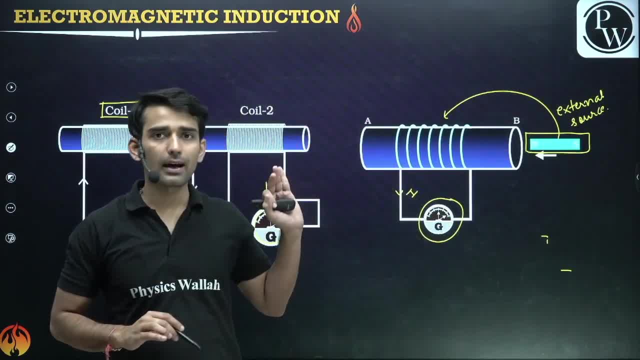 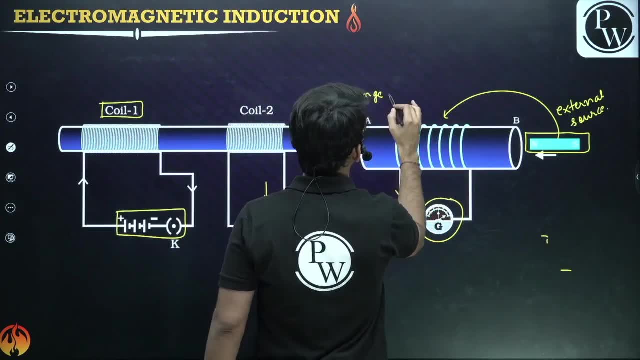 electromagnetic induction right so when you move the magnet when you change the magnetic field the cause is the change of magnetic field across this coil change of magnetic field 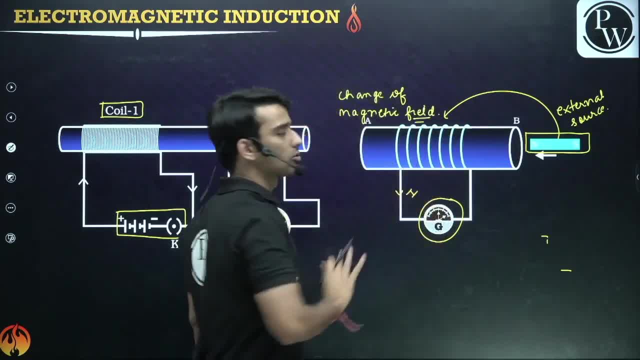 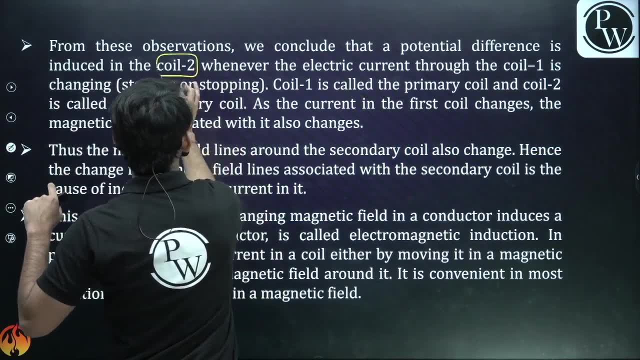 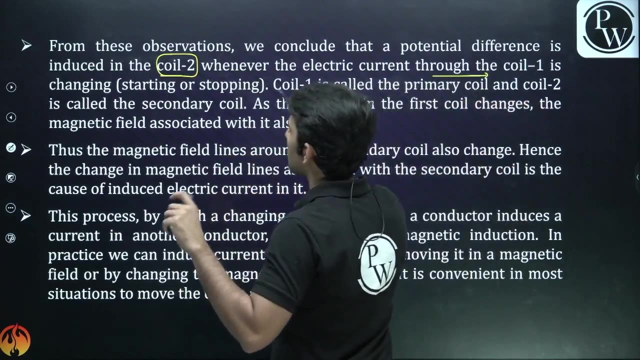 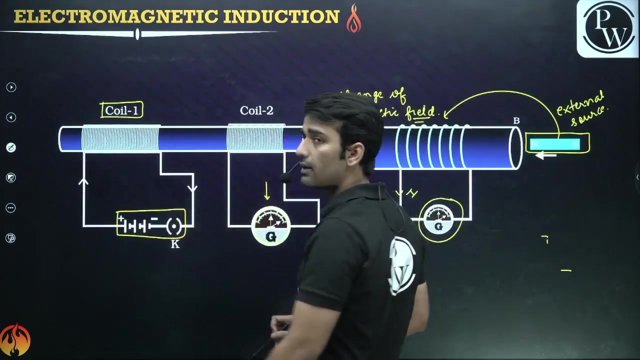 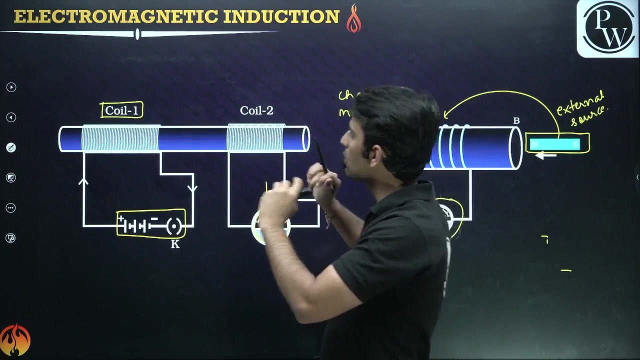 magnetic field across this coil this is the cause of it okay so from this experiment we conclude that potential difference is induced in coil two potential difference or we call it emf or we call it as a result we have electric current through the coil one as soon as you see if you change the current through this coil some emf it is induced in this coil because on changing the current the magnetic field would be changed across this because they they are the kind of on the same current uh soft iron core so if you change field on this the field through this coil would be 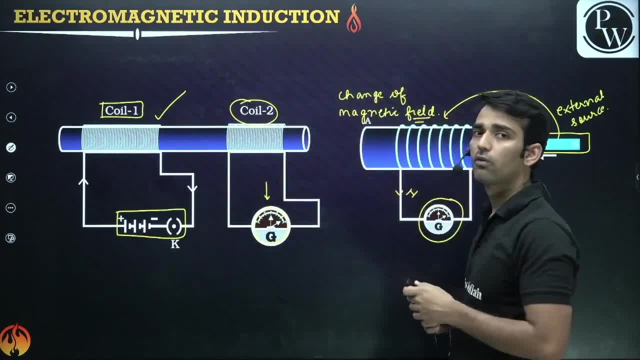 changed and as a result we have some amount of current flowing through this okay so whenever 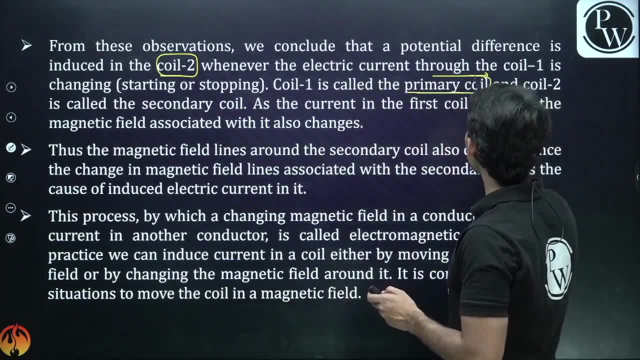 electric current through the coil one is changing coil one is called primary coil the one in which we already have current and the one in which current is induced is called guys secondary coil 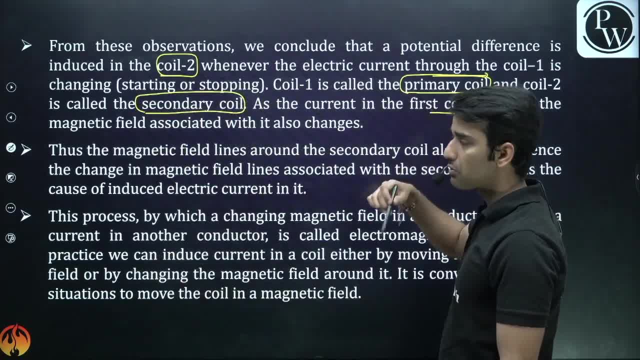 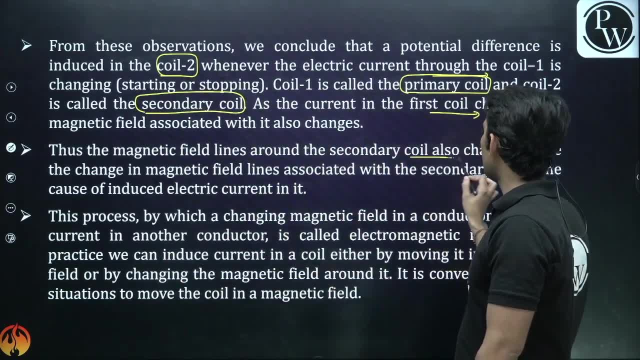 right if you change the current in the primary the magnetic field associated with the primary would also change and as a result we have current induced in the secondary coil so magnetic field lines around the secondary coil also changes and we have current induced the process by which 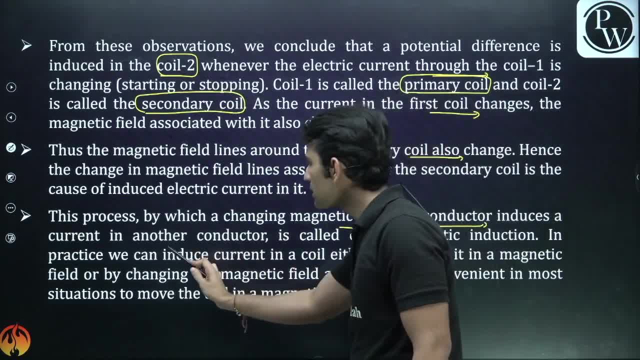 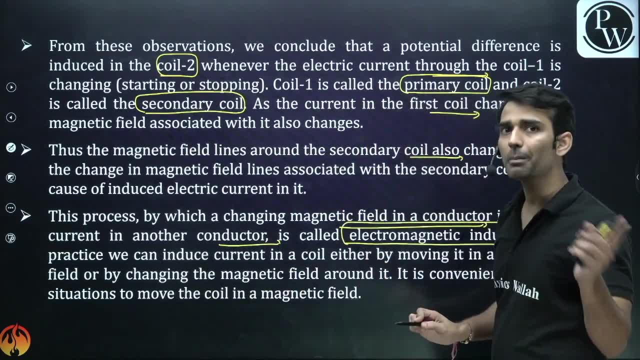 changing magnetic field around the conductor induces a current in another conductor this phenomena or process is called electromagnetic induction we have current from magnetic field at the start of this chapter we had learned about the magnetic field due to current 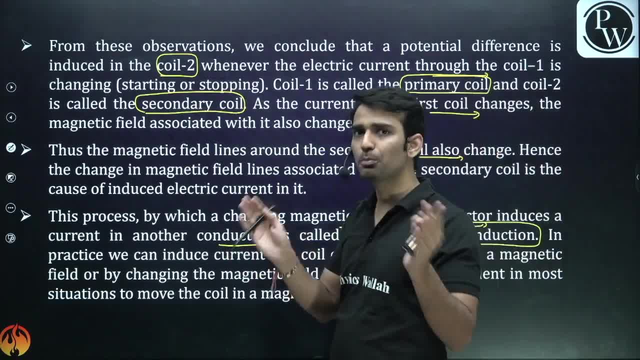 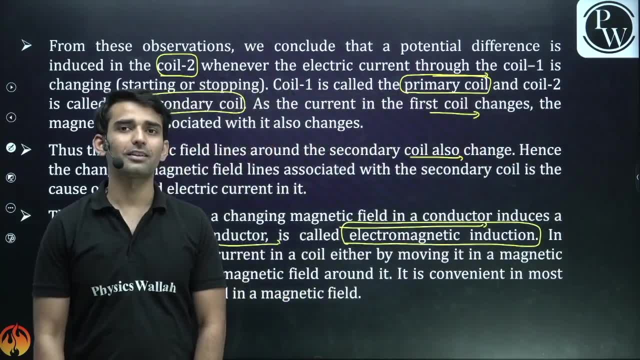 now we have current due to magnetic field so we have both the process right guys so changing magnetic field we have current induced right this 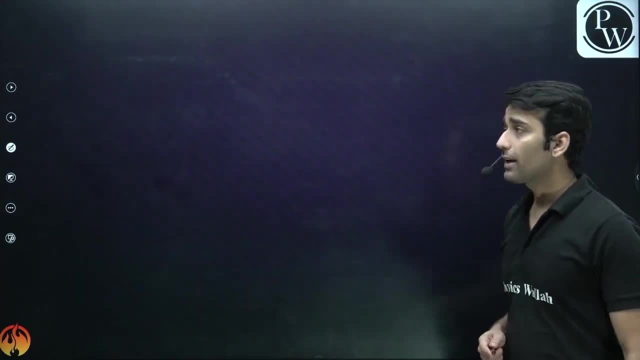 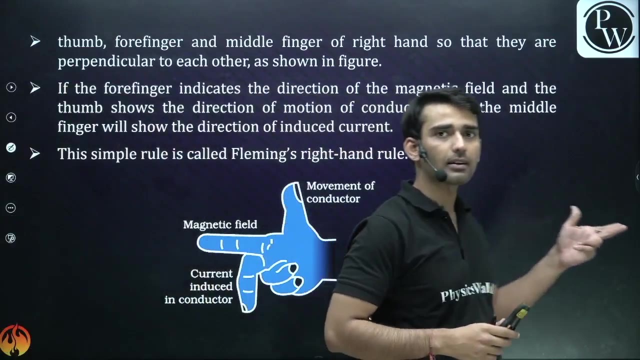 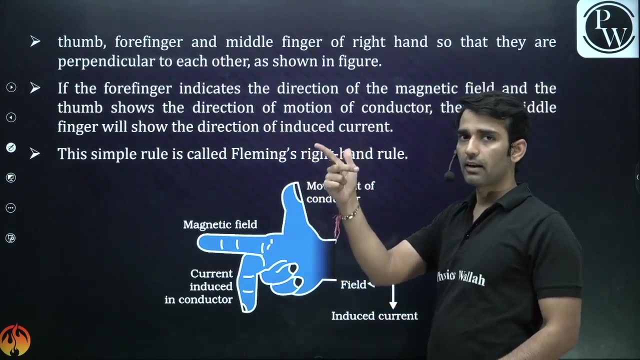 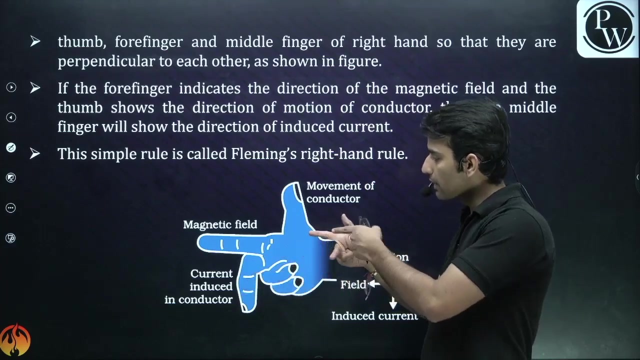 was found out by the faraday michael faraday okay now question is how can we find the direction of the induced current guys like we had right fleming's left hand rule we have fleming's right hand rule what does this rule state just take your right hand forefinger middle finger and the thumb your middle finger will again show will point in the direction of the current forefinger 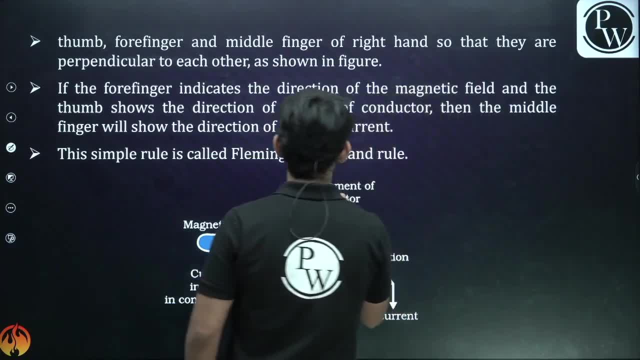 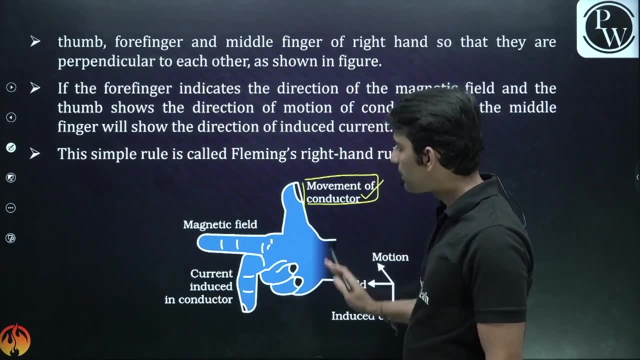 in the direction of magnetic field so guys the movement of the conductor or the force will be along the thumb that the direction in which the conductor would move will be along the thumb so this is fleming's right hand rule forefinger middle finger and thumb are stressed as shown in the figure direction of magnetic field is given by the forefinger thumb points in the direction of motion or the direction of the force 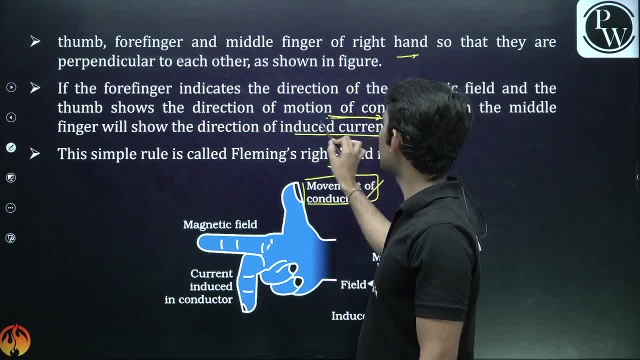 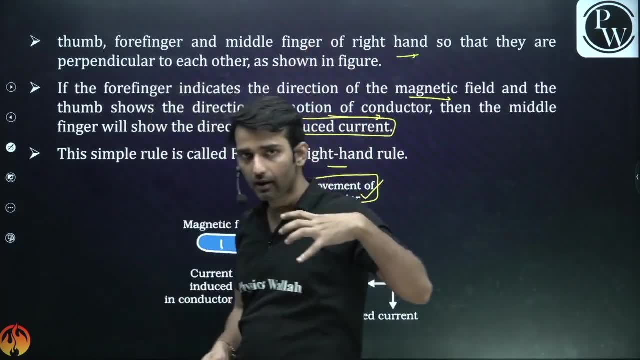 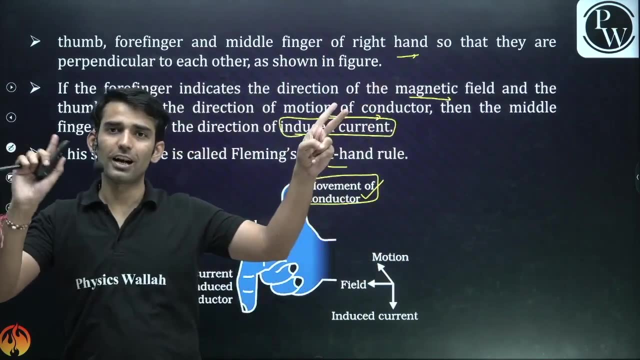 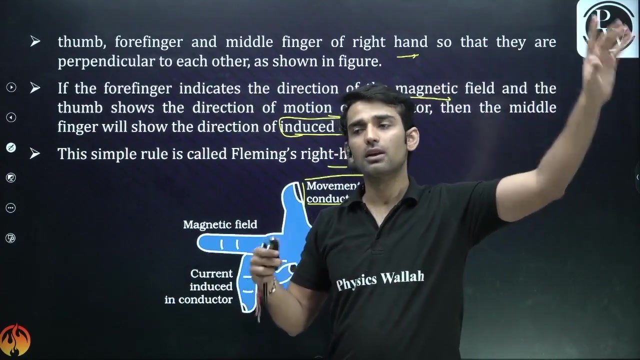 and middle finger will point in the direction of induced current fleming's right hand rule so from left hand rule we used to find the direction of the force and from left hand uh from right hand rule we find the direction of the induced current so both are different both right left hand and right hand rule are different don't don't basically merge them what i have seen student basically get confused in both the laws that was for the force this is for the induced current okay guys now based on this phenomena 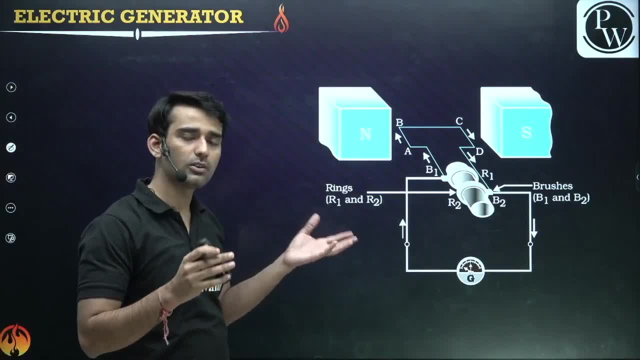 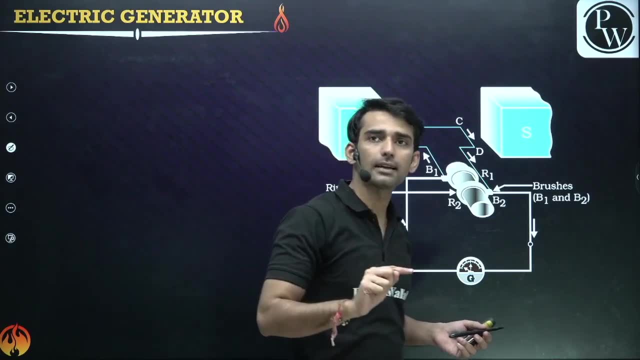 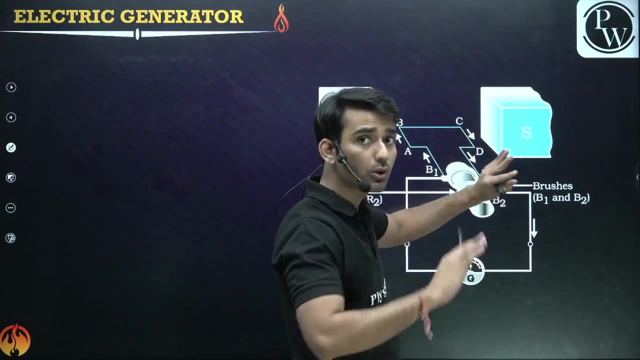 we have electric generator electric generator means we all must have seen those generator in our houses right electric generator gives you electric current now from where does it get the electric current by the expense of the magnetic energy so in electric generator we have kind of same apparatus not quite same north pole south pole we have magnetic field from here to here 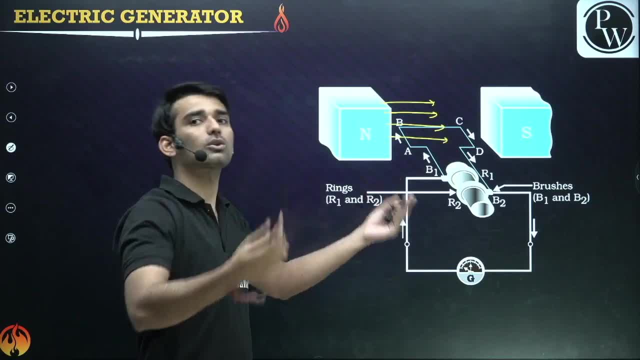 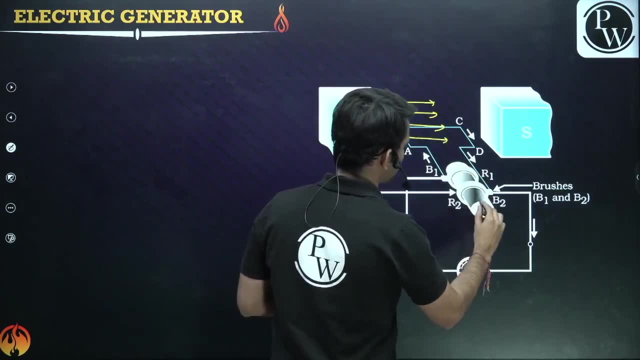 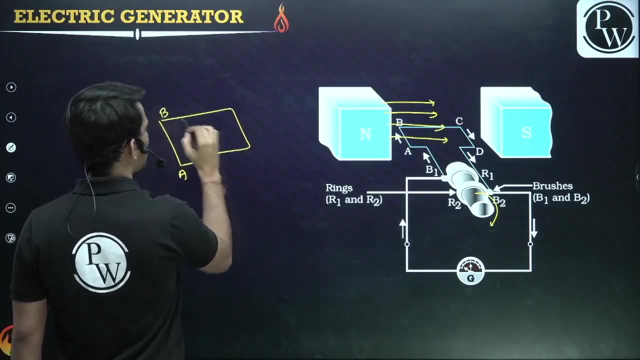 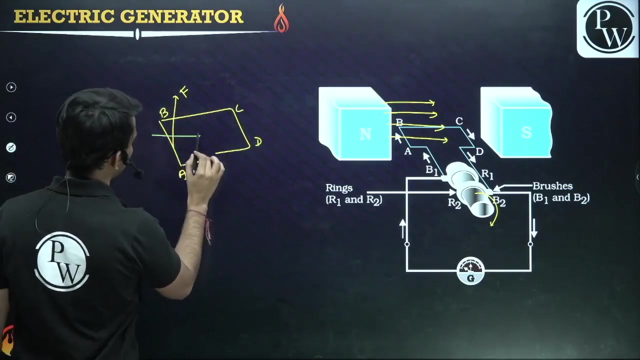 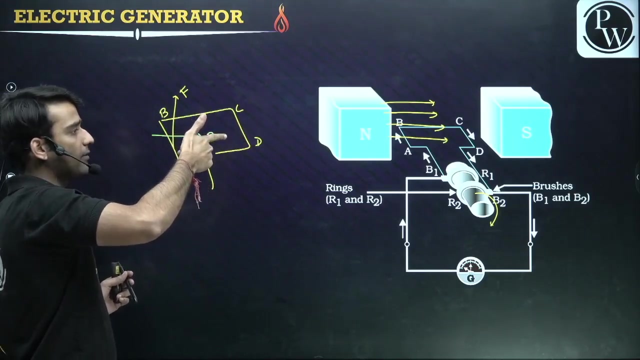 now guys in in electric generator we rotate this coil to get the current so let's say the coil is rotated let's say the coil is rotated like this okay so guys what this means that this is a this is b this is c this is d let's say arm a b is moving upwards right guys and the magnetic field is like this take your right hand right so middle finger uh thumb in upward direction and forefinger here so where is the direct where is my middle finger pointing it reads into the board that means current 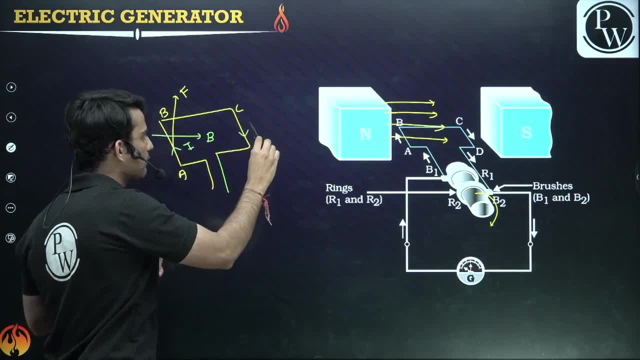 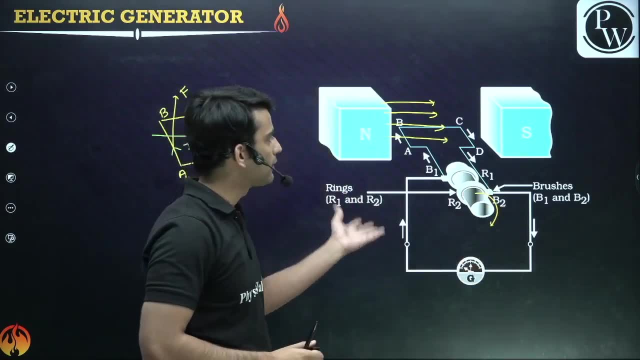 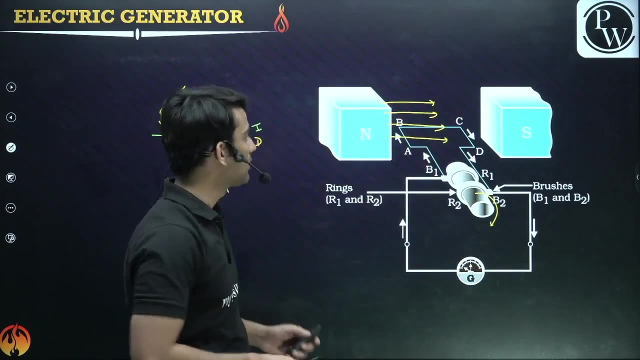 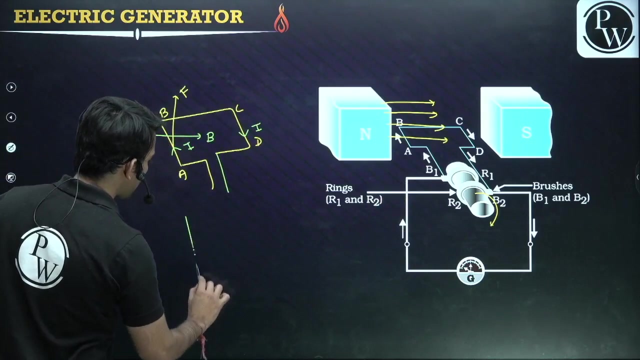 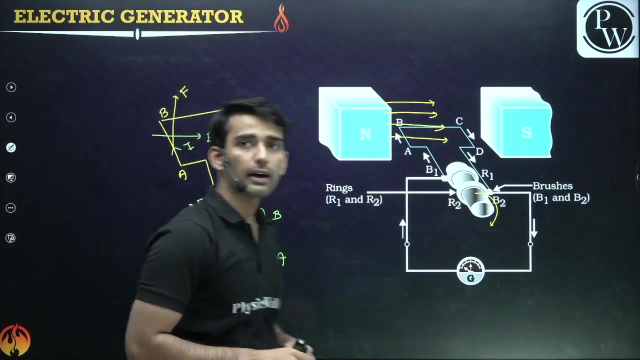 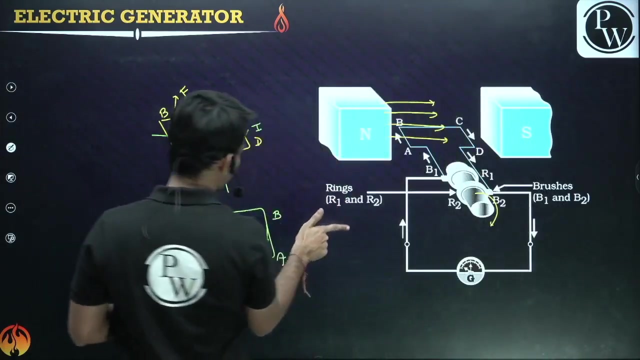 in a b would be like this similarly current in cd would be like this so we are getting some amount of current because here we are expanding our magnetic energy we are rotating the mechanical energy we are getting electrical energy from mechanical energy right guys now question is see basically this is a situation but after half a rotation guys after half a rotation this would be a b and this would be cd a b is going downwards cd is coming upwards right after half a rotation now can you find the direction of induced current in a b right hand rule right just thumb in downward direction magnetic field is like this so here the direction of induced current is a b is like this 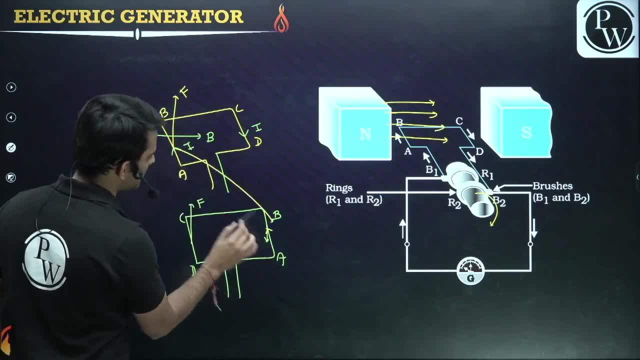 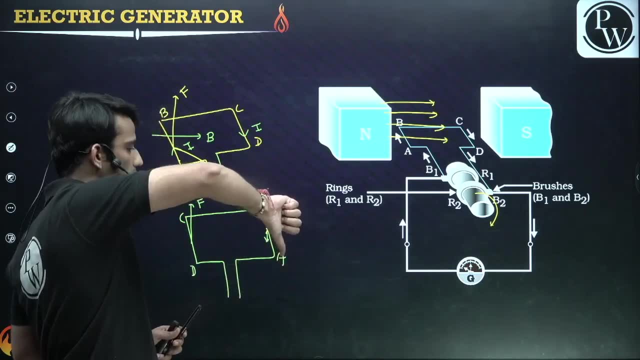 so you can see the direction of induced current in a b is same can you see it guys see because the force is downwards on a b the force is downward right magnetic field is like this so guys you can see basically 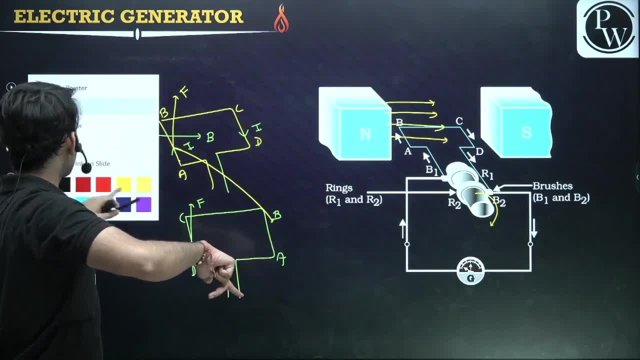 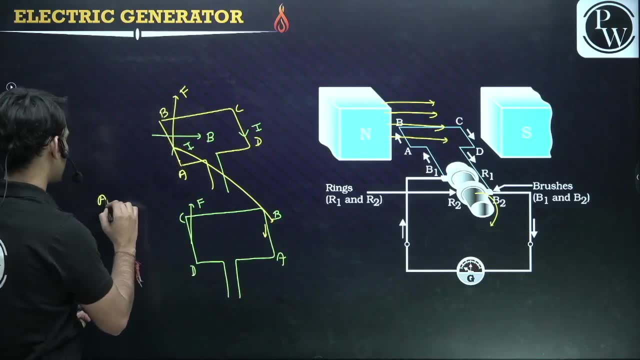 oh yeah fine can you see it guys see listen to me very very carefully the uh force is downwards on a b because a b is moving downwards after half rotation this is after half rotation 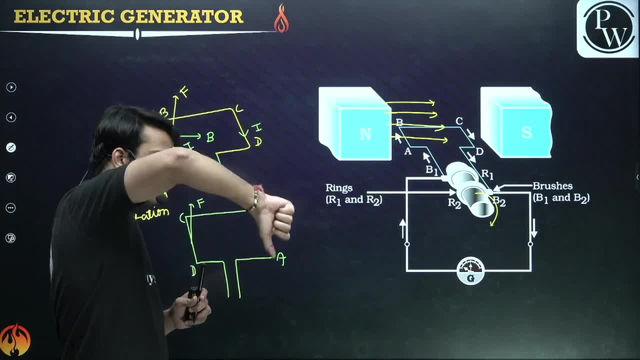 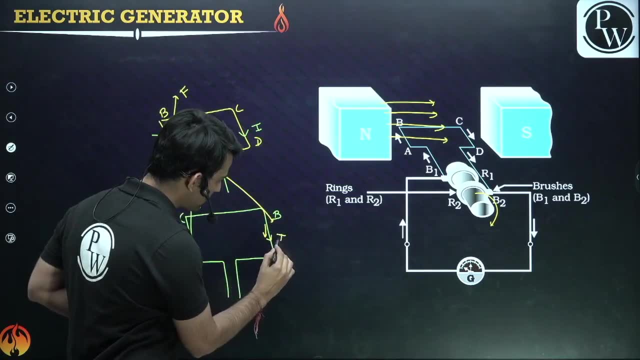 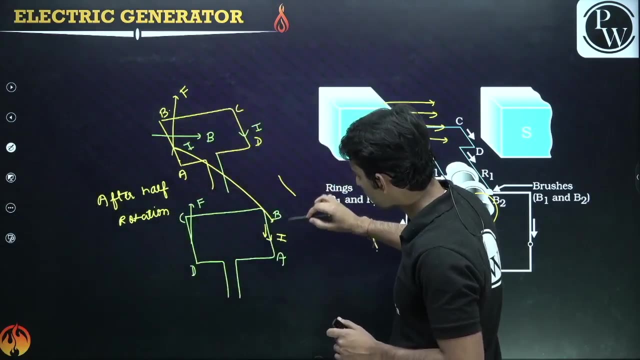 right guys so middle finger thumb downward direction forefinger to the left so you can see the middle finger is pointing towards you that means the current induced in a b would be like this right guys the current induced in the a b here the current was from a to b here the current was from b to a so guys the direction of the induced current is 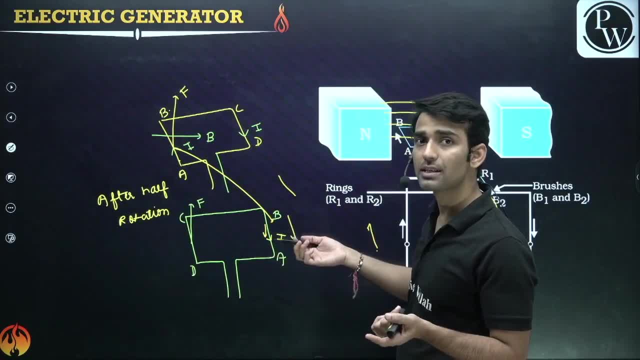 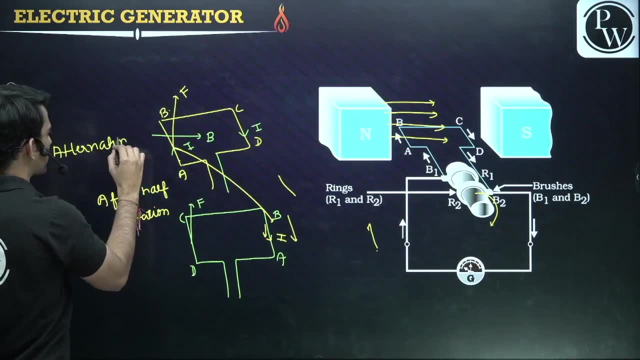 reversed the direction of the induced current is reversed so this is known as alternating current after half cycle the direction of the current is reversed this is called alternating current which 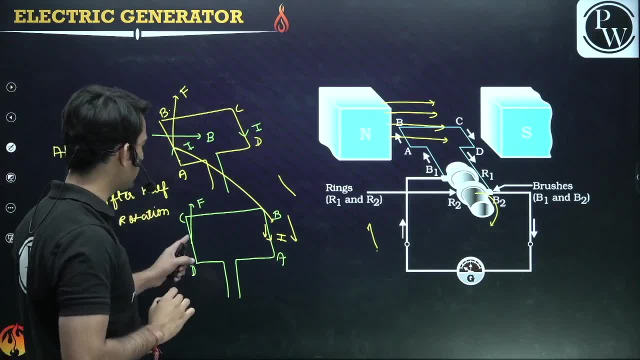 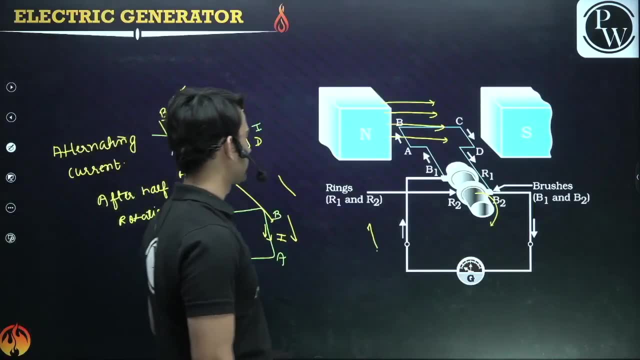 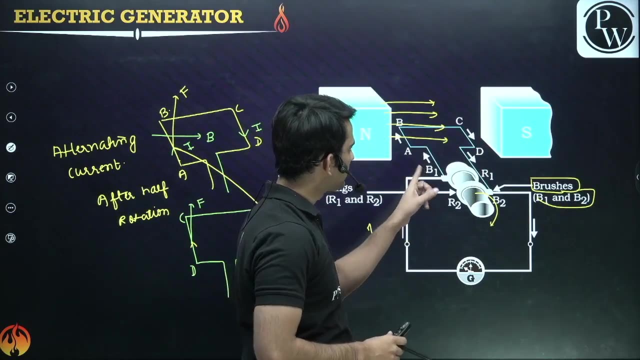 reverses its direction after every half rotation similarly in cd the current is from c to d here current would be from d to c so this is the complete part guys complete part we have brushes we have brushes basically right why do what what do they do because see here a b when the a b would 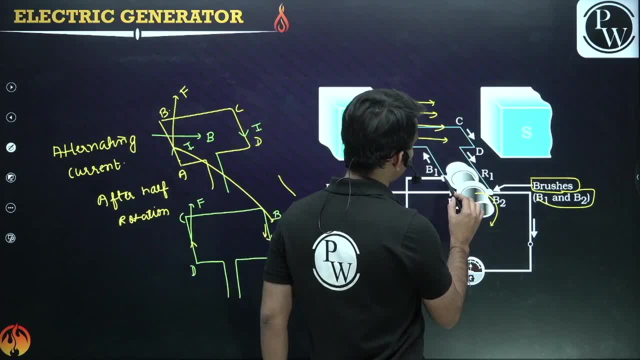 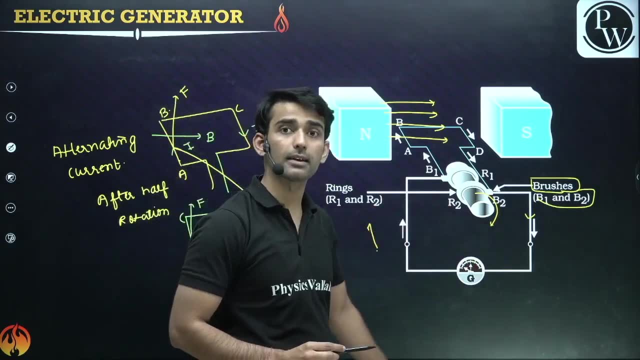 be here and cd would be here what what would be the case this contact is made here so the direction in the outer circuit would be reversed the direction in the outer circuit would be reversed 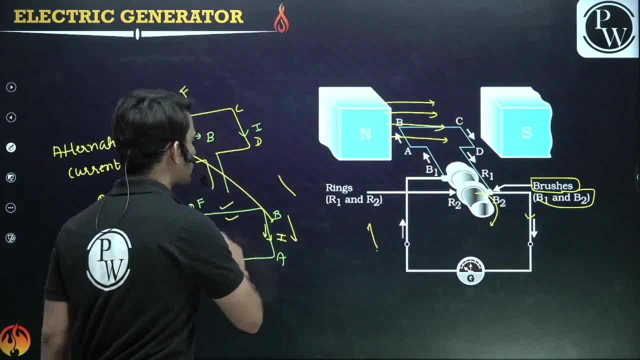 after every half rotation okay guys so this is the case fine so this is basically electric generator 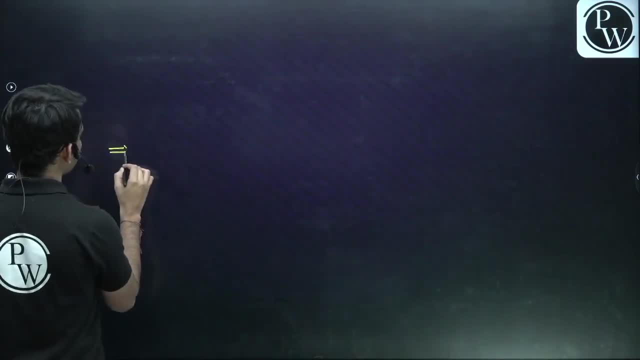 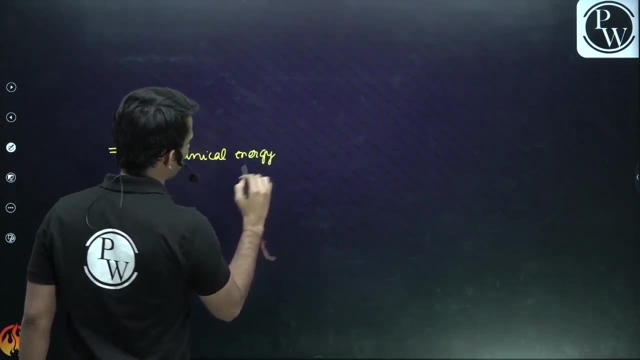 we are converted what type of energy guys what type of energy we are converted mechanical energy into electrical energy mechanical energy into electrical energy fine guys mechanical energy into electrical 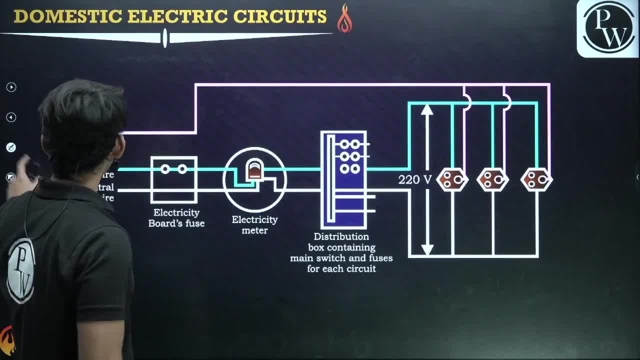 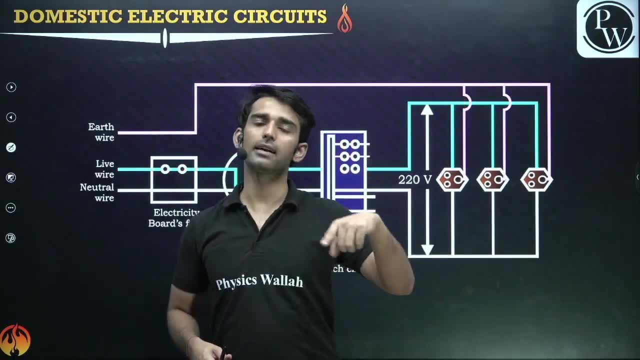 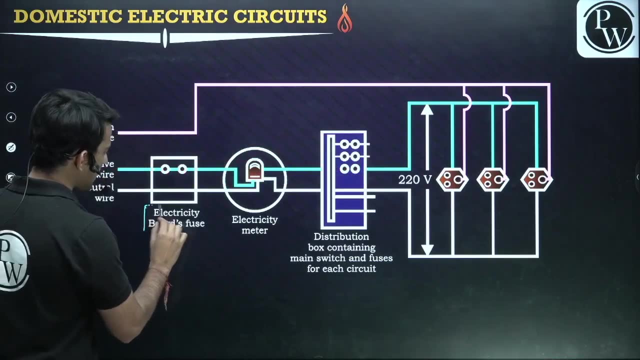 electrical energy clear now last part of the chapter is electric circuit or domestic circuit guys we have a wiring in our circuit we have three wires live wire neutral wire and earthing we get current from the live wire so basically this blue one is a live wire as soon as it enters our house it passes through a board fuse right then it passes through electric meter left from electric meter we have live wire we have neutral wire the meter after meter we have a distribution box in our houses we have a distribution box in our houses we have a distribution box in our houses 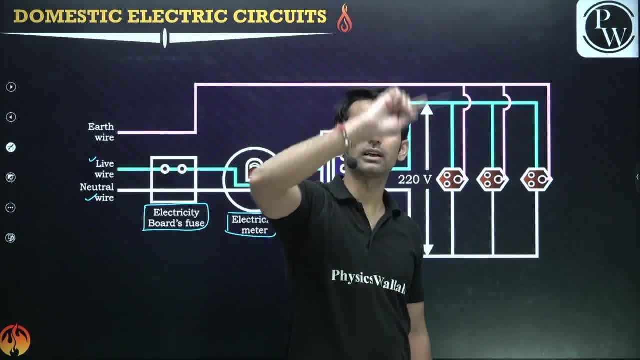 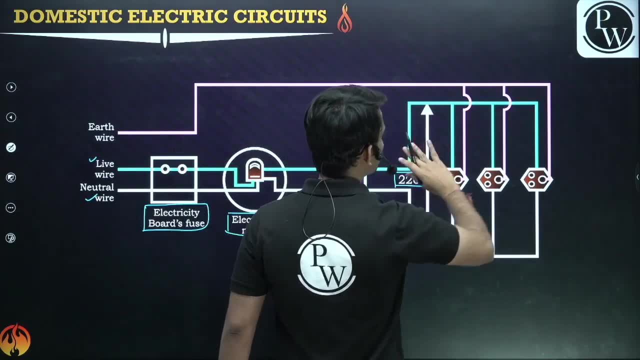 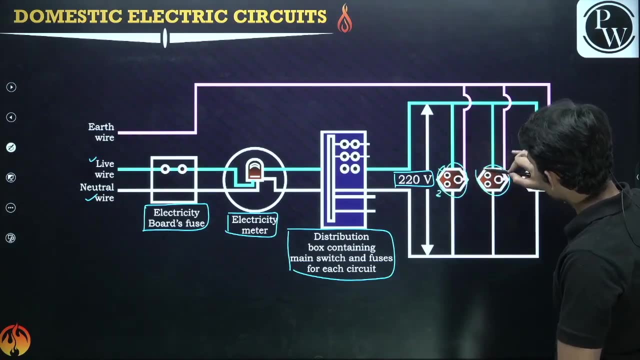 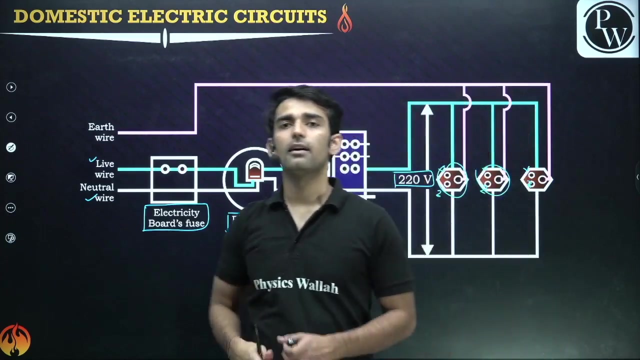 from where that the the wire to the different rooms gets distributed so guys you can see the voltage we get in our homes is 220 volt so you can see all the appliances are connected in parallel for for every socket we have one live one neutral one live one neutral one live one neutral this pink one is the earth wire what is the cause of role of earth wire when we just when we get a excessive current basically with uh when when the current when we get an excessive current basically 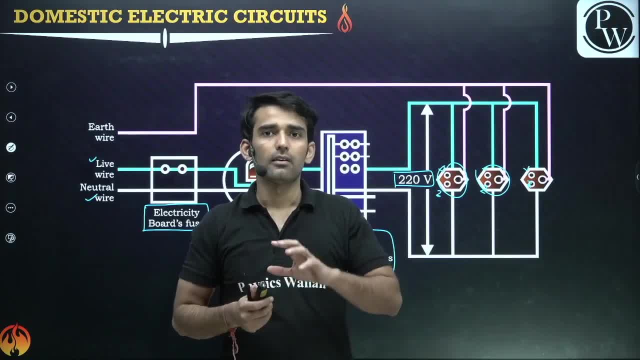 when any metal body experiences some current right for example if you are in a fridge or in 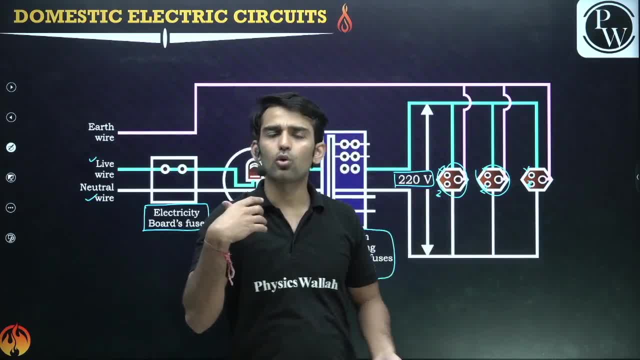 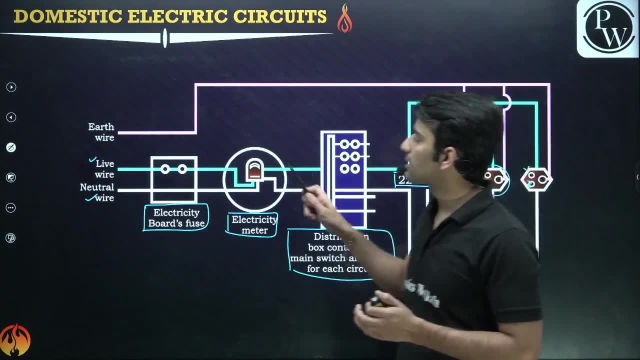 refrigerator or in ac live wire could could touch the body of the uh metal body that means we may get the electric shock in such a situation we connects a earth wire the third socket 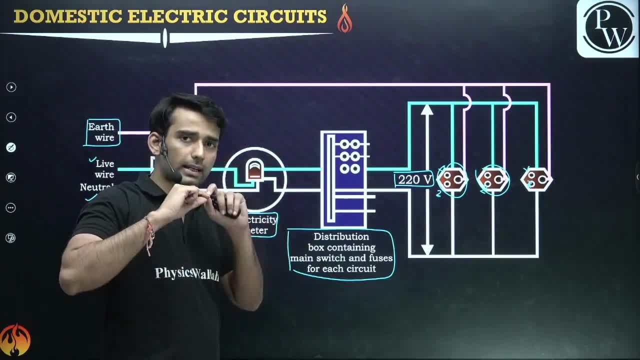 to the circuit what does the earth wire do it takes that excessive current towards the earth 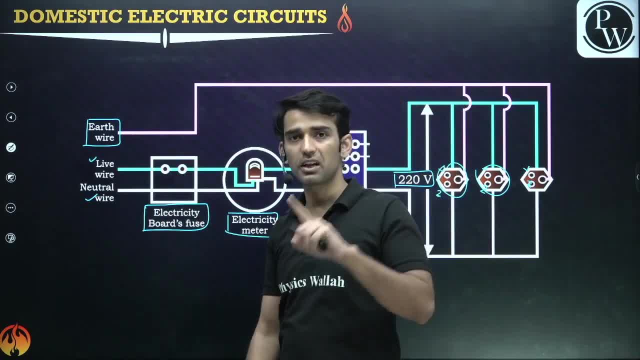 it is connected to the earth and the earth is having us the infinite potential right so it is 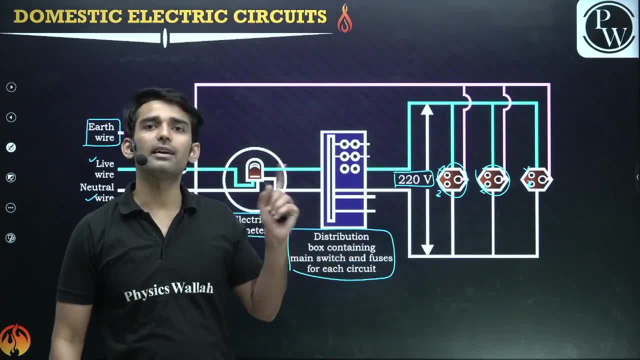 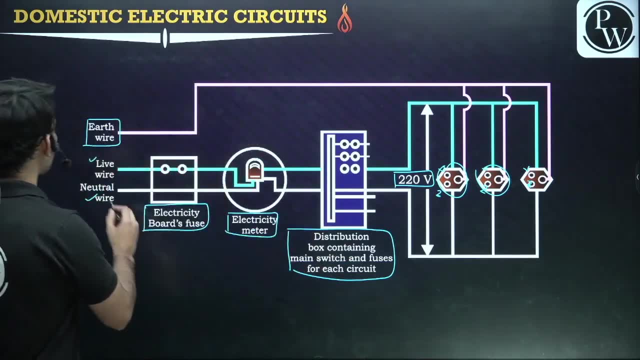 earth so that current flows to the earth and it is we are preventing prevented from getting an electric shock so guys this is happens in the electric circuit basically we have earth wire 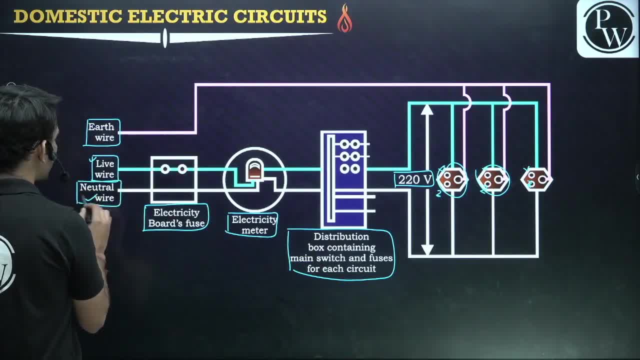 from live wire basically we have current and from neutral wire we are it's a neutral wire right we don't have current here and the potential difference between these two wire is 220 volt the potential difference between these two wires is 220 volt so for every connection you can see whether it is it a series or parallel connection obviously guys 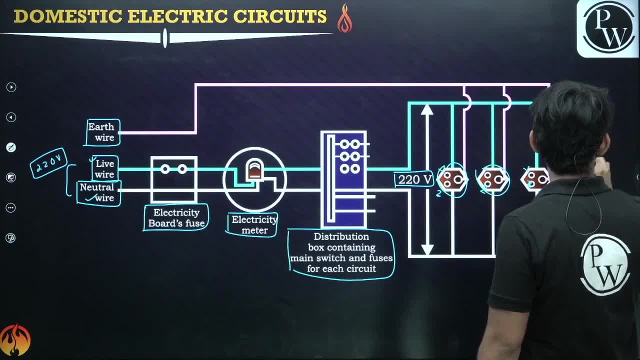 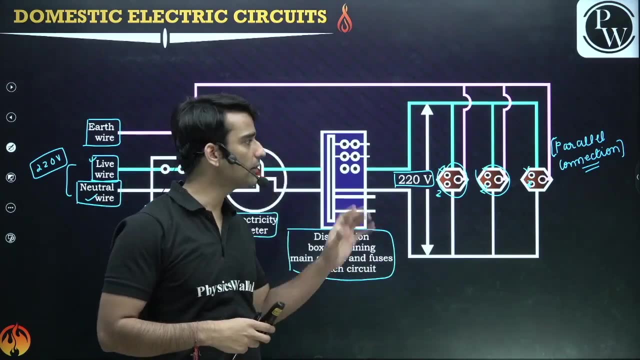 this is parallel connection i had told you in electricity this is parallel connection this is parallel connection the field lines the this is in connected in parallel right because in parallel we have we have same voltage and current is distributed accordingly also if one 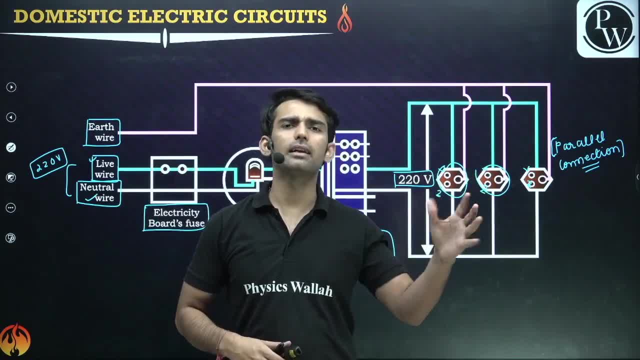 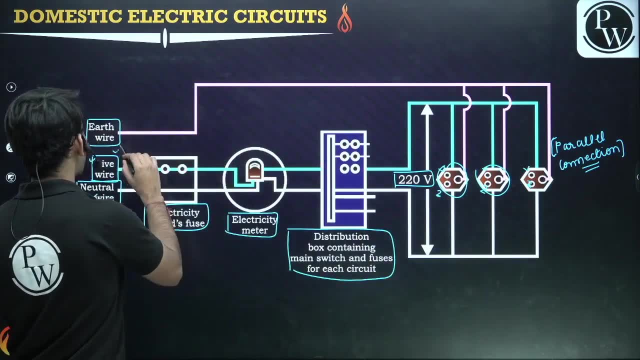 of the appliance is affected or damaged the other there would be no effect on the other appliances so this is the advantage of the parallel connections or advantage of the parallel connection 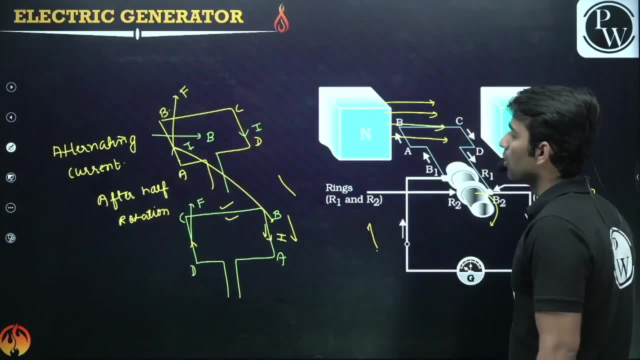 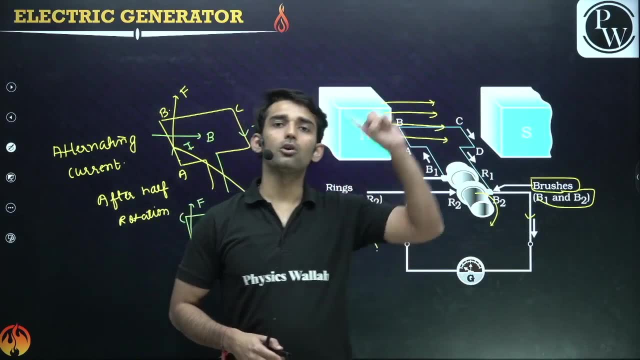 guys so this is the distribution box okay so we have electric generator we have we have read about the domestic circuit in our houses right so i had also told you about the advantages of the parallel 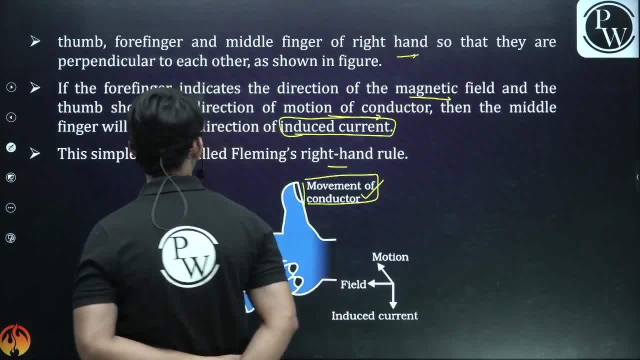 connection and the series connection okay guys we had read about the fleming's right hand rule right hand rule states that if you stretch your forefinger middle finger and the left in the 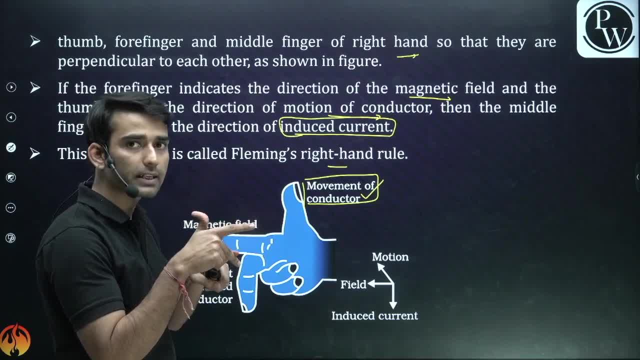 thumb thumb points in the direction of the force middle finger in the direction of the induced current and four finger points in the direction of the magnetic field guys it this question is 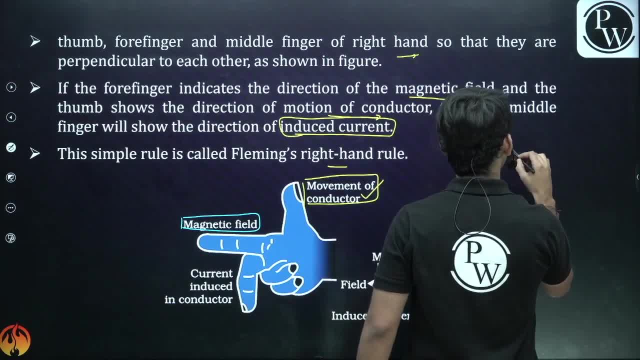 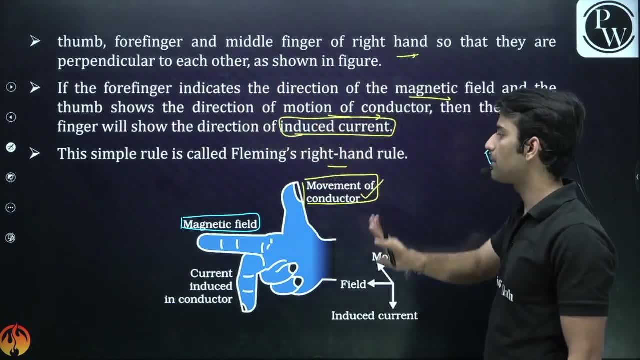 directly asked in your exam that state fleming's right hand rule it can be of two marks can be of three marks just write it as it is this language you will get complete marks and if you can draw 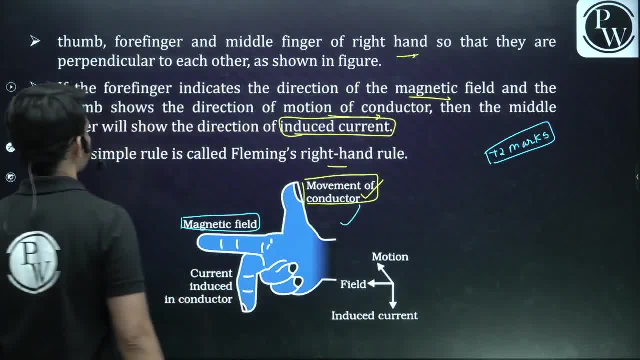 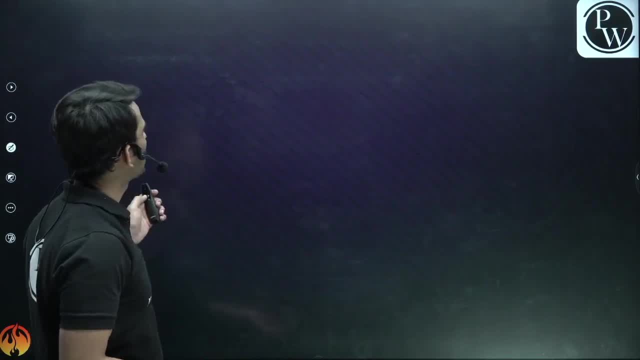 this figure it would be completely fine okay then we had read about the electromagnetic induction what is the phenomenon of electromagnetic induction we had also read about what on what 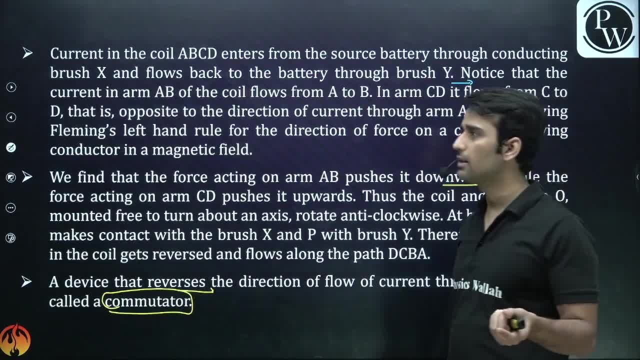 principle is the electric motor based we had also read about what principle is the electric motor based it converts mechanical energy electrical energy into mechanical energy guys right then we had read 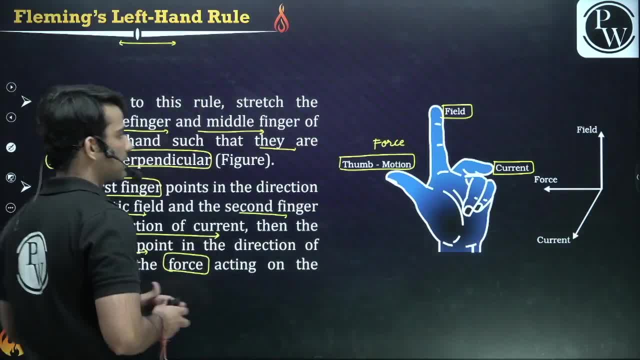 about the solenoid we had read about the fleming's left hand rule it states that if you take your left hand and stretch all that middle finger or thumb forefinger and the middle finger middle finger will point in the direction of the current forefinger in the direction of the magnetic 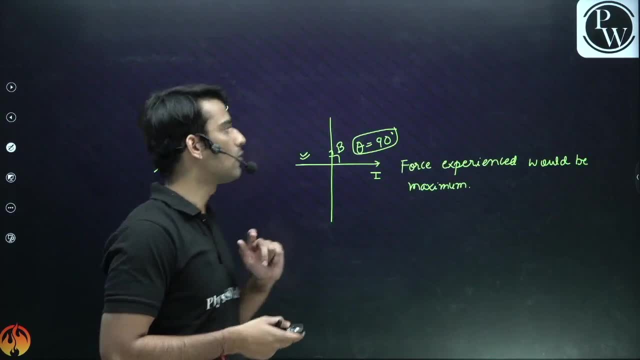 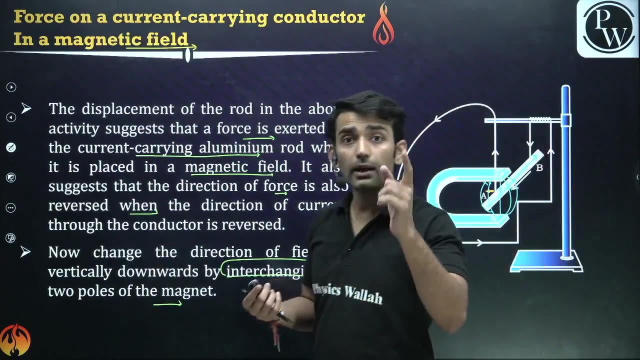 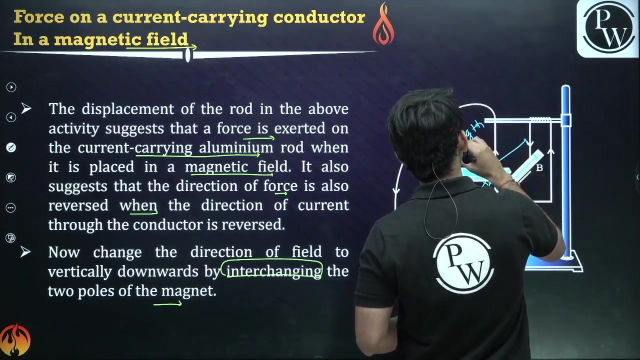 field and thumb in the direction of the force exerted okay then we had read about how does the force on a current carrying conductor depends it depends on the magnetic field it depends on the length of the conductor guys let me tell you this if you increase the length of the conductor the force exerted on the conductor would be increased we also have a formula for that but 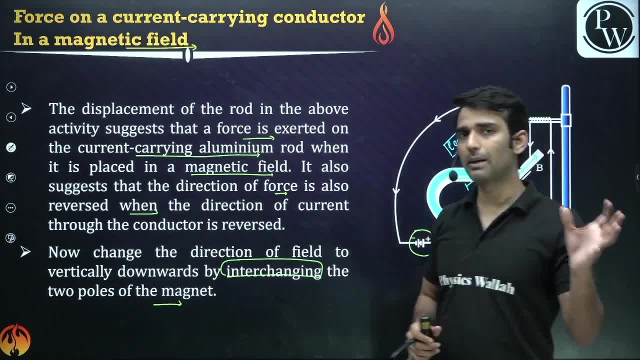 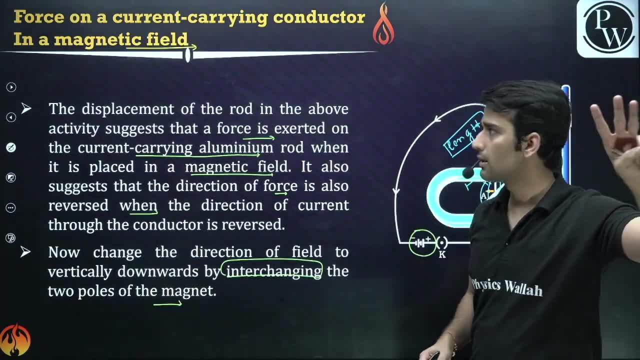 you will study that in the higher classes but right now just keep this thing in mind that it depends on the length of the conductor it depends on the current it depends on the magnetic field right if you change any of these the force would be changed okay then we had read about the 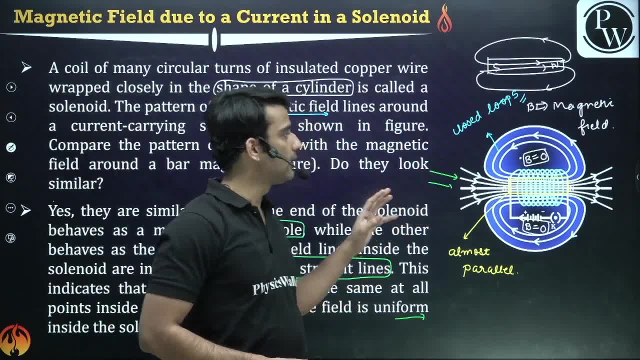 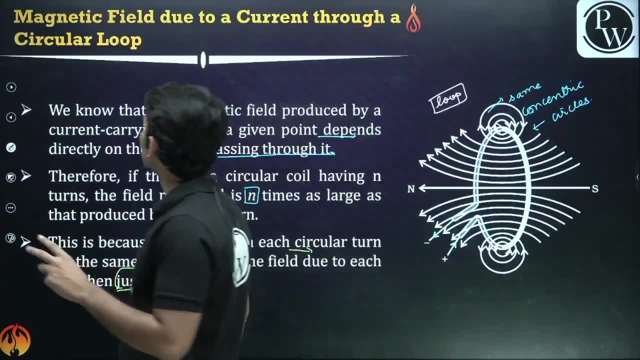 electromagnet we had read about the solenoid solenoid basically right we have a pattern of the solenoid is kind of same as that of the electromagnet right guys then we had also read about the magnetic field due to a current carrying circular loop it kinds of looks like this so guys 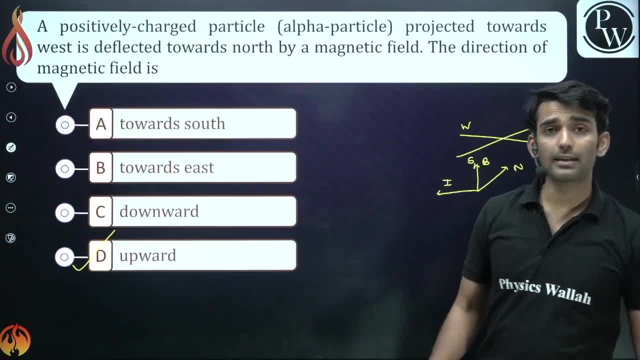 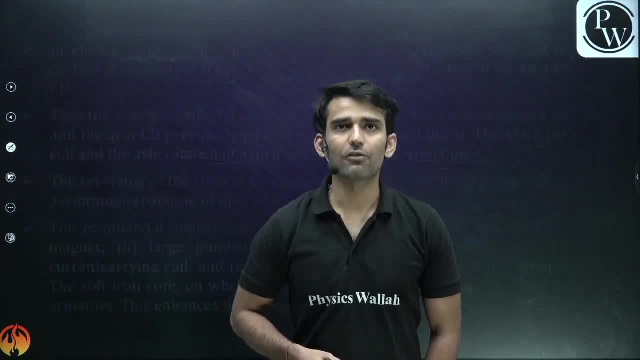 we had seen all these things in our class so i hope you guys have completely enjoyed the session we have a thorough revision of this chapter magnetic effects of electric current so you will also be getting a dha for this guys okay so just stay connected fine so this was all about the 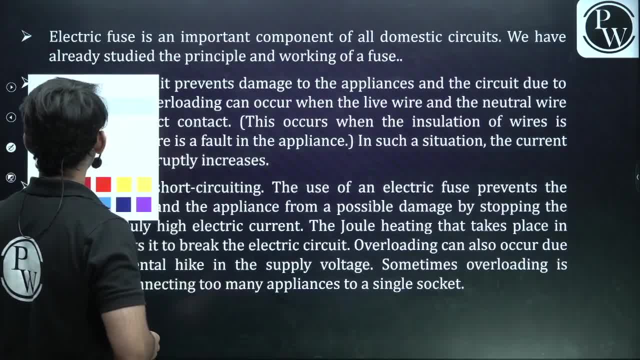 thing electric circuit thing so now the last part of the video is that we are going to talk about the electric fuse so guys the fuse basically domestic circuit why do we use fuse because it prevents 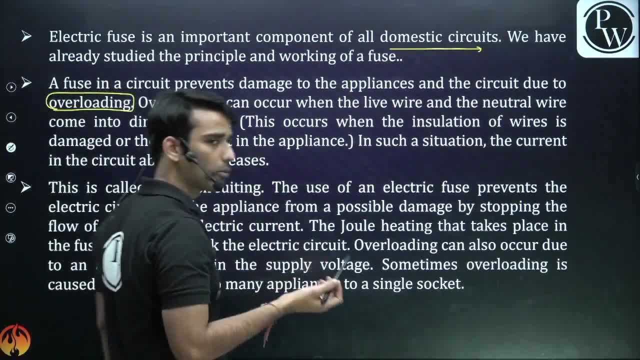 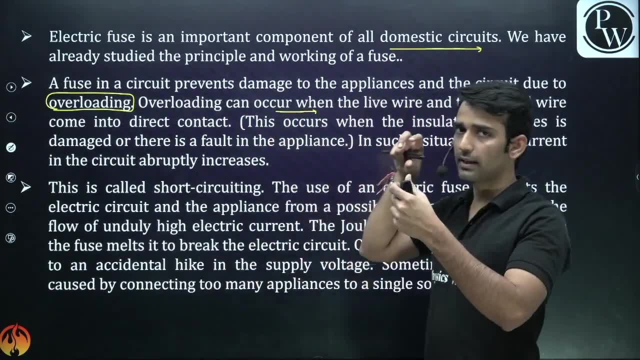 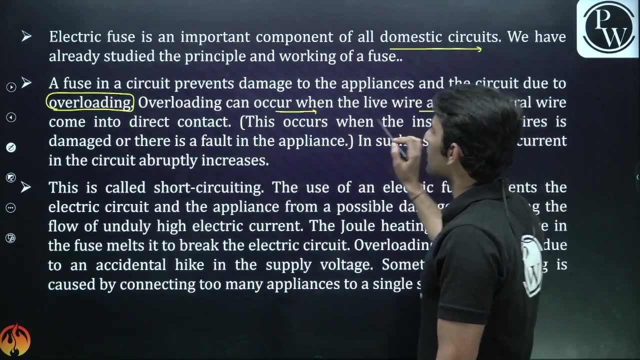 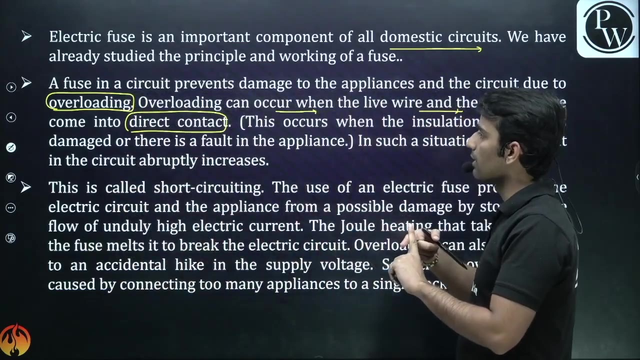 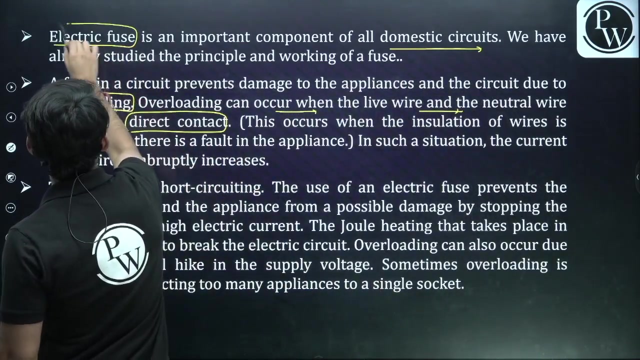 whenever there is a overloading there is excess of excessive amount of current that flows in the circuit to prevent that basically overloading can occur whenever basically uh if you connect too many sockets in a circuit overloading can occur in order to prevent that live wire and neutral wire come into direct contact the live and the neutral wire come can come into direct contact short circuiting right and we have excessive current in that case now what does the fuse do fuse basically is a safety appliance it has a wire it has a it has an alloy wire connected in between